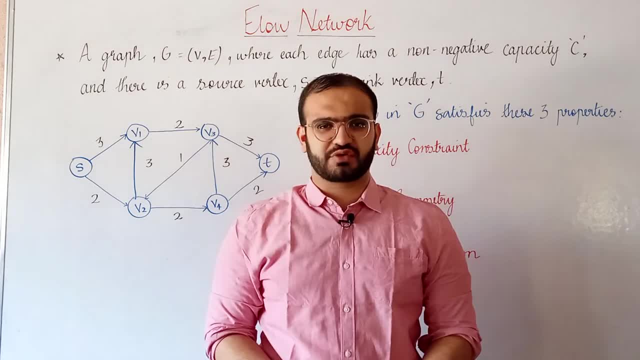 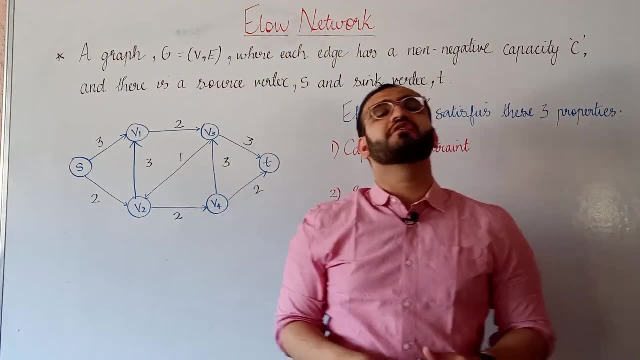 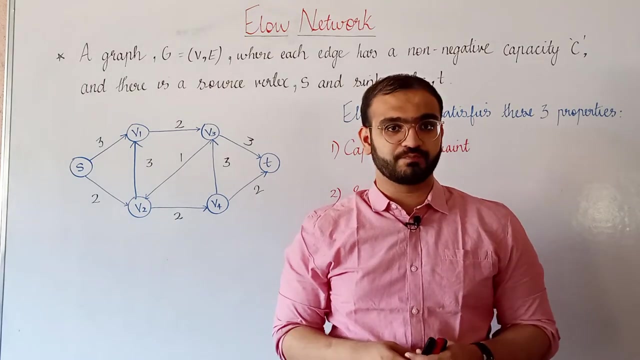 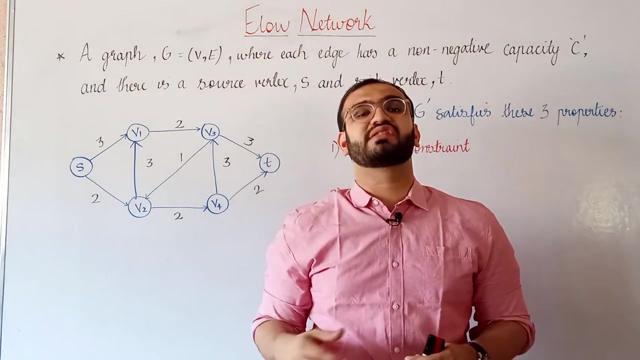 Hi guys, welcome to this video of the advanced data structures playlist where we are going to discuss flow network. So in this video we will start off with what is a flow network, then we will define the different properties of a flow and then we will look at residual capacity and residual graphs and then we will move towards the max flow problem, where we will discuss the Ford-Fulkerson algorithm. 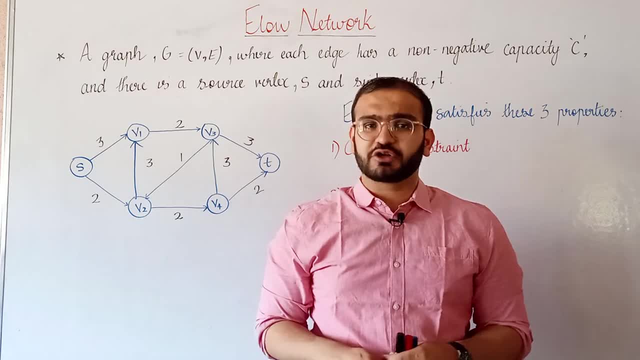 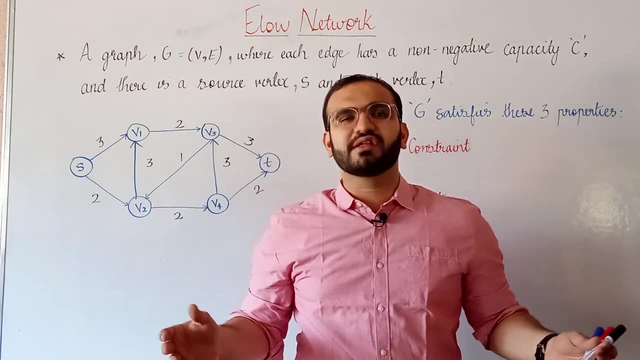 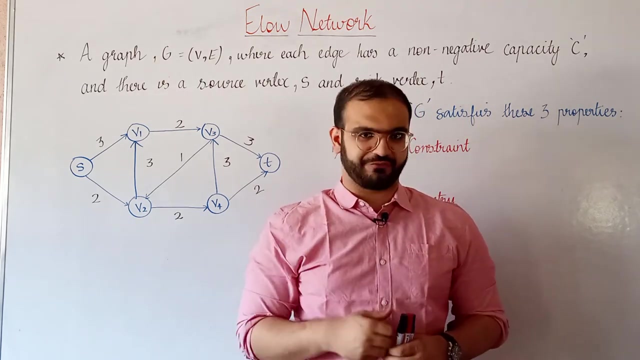 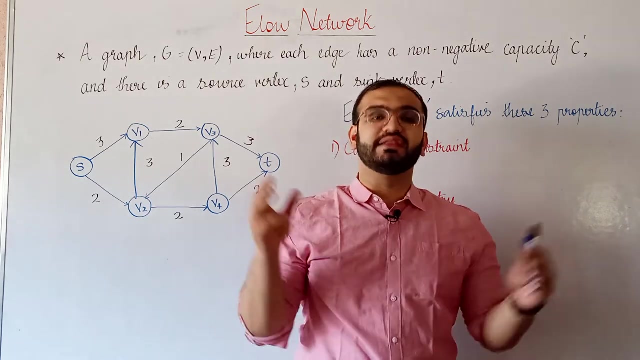 And then, finally, we are going to spend the later part of this video in solving a max flow problem using the Ford-Fulkerson algorithm. So let us start. So what is a flow network? A flow network is actually a graph in which each and every edge has a capacity, And in this graph you have got a source vertex and a sink vertex. 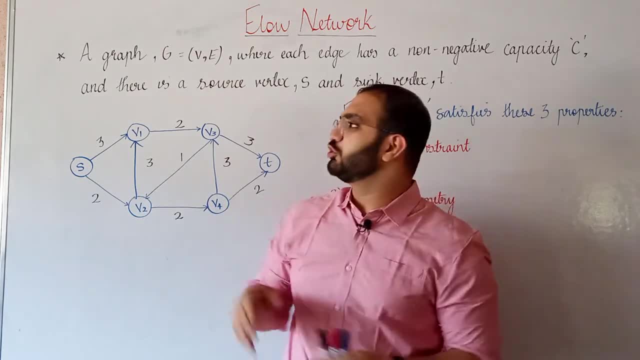 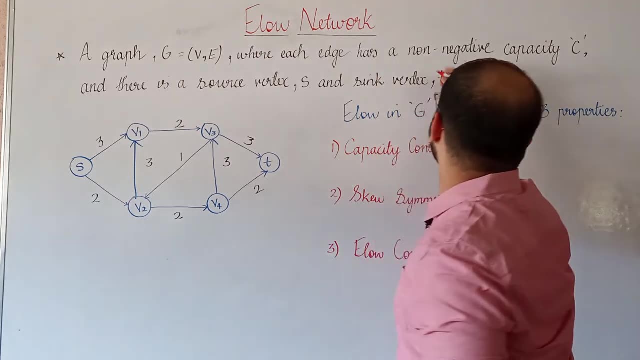 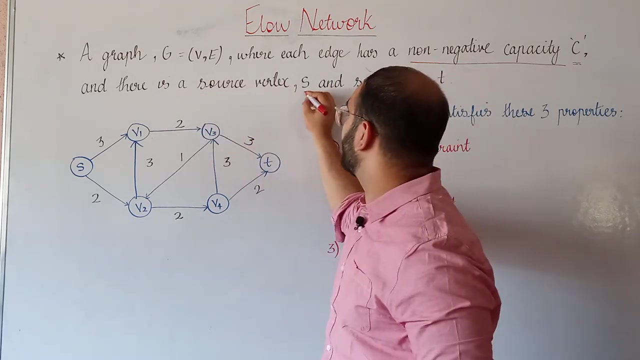 Or a source vertex and a destination vertex. So, if you look at it, a flow network is actually a graph where each edge has a non-negative capacity, C, and there is a source vertex in this graph called as S and a sink vertex called as T. 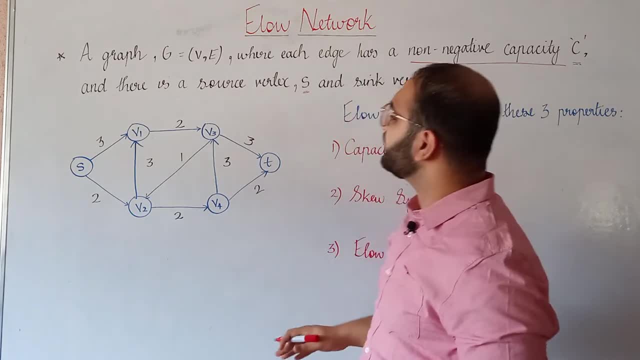 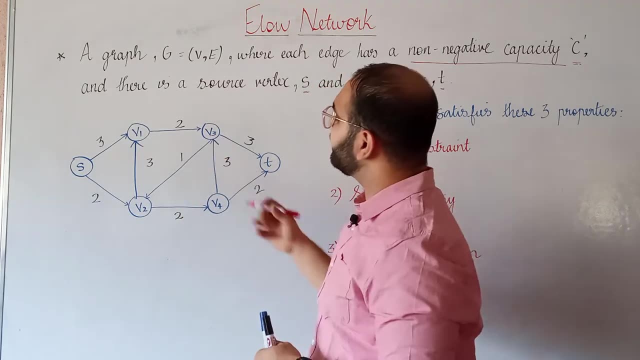 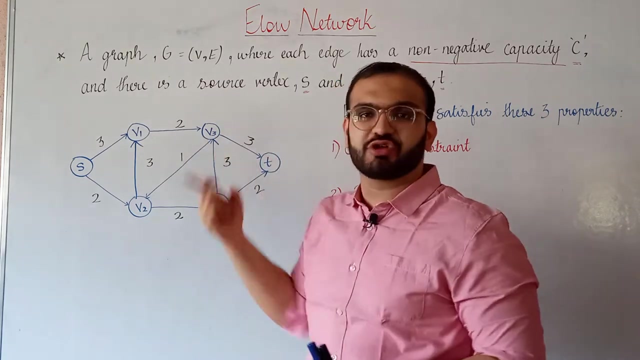 So here I have drawn a flow network. In this you can see that it looks like a graph And, of course, a graph with directed edges. You can notice over here that each and every edge has an associated capacity or an associated number, which is known as capacity. 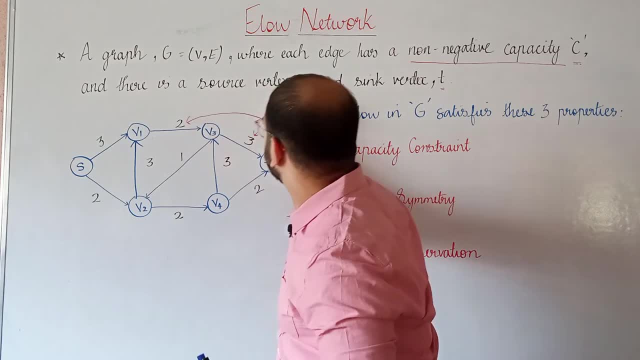 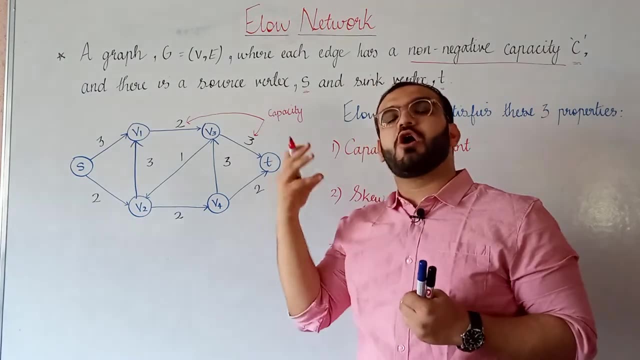 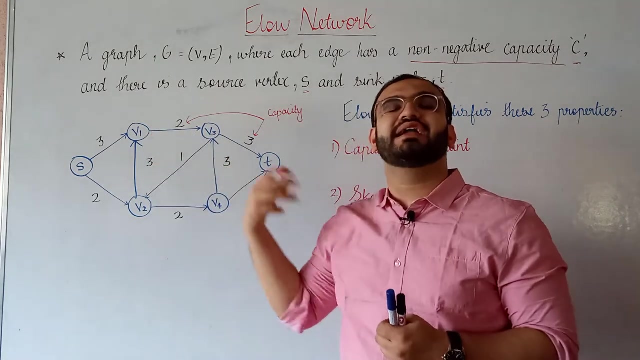 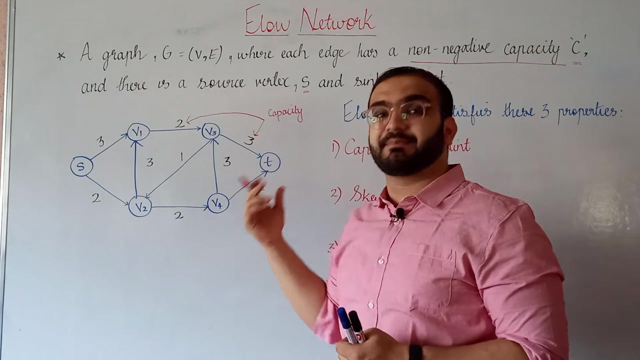 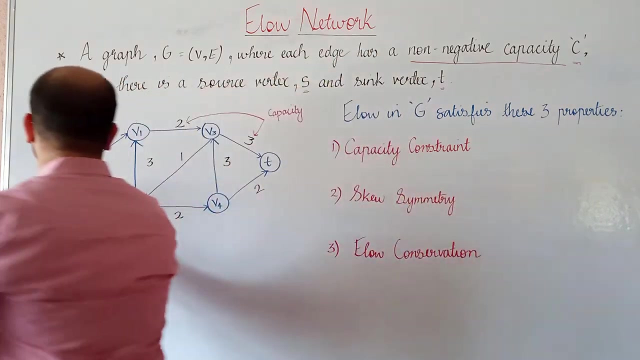 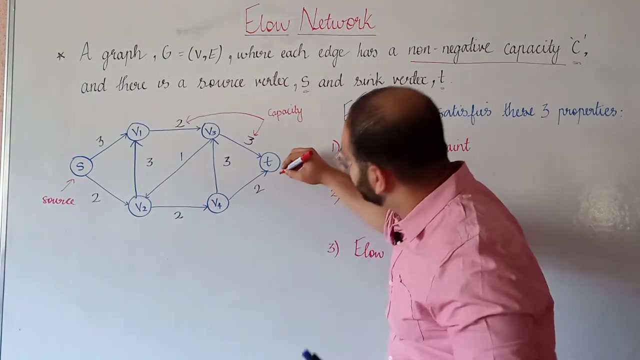 Like these are actually called as capacity of the edge right. That means the maximum amount of material, any kind of material that can flow through this edge, is known as its capacity right. So, as you can see over here, each and every edge has an associated capacity C, and apart from that, in this graph you can see that we have got a source denoted as S and a sink denoted as T. 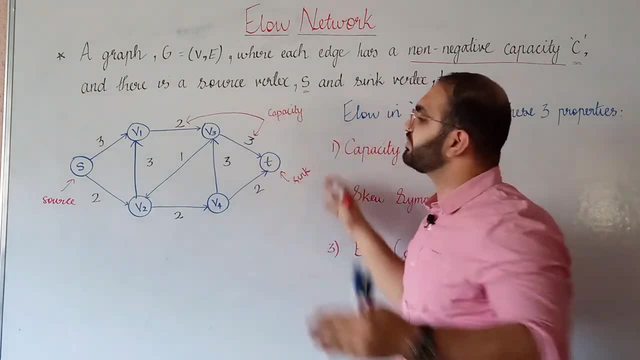 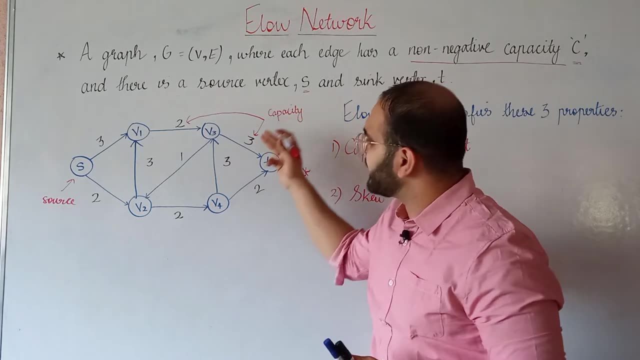 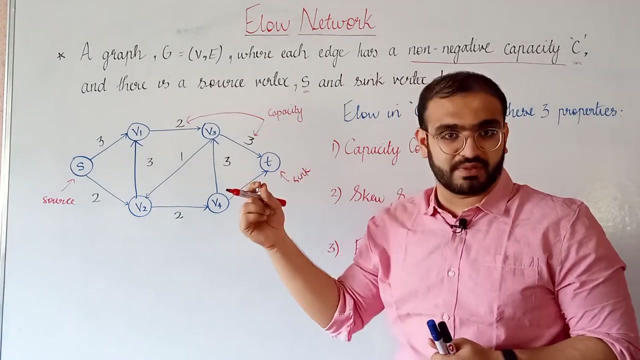 So we have got these two vertices, So this is basically a flow network. Now, apart from this one number, that is capacity, which is associated to each and every edge in this flow network, there is another number that is associated to each and every edge. 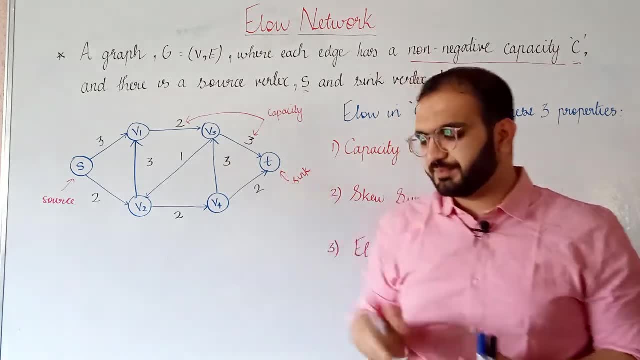 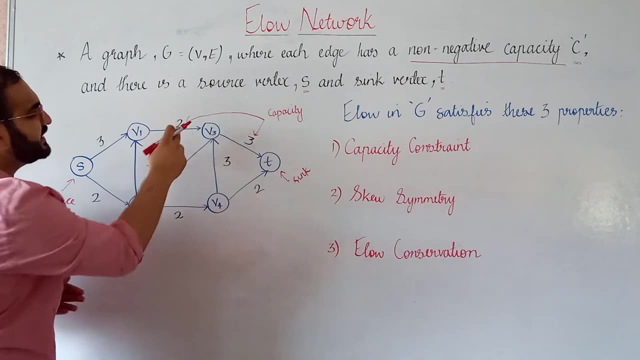 And that number is known as the flow. So basically, when we say that from V1 to V3, the capacity is 2.. That means that the maximum amount of material is C, So the amount of material that can pass from V1 to V3 is 2, or the capacity of this road is actually 2.. 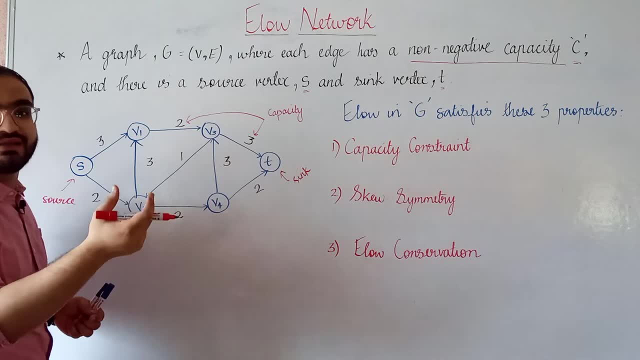 But what is the actual amount of material that is flowing through this path, through this edge, So that quantity is denoted using another number that is known as flow? okay, I will randomly write down the flow over here. I will use this red color. 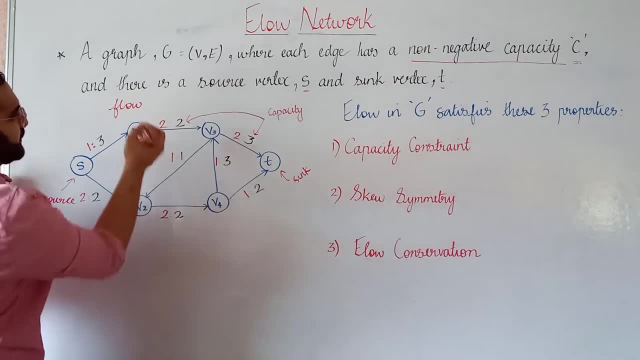 The red. I have written down the flow for each and every edge, right? So these- this 2 over here and this 1 over here- is the flow for these particular edges, right? So basically, flow determines the actual amount of material flowing through a particular edge. 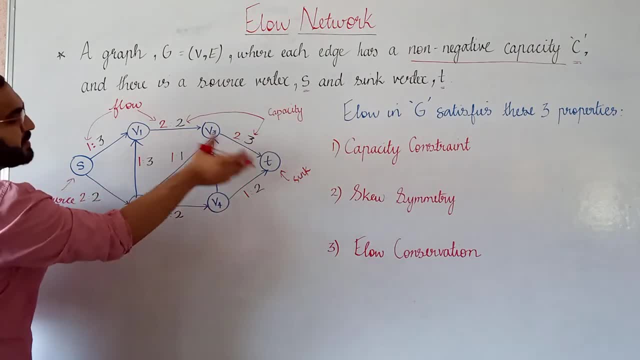 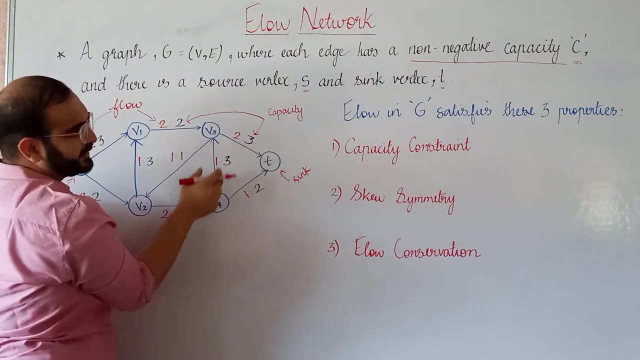 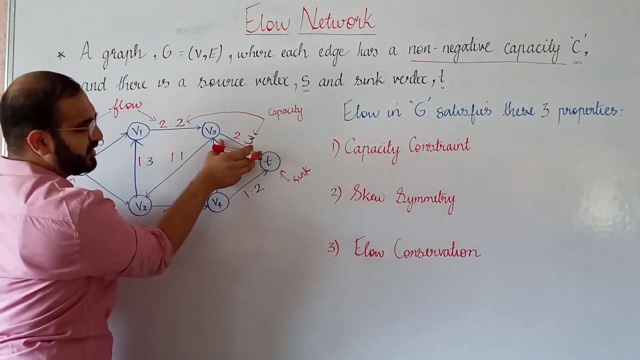 Whereas capacity determines the maximum amount of material that can flow through an edge. For an example, over here, from V3 to T, in this edge the capacity is 3.. That means the maximum amount of material that can flow through this edge is 3.. 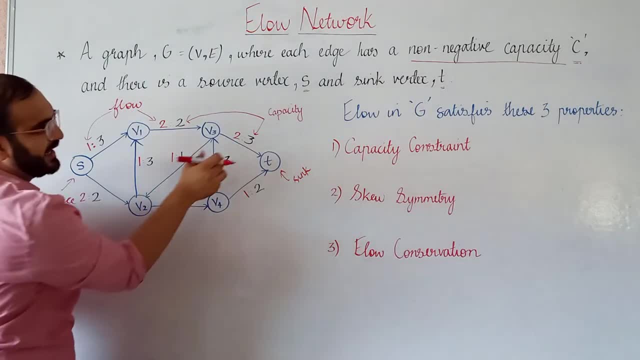 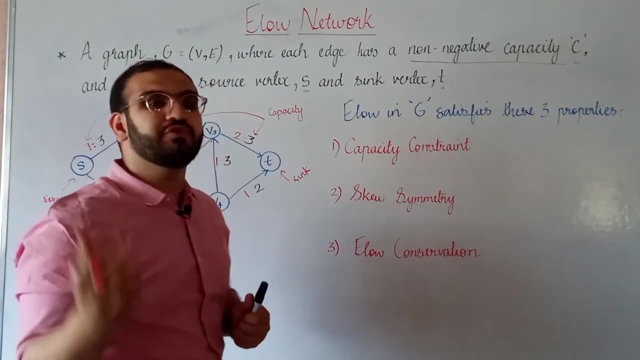 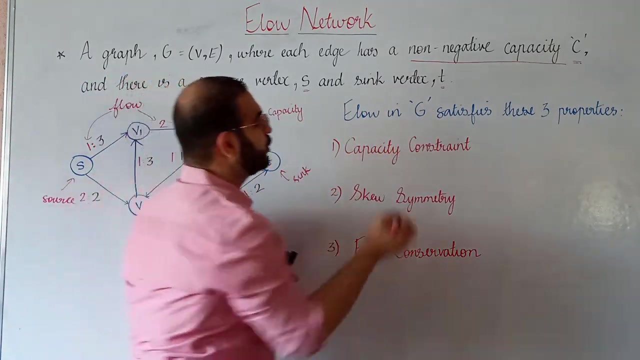 Whereas its flow value is 2.. So that means the actual amount of material flowing through this edge right now is 2, right. So now, in order to better understand flow through a network, let us look at some properties that flows in any flow network, such as funds. 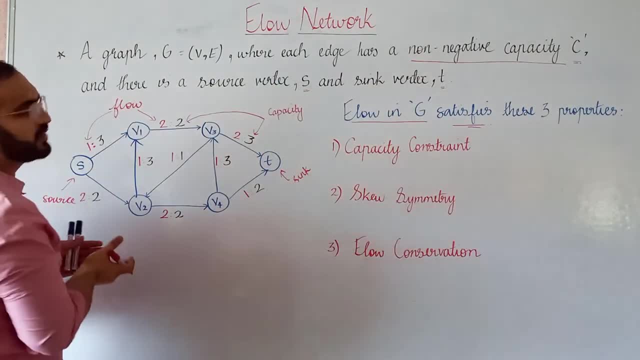 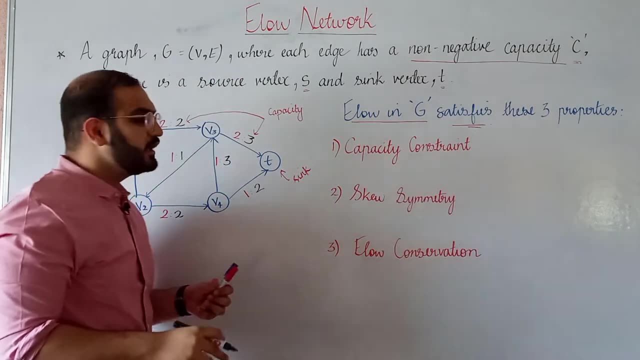 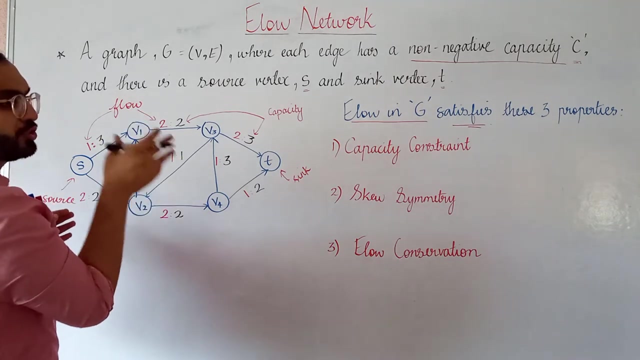 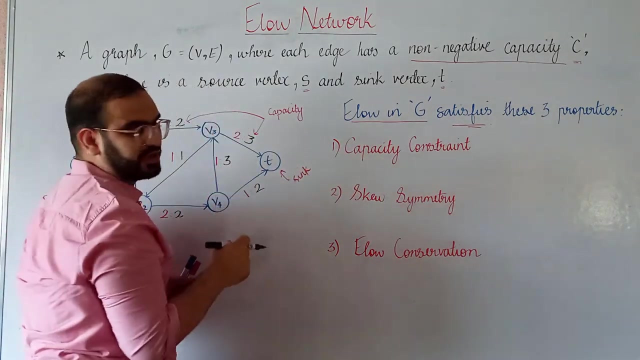 So let us look at these 3 properties That a flow in any particular flow network satisfies. So the first property is actually capacity constraint, right. That implies that for any particular edge in the flow network, the flow through it should always be less than or equal to the capacity of that edge. 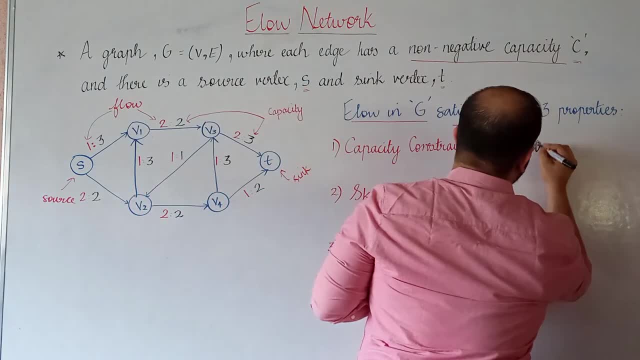 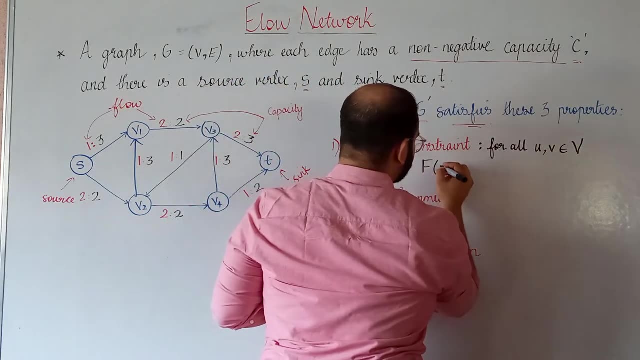 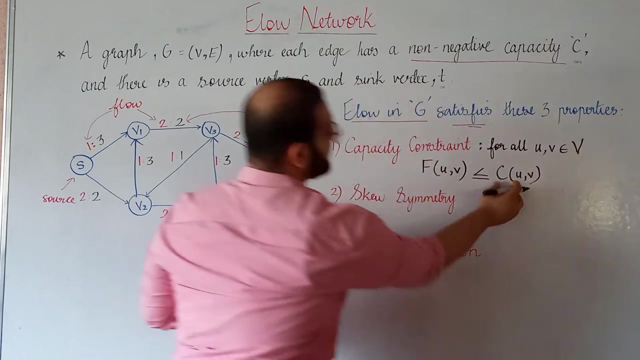 If I write it down, I can write it in this way: For any particular edge in our network, the flow through that edge should always be less than or equal to the capacity of that edge. So C denotes the capacity, whereas F denotes the flow of that edge. 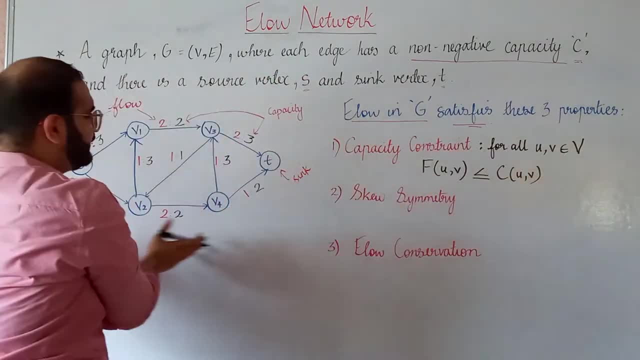 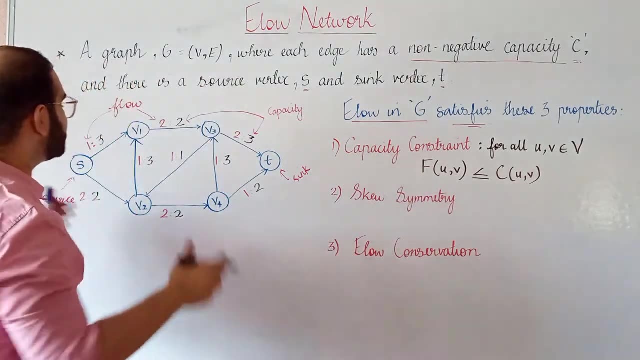 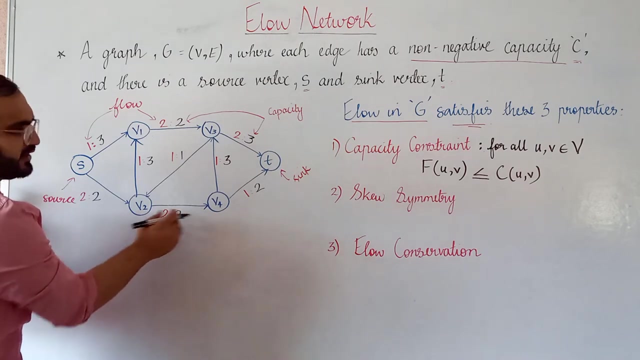 So for all the edges in our flow network, this capacity constraint is a property that needs to be followed. So even here you can see that here the capacity is 2. And the flow is actually equal to the capacity that is, 2. Whereas over here the capacity is 3.. 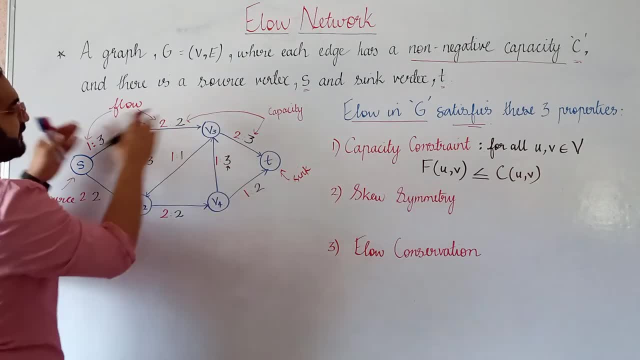 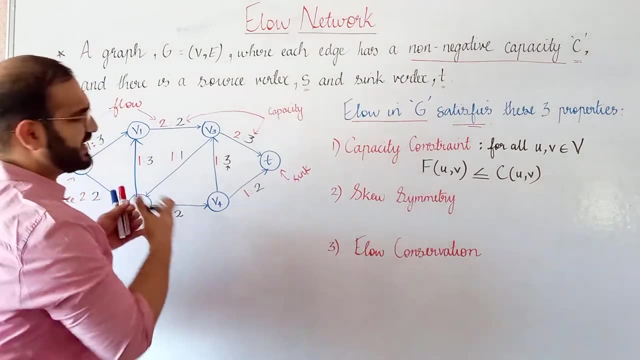 Whereas the flow is less than the capacity. Nowhere over here you will find out that the flow is actually greater than the capacity. Even in the real case scenario, you will understand that it is not possible for the flow to be greater than the capacity, right? 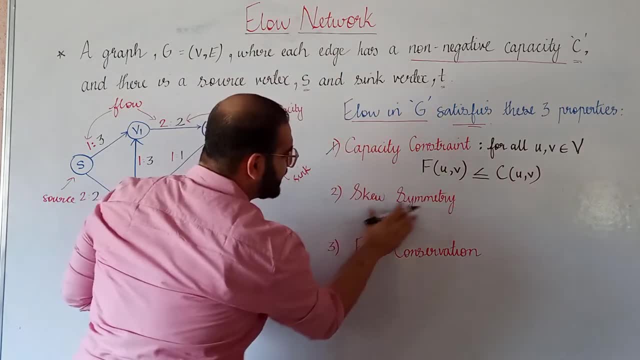 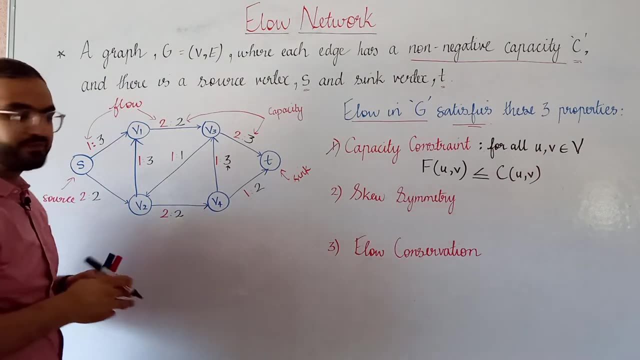 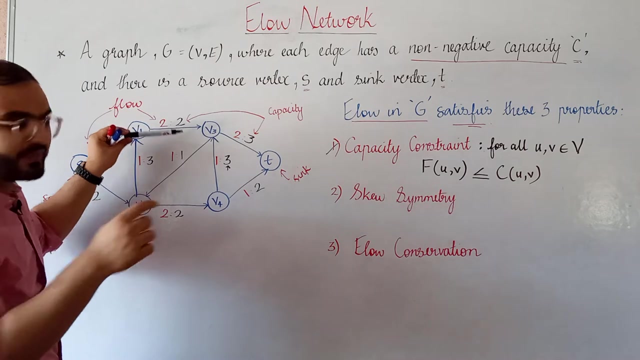 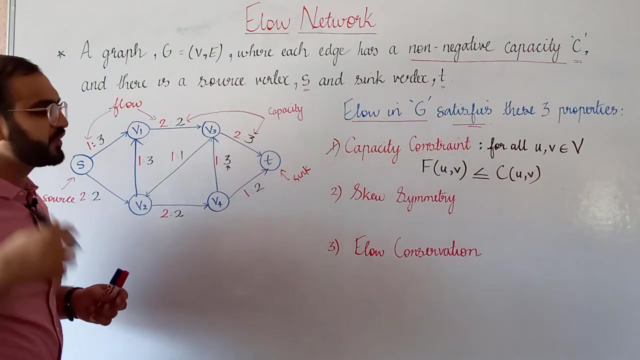 So this was the capacity constraint. Now talking about skew symmetry. So basically, skew symmetry says that for each and every edge, if there is a path flowing in this direction with a particular flow, there will be another path in the opposite direction with a negative flow. 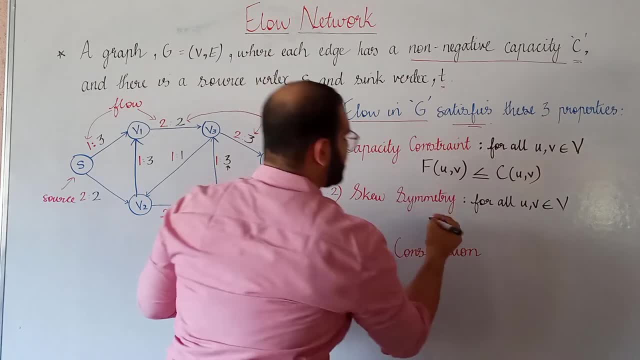 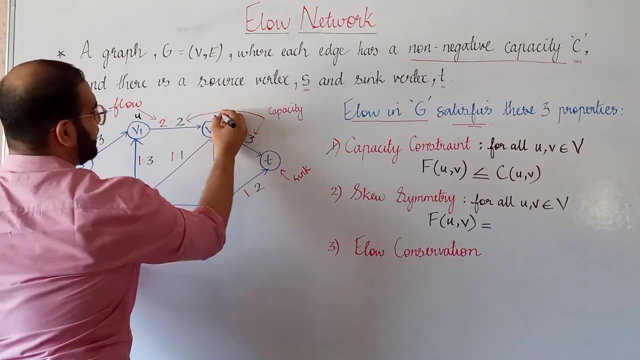 So if I write it down, that implies for all the edges: if there is a flow from the vertex U, let us call this as vertex U and this as vertex V. So if there is a flow from U to V, then there will be another flow in the opposite direction. 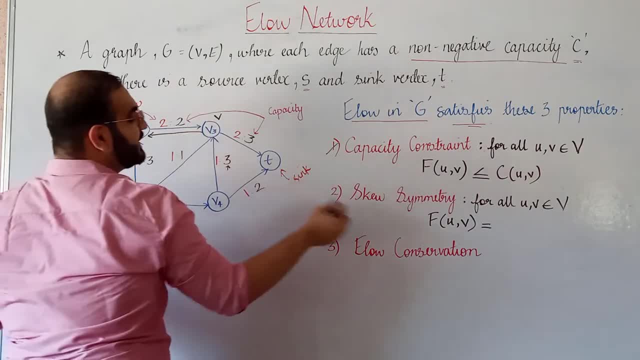 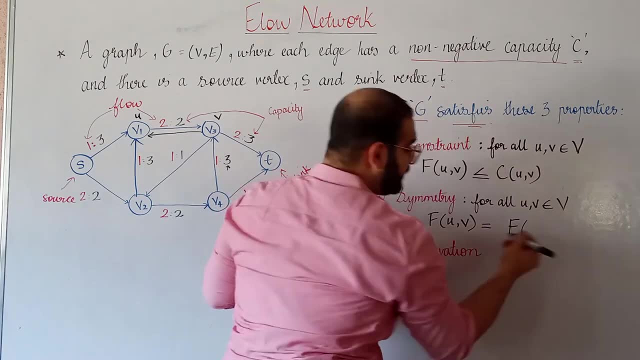 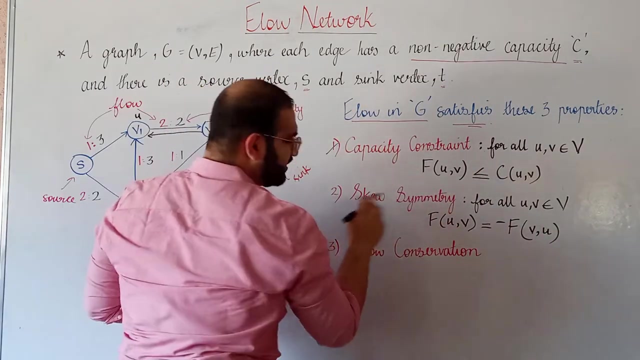 in this opposite direction, which will be negative of that flow from U to V And that flow because it is in the opposite direction, so we will write it as F and it will be a negative flow, Right? So this is the skew symmetry property that is satisfied by any flow in a flow network. 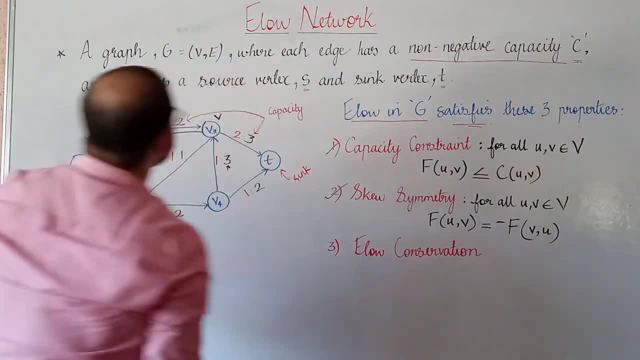 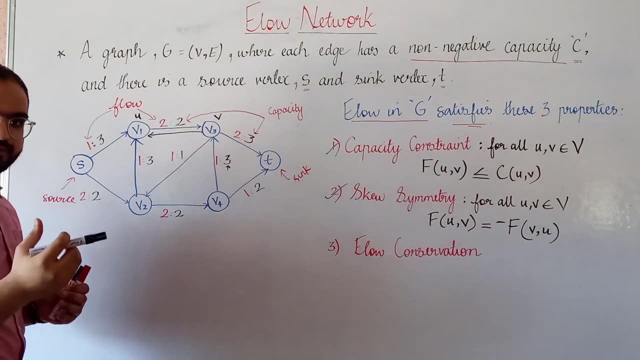 Talking about flow conservation. Now, to understand flow conservation, what you need to understand is that at any particular vertex in our flow network, the flow will not be accumulated, or the material that is passing through the entire flow network is not going to be accumulated at any particular vertex. 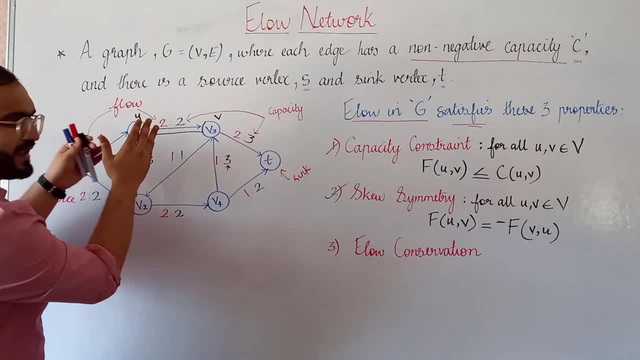 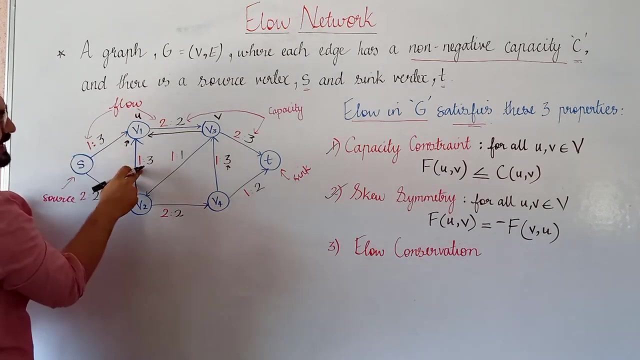 That implies that whatever is going into any vertex will also be coming out of that vertex Right. So, for example, if we look at this V1, in this V1, there are two flows going into it. One is of value 1 and another one is of value 1.. 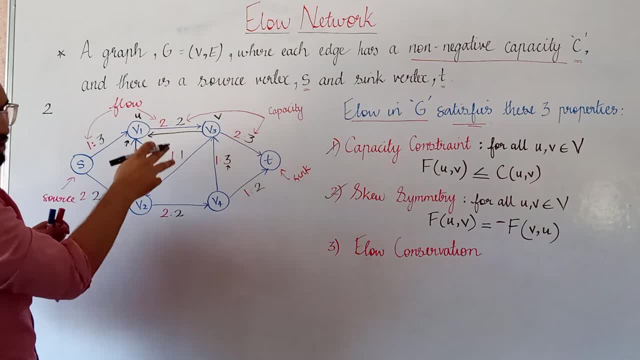 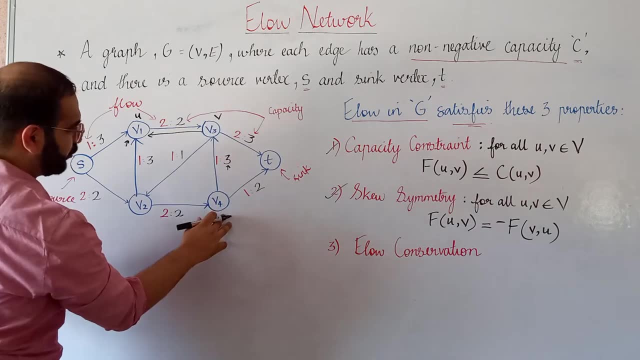 So the total flow that is going into V1 is 2.. And, as you can see, the total flow coming out of V1 is 2. Right Over here also, if you look at V4.. So at V4, the total flow that is going into it is 2.. 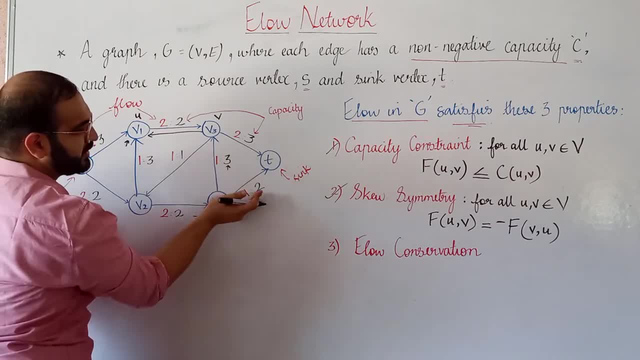 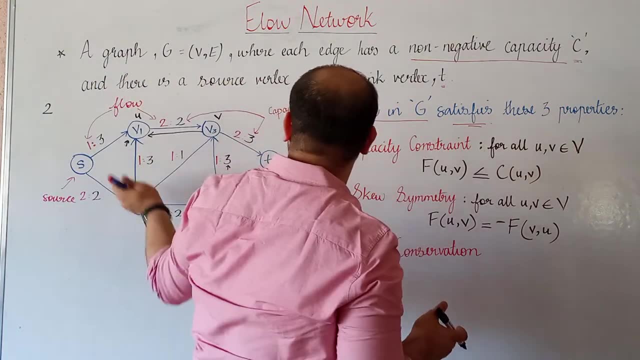 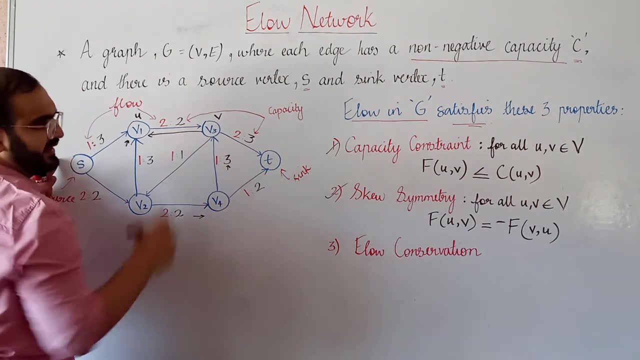 Whereas the total flow coming out of it is 1 plus 1, 2.. Right, So this flow conservation property has to be satisfied at each and every vertex in a flow network, Except at the source and at the center, Because, as you can see over here, 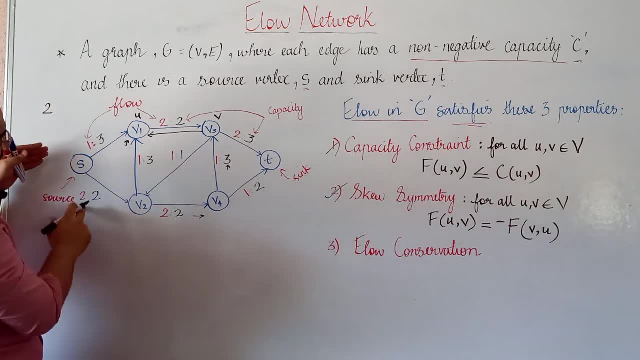 actually the flow coming out of source is total 1 plus 2, 3.. But there is no flow going into the source. That is why it is known as the source Right, A vertex that has no incoming flows Right, Even in this case, sink. 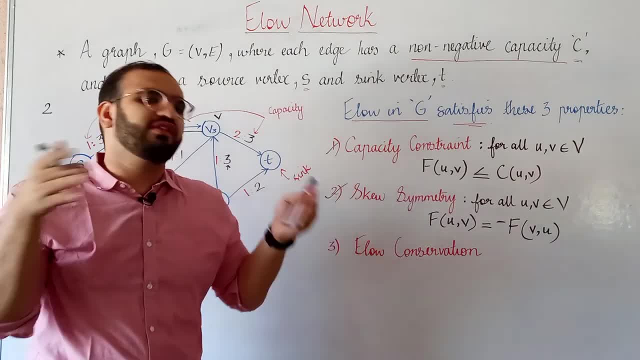 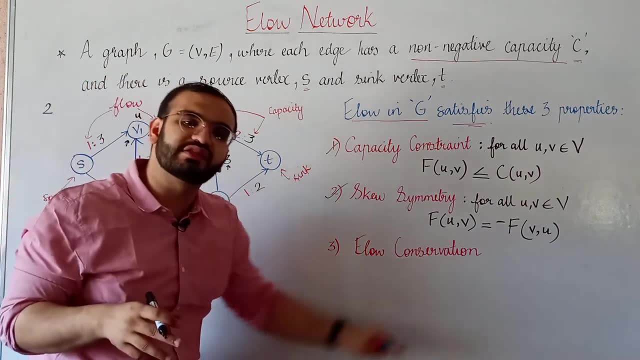 you will find that there are no outgoing flows. That is why it is known as the sink. But over here, at the source and the sink, you will find that this property of flow conservation does not hold. Rather, it holds for each and every vertex, except these two. 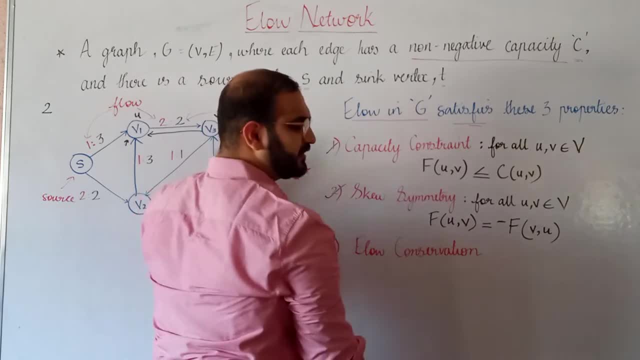 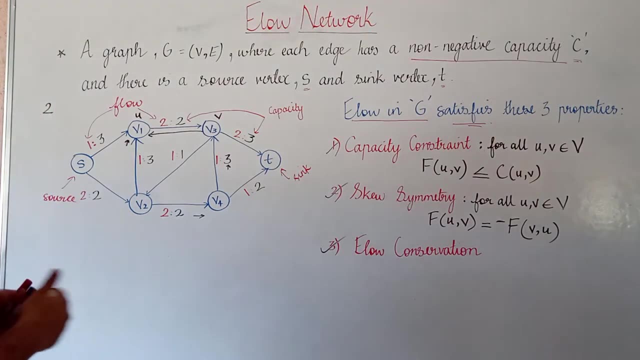 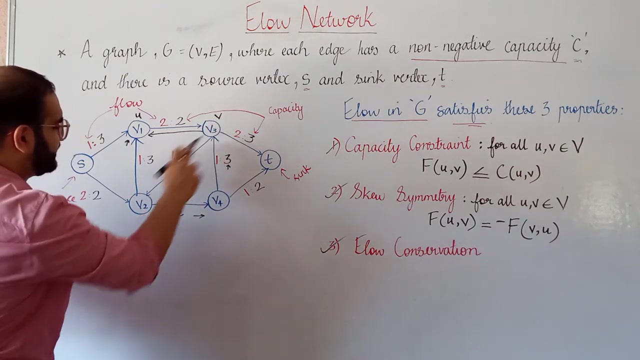 Right, So this flow conservation property holds for every vertex except the source and the sink. Another thing that you should know in case of flow network is that, if you see over here, there is a cycle Right From V2 to V4 and V4 to V3 and then back to V2.. 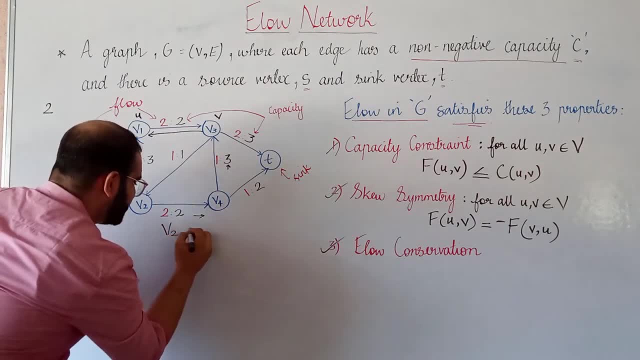 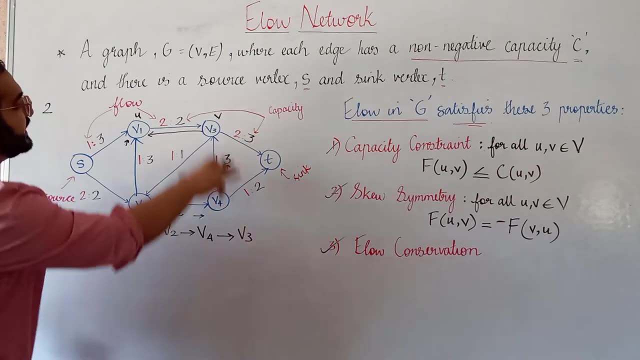 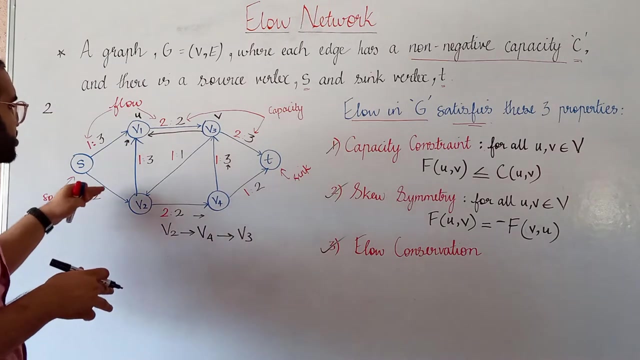 So V2, V4. So you see one cycle over here: V2, V4, V3.. Right, So this is a cycle. So basically, some material is flowing into this cycle. So even if you subtract an equal amount from each and every edge, 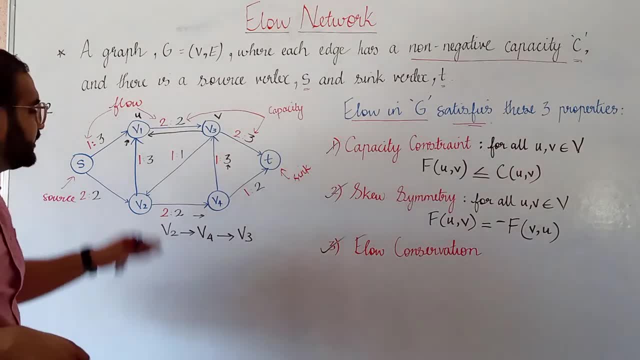 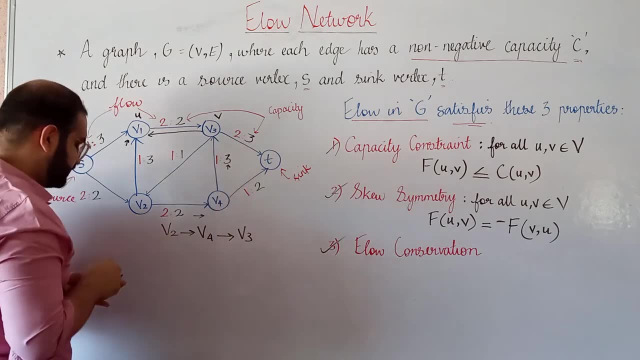 it will not make any difference And all these properties will still hold if you subtract an equal amount of flow from each and every edge in this cycle. So suppose, if I want to subtract, so right now. as you can see if you look at this V2,. 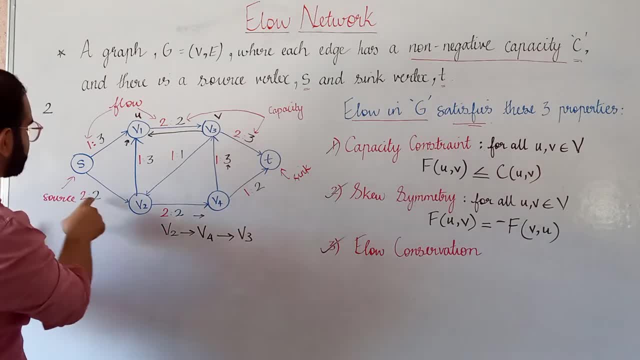 the flow conservation is followed Right, Because 2 is coming into it and 1 is also coming into it, Whereas 1 is going out over here 2 is going out. So basically, 3 is coming in to V2 and 3 is going out of V2.. 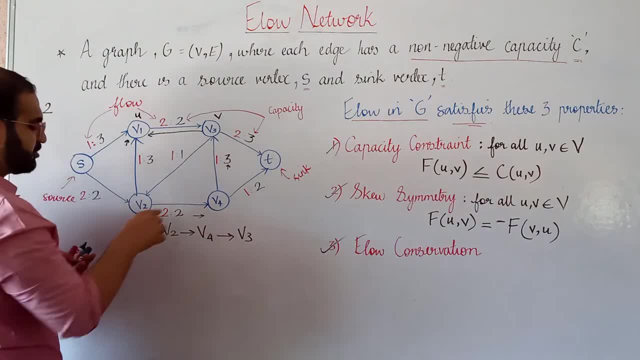 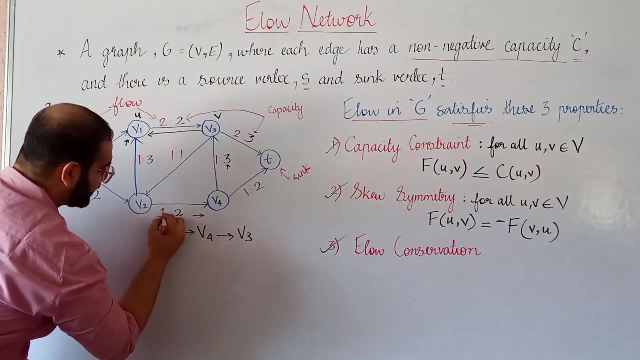 So suppose, if we subtract an equal amount, so if I subtract 1 from each of these, so this will, the flow of this will change from 2 to 1.. Right, And the flow of this will change from 1 to 0.. 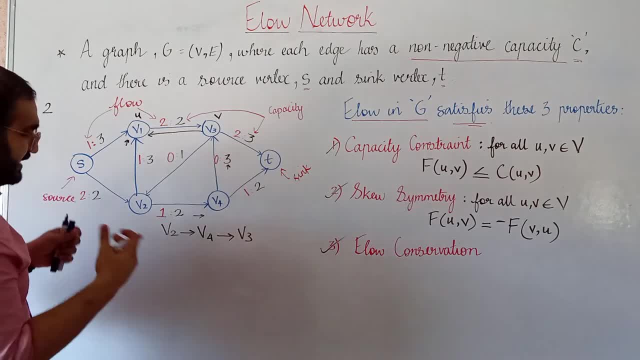 Flow of this also will change from 1 to 0. Now, if I again check, is the flow conservation property still holding right now. So again, if I look at V2, the flow going into V2 is 2 plus 0.. 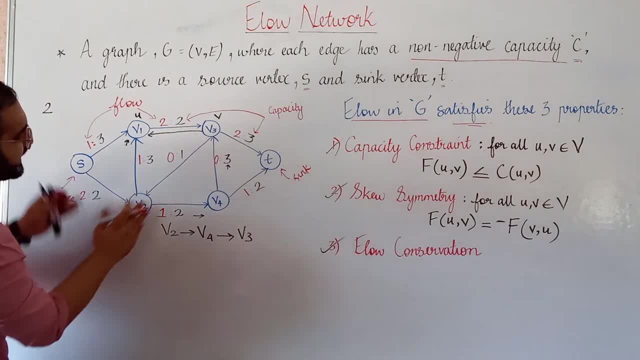 So it is total 2.. And the flow going out of V2 is actually 1 plus 1, 2.. So 2 is coming into V2 and 2 is going out of V2.. So flow conservation still holds. So, after understanding what is a flow network, 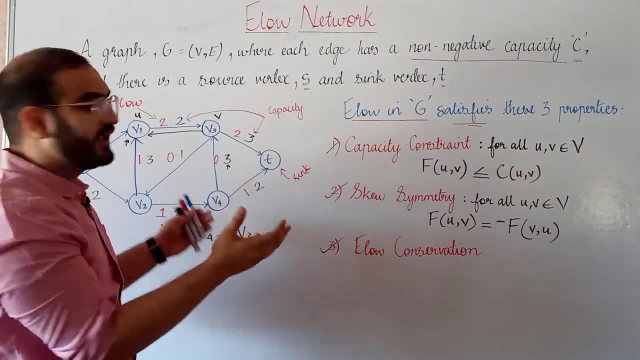 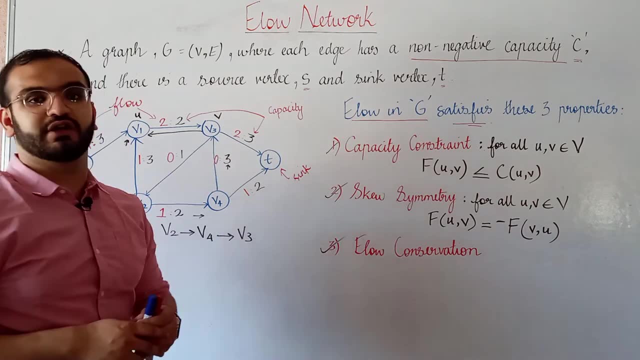 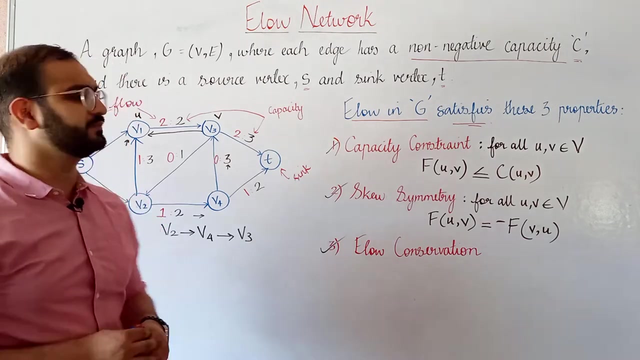 and the different properties that a flow in a flow network holds. let us now move to the max flow problem in a flow network. Let us now move. let us now understand a max flow problem in a flow network. So what is the aim of the max flow problem? 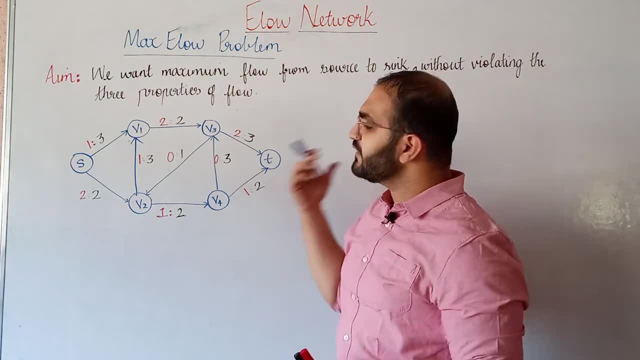 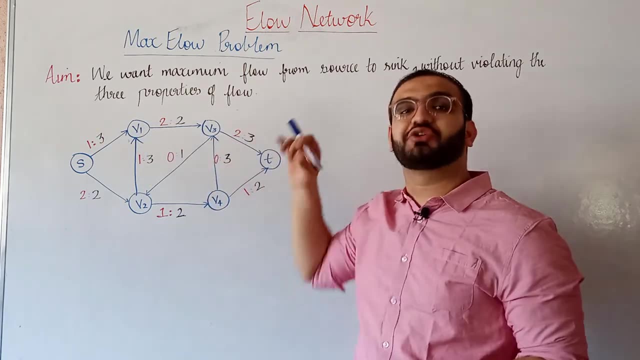 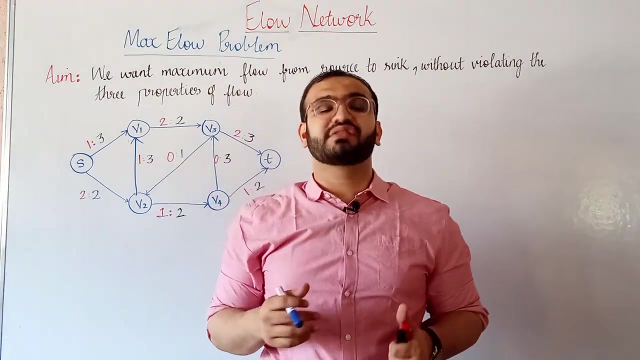 So in the max flow problem, we want maximum flow to be pulled out of the source and be pushed into the sink without violating the three properties of flow that we saw just now, That is, namely capacity constraints, skew symmetry and flow conservation. So we want these properties. 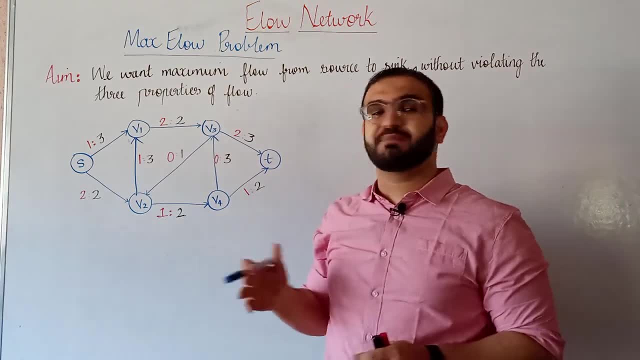 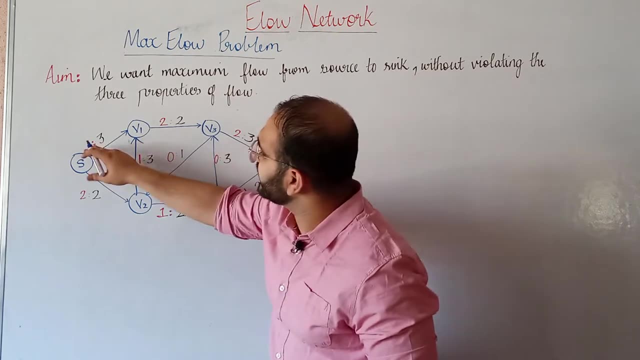 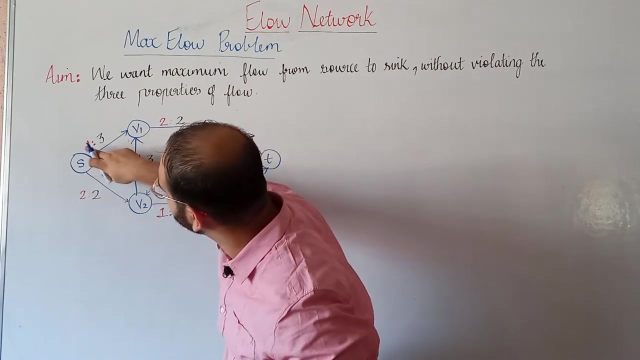 to be followed at the same time that we pass maximum flow into this flow network. So, currently, what is the flow that is flowing out of the source and going into the sink? So, as you can see, the flow coming out of the source is 2 plus 1, right. 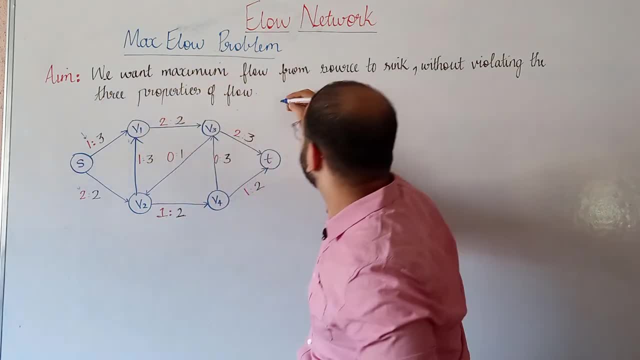 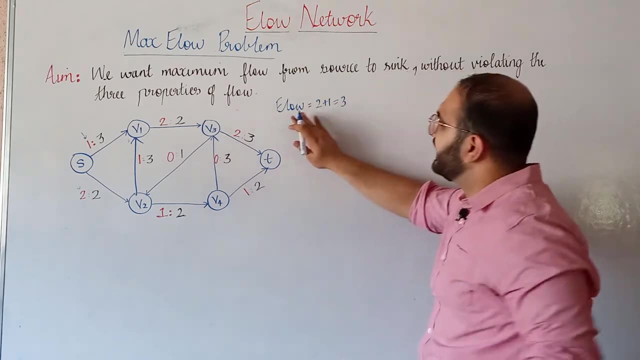 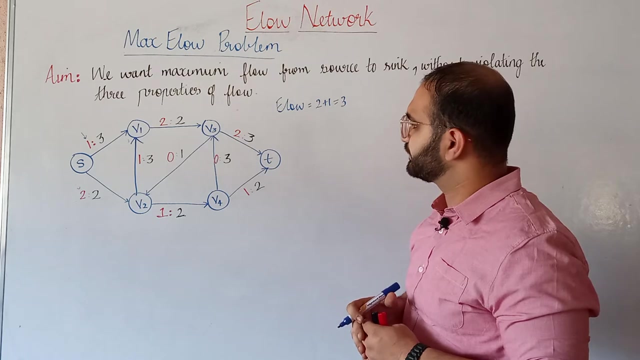 Is 2 plus 1, right, So currently the flow is 2 plus 1, 3.. Okay, So the question is: is this the maximum flow Or there is some slope to increase the flow in this flow network, So sometimes it might happen. 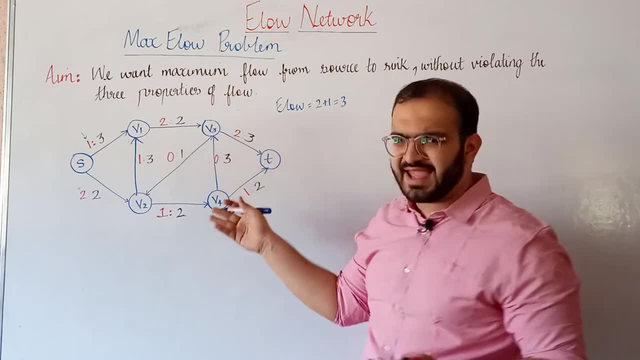 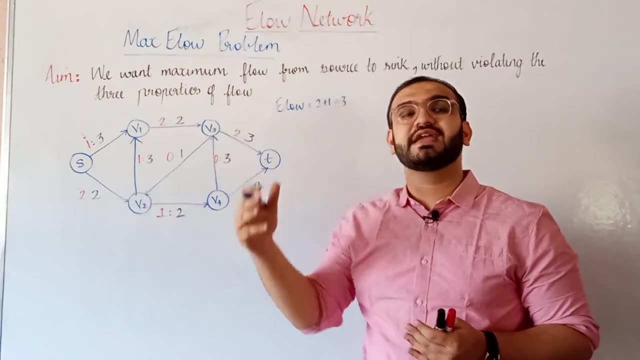 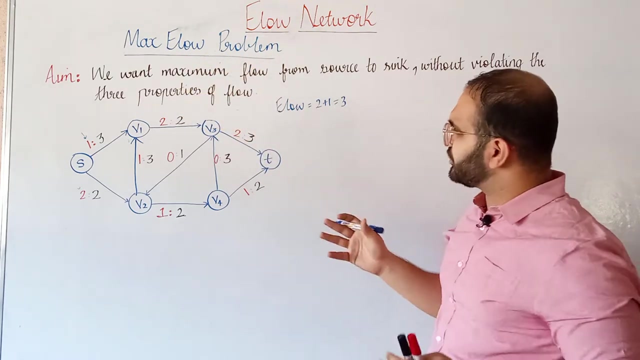 that when you decrease the flow at any particular edge, at any one or two edges, your overall flow might increase and it might take you more closer to the maximum flow that you want to achieve in this max flow problem. So is there any edge in this particular flow? 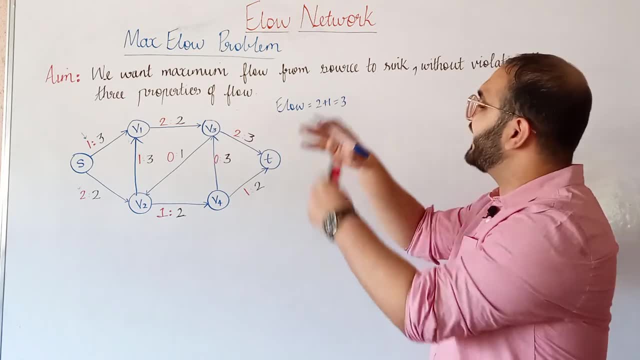 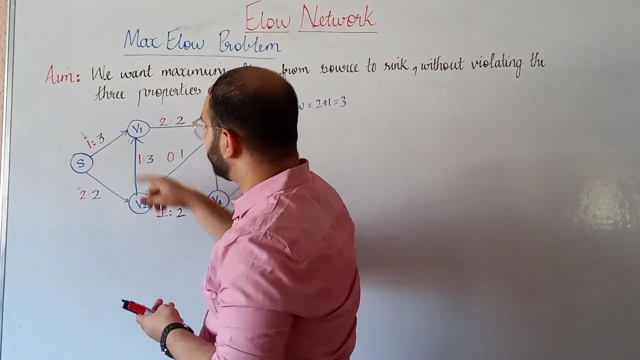 network where we can decrease its flow and increase the overall flow. So suppose, if I decrease the flow at this edge- V2 to V1, I decrease it from 1 to 0,. okay Now, because I have decreased one outgoing flow from V2,. 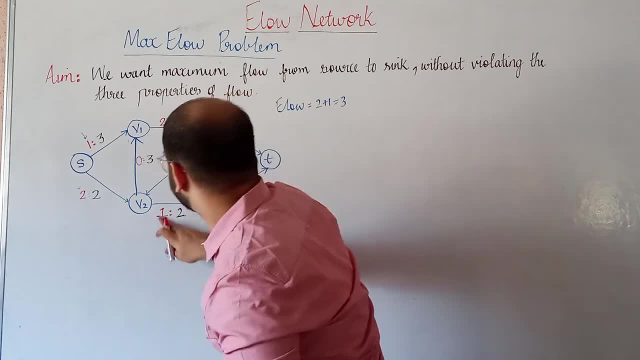 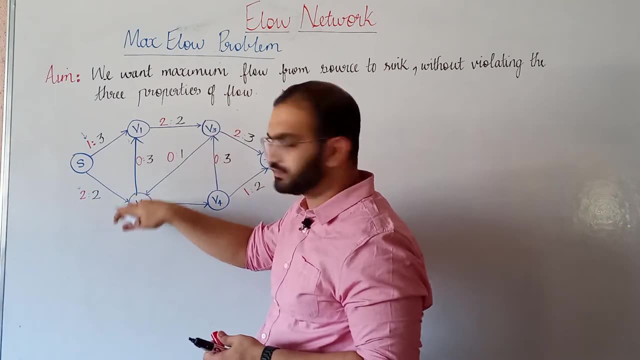 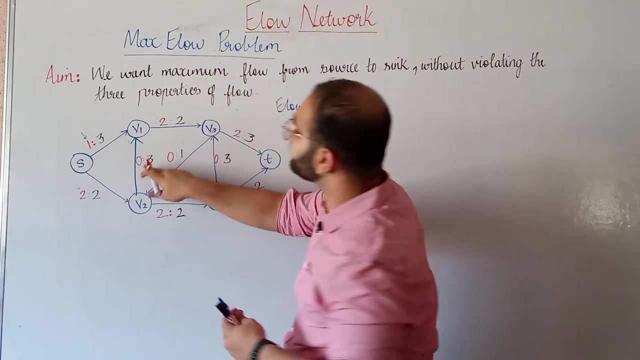 so I have to increase the other outgoing flow. So this will increase from 1 to 2, right, In order to maintain the flow conservation at V2.. Okay, And again, this will also increase from 1 to 2.. So basically, we just decreased. 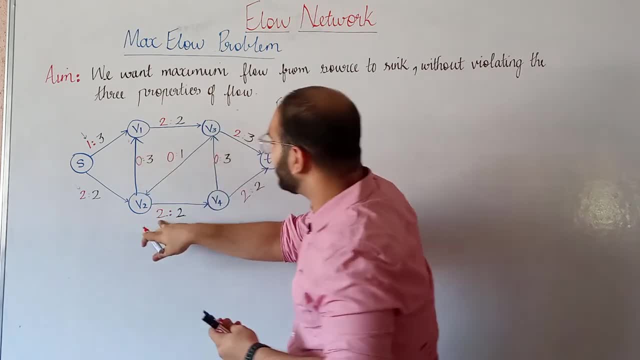 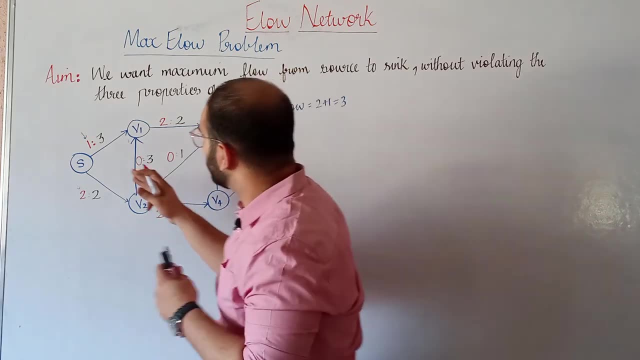 the flow at a particular edge and that has led to increasing flows over here, But still are we maintaining flow conservation at each and every edge? So if you look at this V1, the incoming flows at V1 is equal to 1 plus 0.. 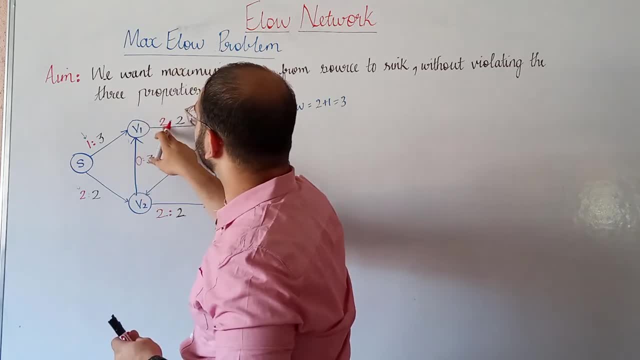 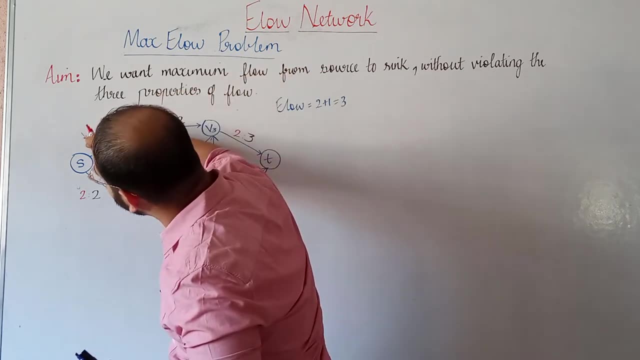 1. But the outgoing flow is actually equal to 2.. So this is not maintaining the flow conservation problem. It is maintaining the flow conservation property. So what we can do over here is that we can actually increase this flow. So even if we increase it, 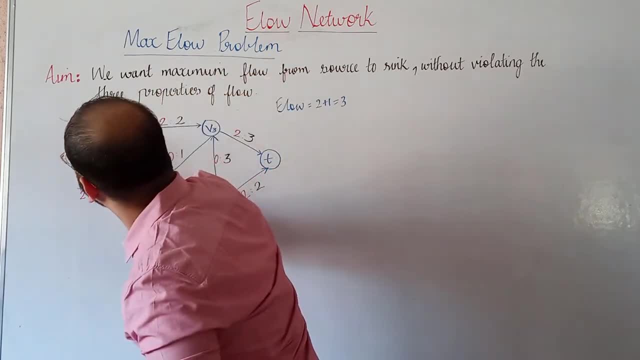 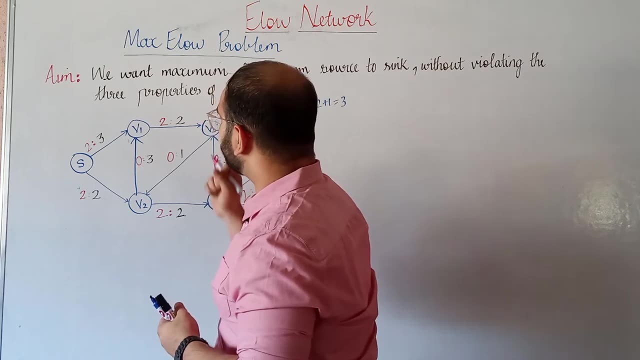 from 1 to 2, it is lesser than the capacity 3 of this edge S2, V1.. Right, So now, if you look at this flow network, you will see that the flow that is coming out of the flows and going into the sink. 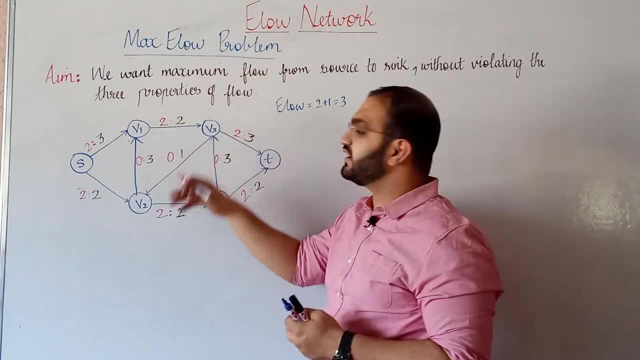 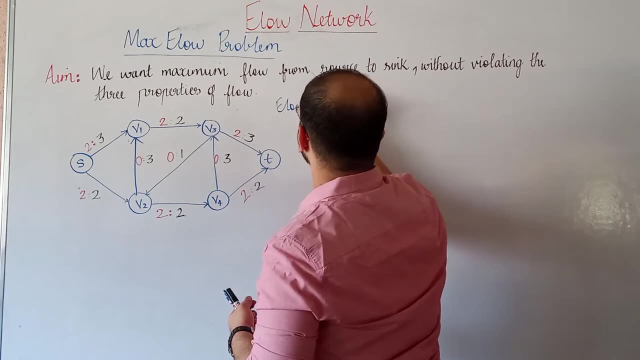 is actually 4.. Right, 2 plus 2, 4 and 2 plus 2, 4.. So earlier it was 3.. Now it has changed to 4.. So this is actually less than the capacity. 3 and it has changed to: 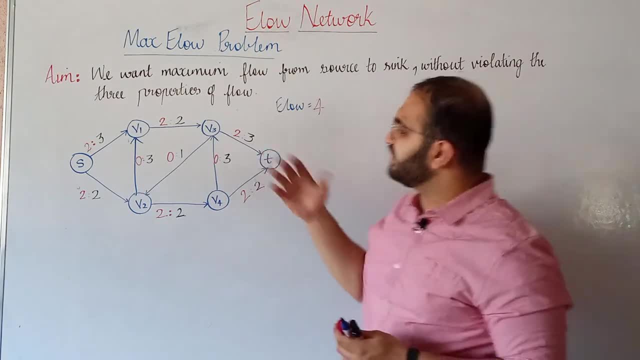 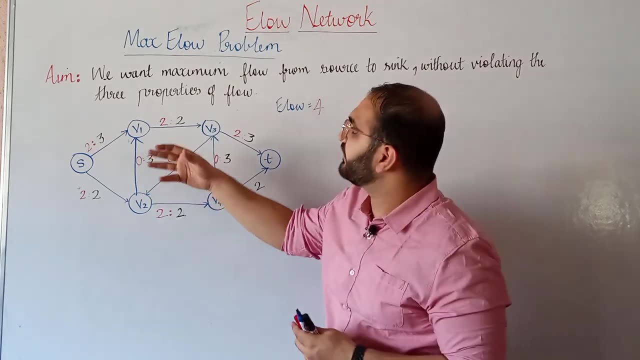 4. Right. So basically, in this case, I knew already that if I decrease this edge, there might be a possibility of an increase in the overall flow of the network. But what if you have got around 10,000 edges in your flow network? 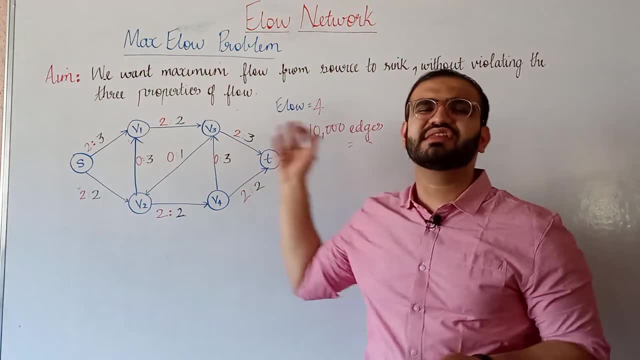 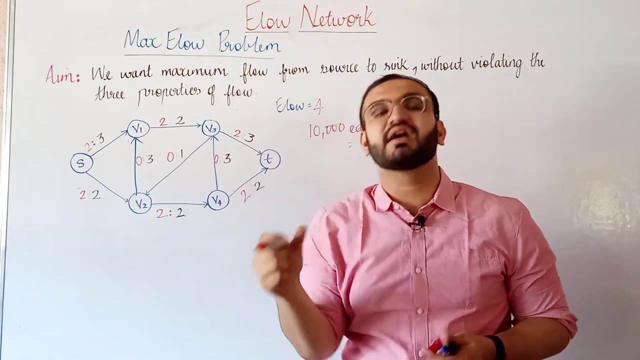 In this case, how will you identify that this is the particular edge whose flow, if I decrease, will lead to an increase in the overall flow? So what we can do over here is that we can increase in the overall flow. It is extremely difficult. 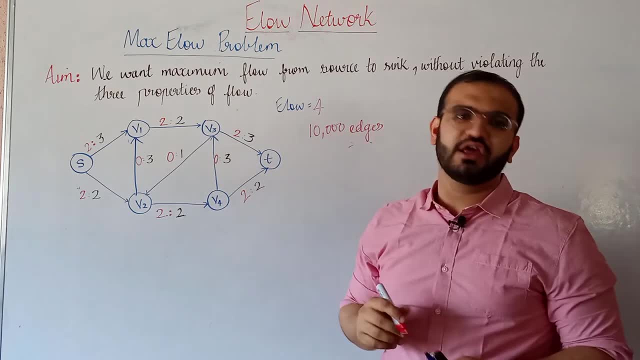 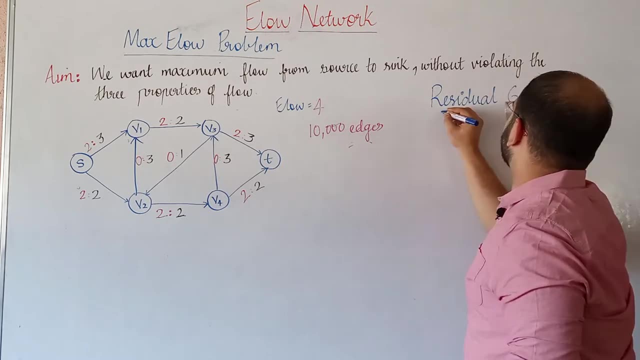 to identify in such a big flow network, Right? So how will you do that? So that is where residual graph comes into the picture. So you might already be knowing the meaning of residual. Residual means something that is net, Right? So this residual graph, 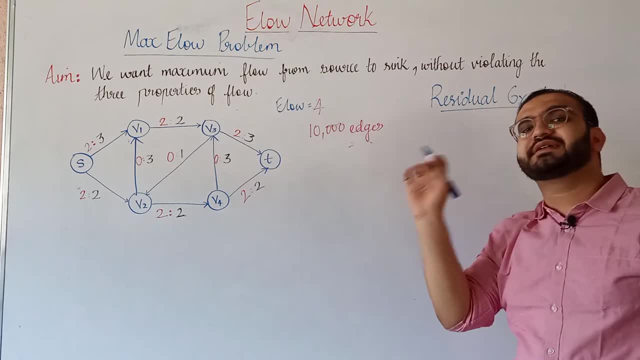 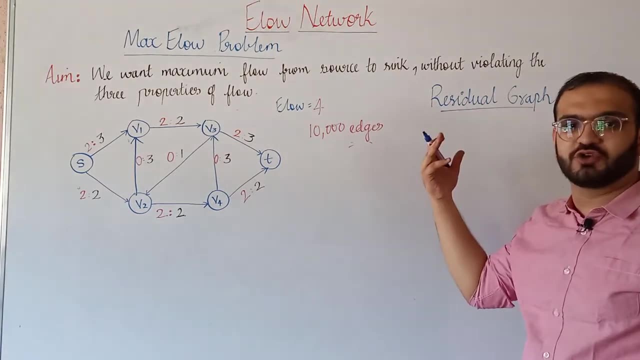 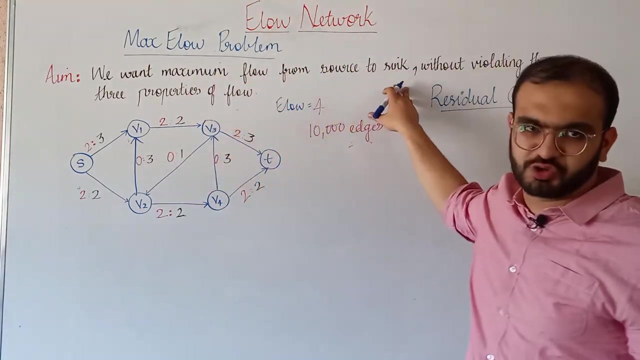 will actually point out at those particular edges where we need to focus in order to increase our overall flow and take it closer to the maximum flow, So that, finally, we can achieve the maximum flow from source to sink Right. So residual graph is going to help us. 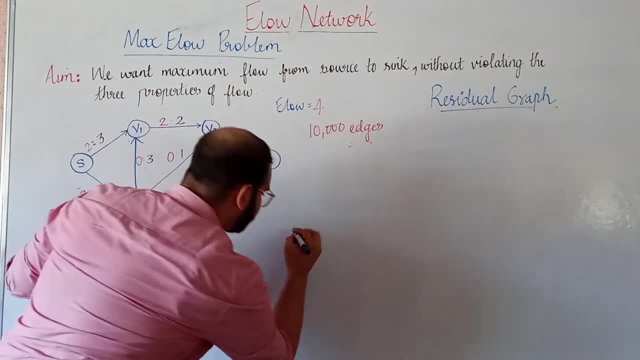 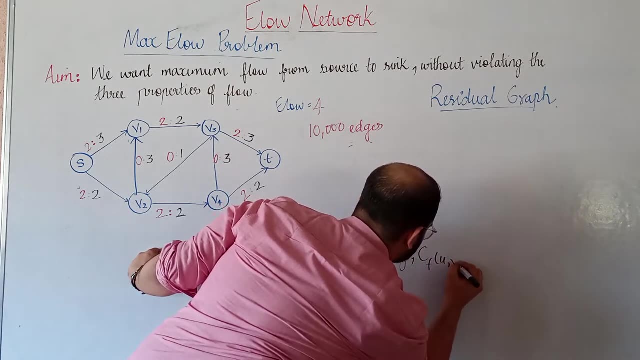 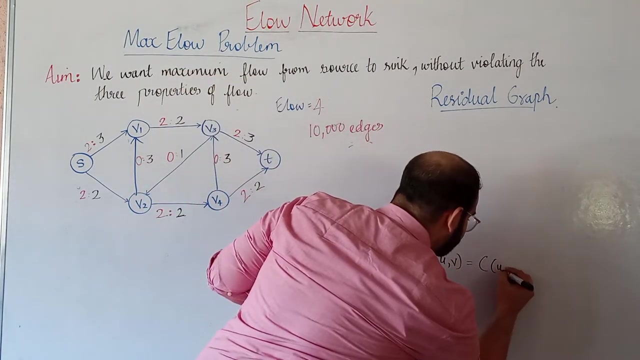 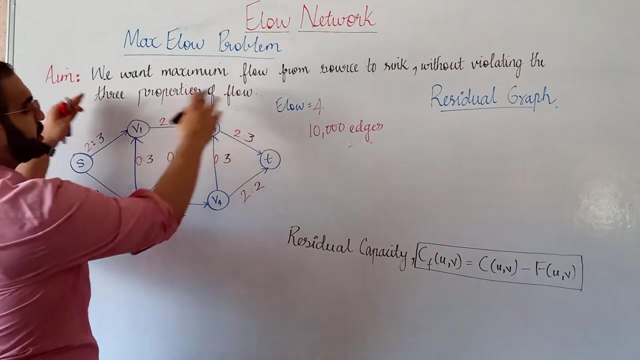 in that And in case of residual graph, we have got residual capacity, which is denoted using CF UB, and this value of this residual capacity is actually equal to capacity from U to B minus flow from U to B. Okay, So now we will draw. 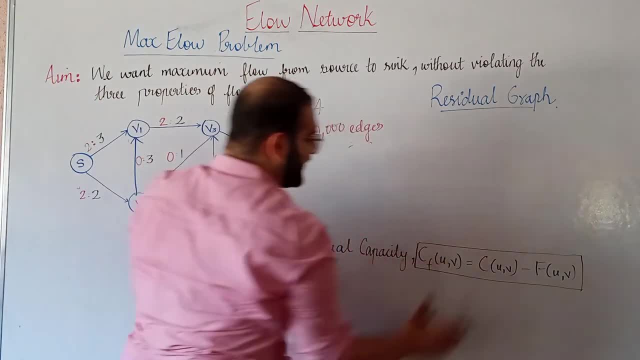 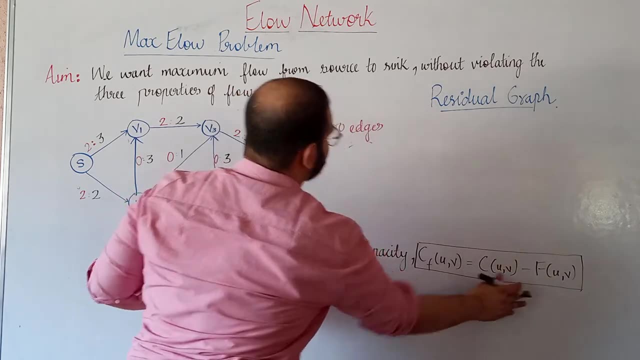 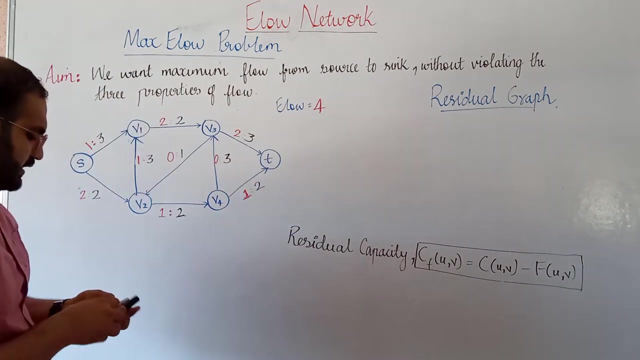 a residual graph for this flow network over here. Okay, And then you will understand that for each and every step, we are actually following this expression or this formula. Okay, So now we are going to draw a residual graph for this flow network over here. 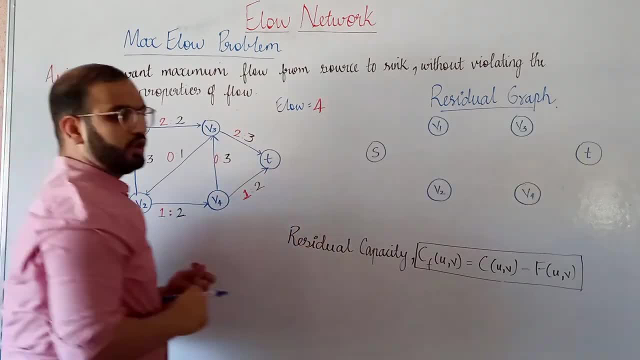 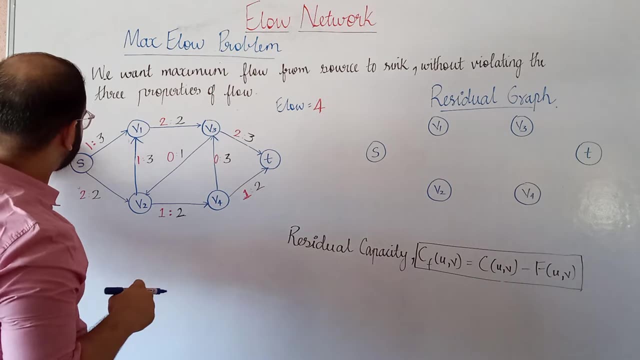 Okay, As we have them in our flow network. Okay, So these are the vertices. Now, as we can see over here, there is already a flow that is flowing from S to B1 and the value of that flow is 1. Right. 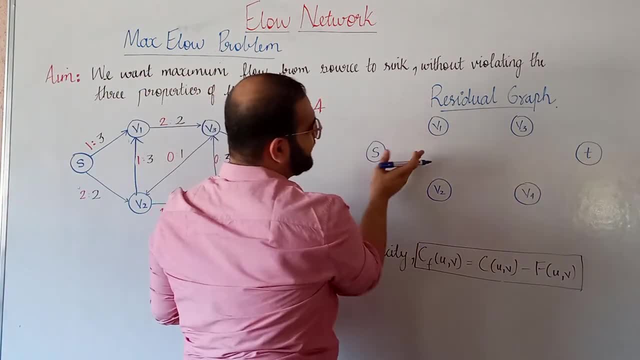 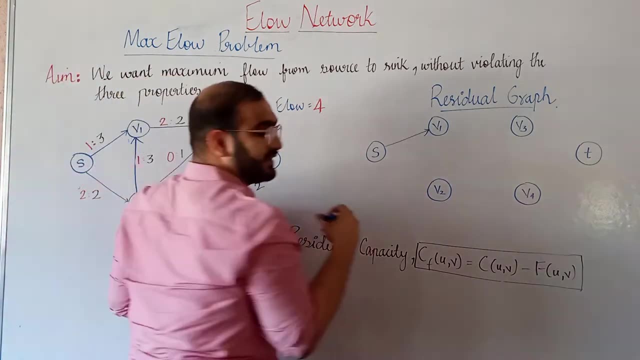 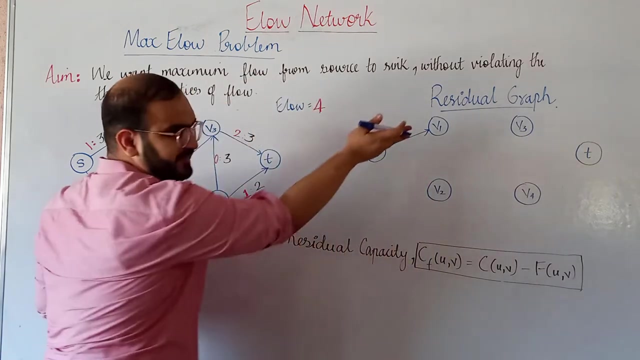 So the residual flow at this path, or the left out flow that is possible at this path, is actually the capacity on this edge minus the flow at this edge. That means of a flow of value 2 from S to B1, because already 1 is flowing. 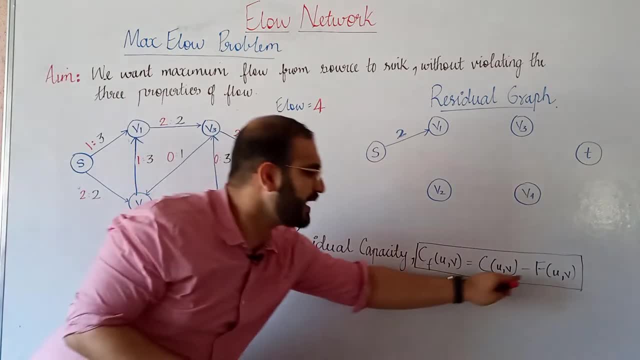 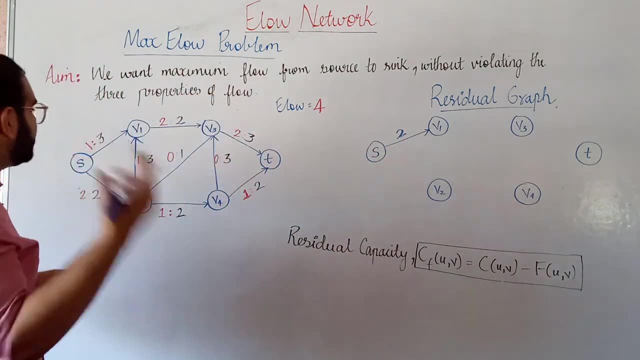 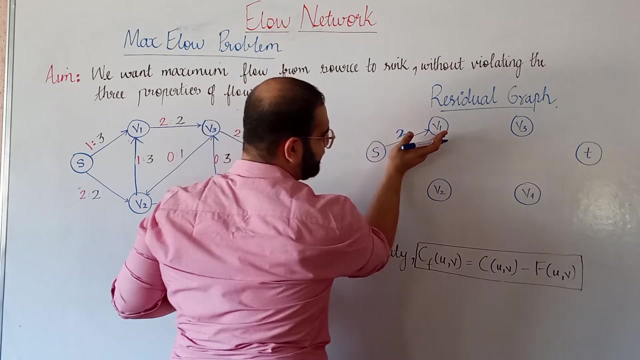 from S to B1 and we did capacity minus flow for this edge in order to determine the residual flow at this edge. Right Apart from that, another thing that we need to do is that, because there is a flow that is already flowing from S to B1, 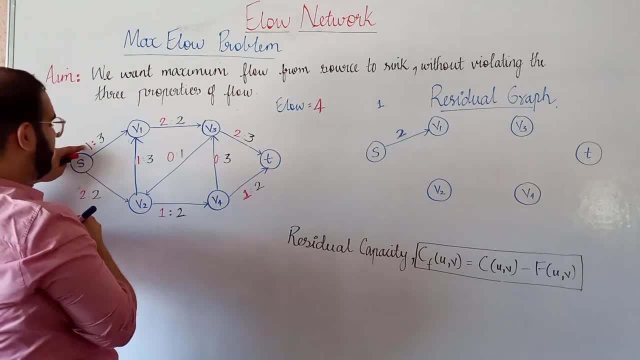 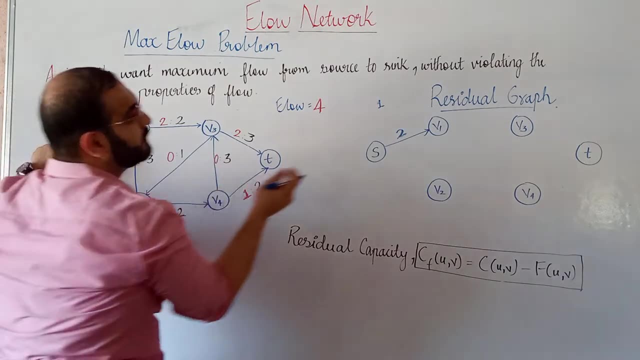 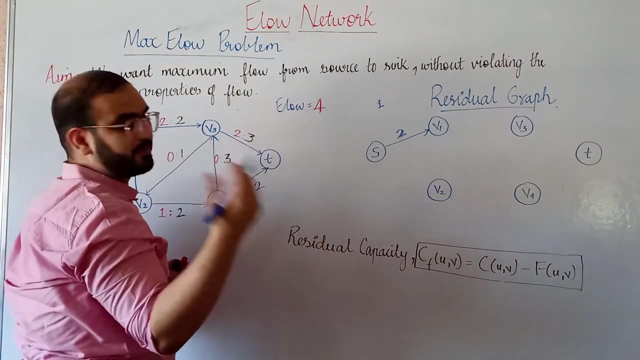 and the value of that flow is 1, as you can see over here. so in order to actually so, in order to denote that flow in this graph, we need to draw an edge in the opposite direction, Right? So basically, I am following the skew symmetry. 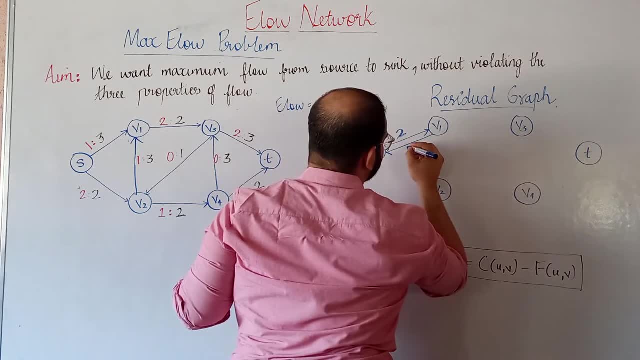 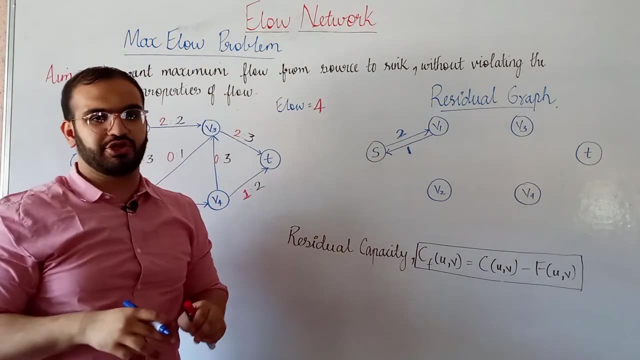 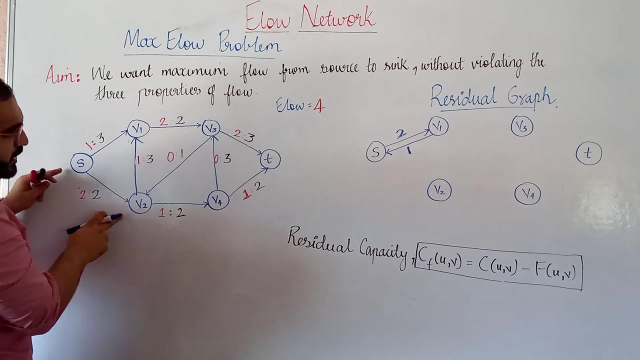 property over here. so we will draw an edge in the opposite direction of the value 1.. Right, Because there was a flow from S to B1, so I drew an edge in the opposite direction. Now, if you look at this edge from S to B2, 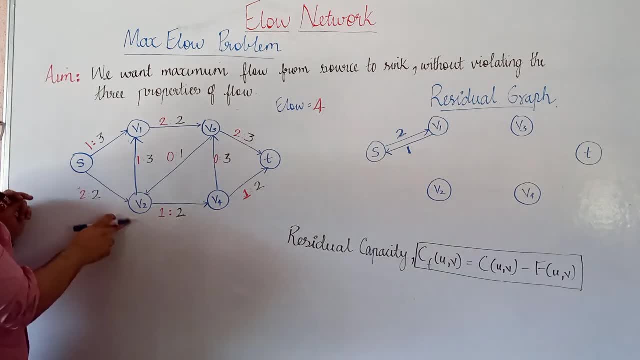 so basically, there is a flow of 2 already flowing from S to B2, so there is no more amount of material that can flow because it is already flowing at its capacity, Right? So we cannot draw an edge from S to B2, rather we can. 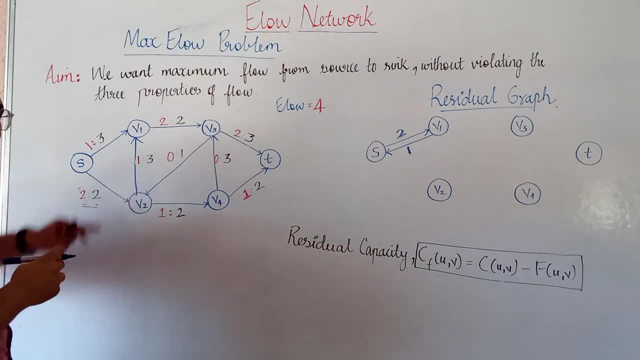 draw an edge in the opposite direction, from B2 to S, in order to denote this flow that is already flowing Right. Okay, Now, if you look at this edge- V2 to V1- so there is a flow that is already flowing from V2 to V1. 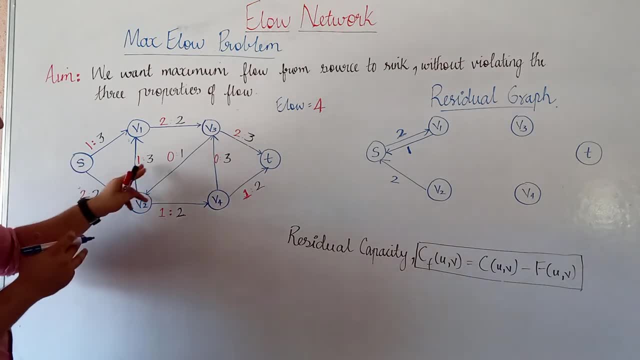 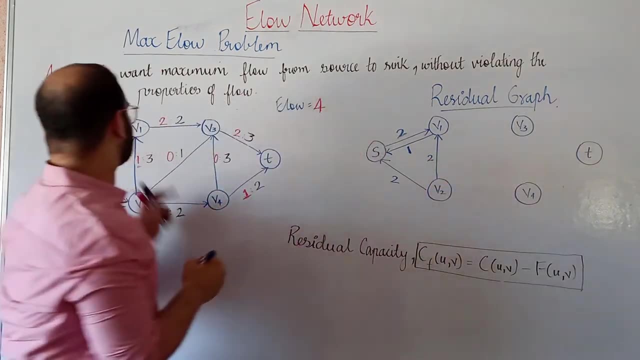 and its value is 1.. So the residual flow that is possible is 3-1, that is, 2, in this direction, right From V2 to V1. and to denote this flow that is already flowing from V2 to V1, we will draw: 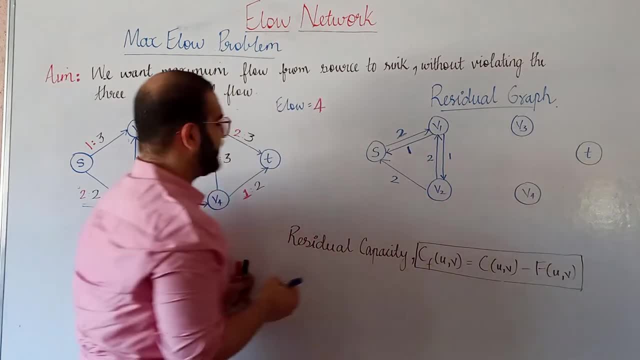 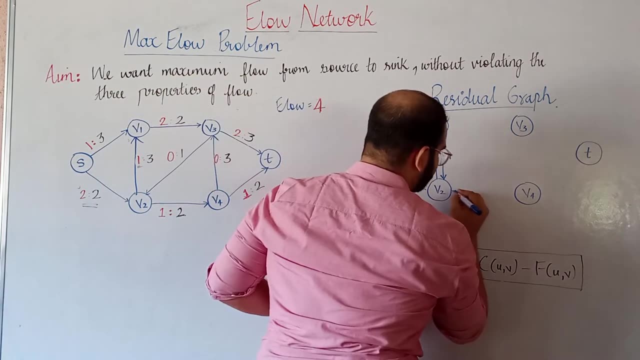 it in the opposite direction, from V1 to V2, and its value is 1.. Okay, Now from V4 to V3. there is nothing flowing in this direction from V4 to V3, so the extra flow or the residual flow that is possible. 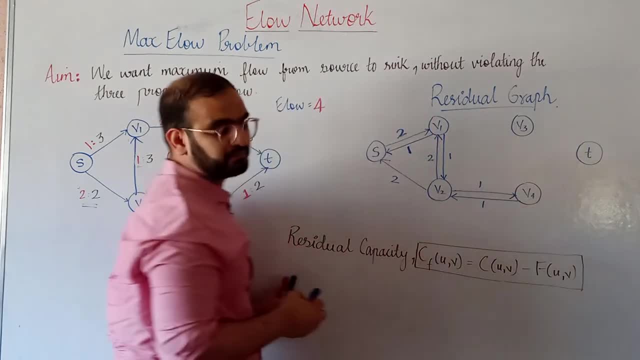 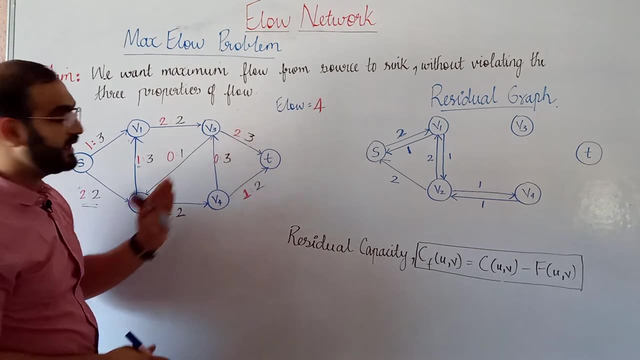 from V4 to V3 is actually 3. Because initially the residual flow that is possible is 1, because 2-1 right V2 to V4: 1 and to denote that flow that is already flowing from V2 to V4. 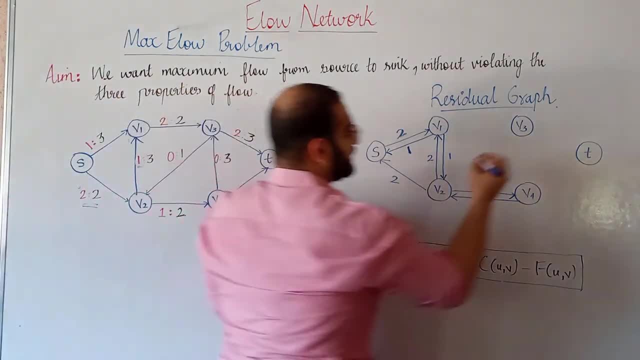 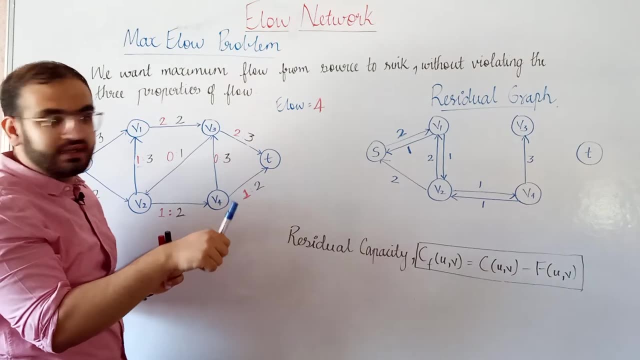 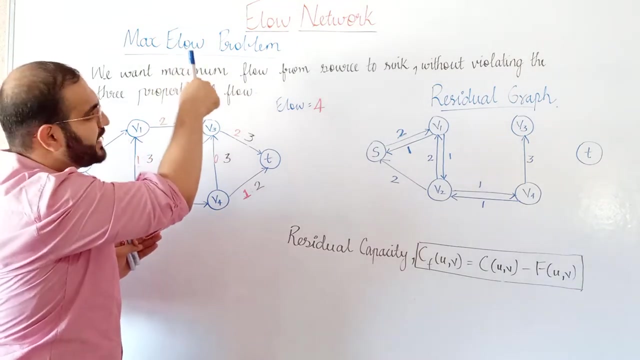 is 1, because initially nothing is flowing in this direction, right? So the residual flow from V4 to V3 is 3, and we don't draw an opposite edge over here, because we don't have to denote any flow, because nothing is actually flowing in this direction. 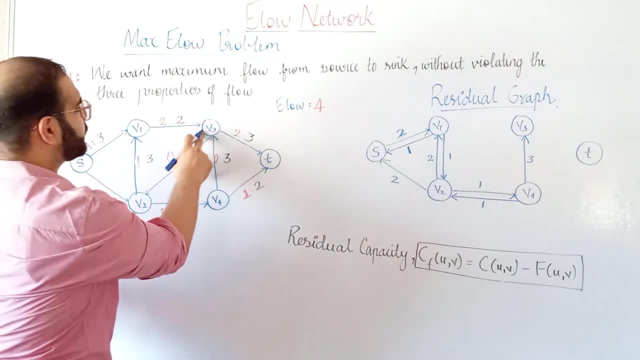 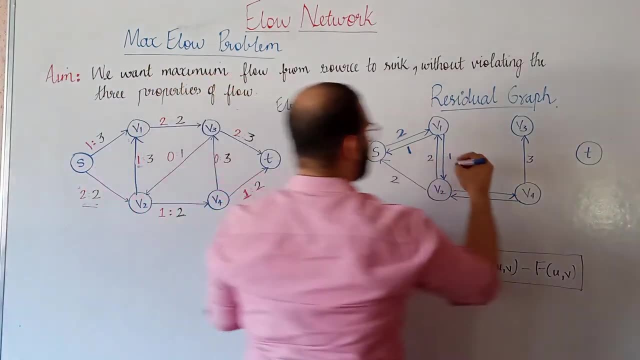 from V4 to V3. so we don't have to draw any edge from V3 to V4 right Now. if we talk from V3 to V2, again nothing is flowing in this direction. so the residual flow is 1 right Because the capacity 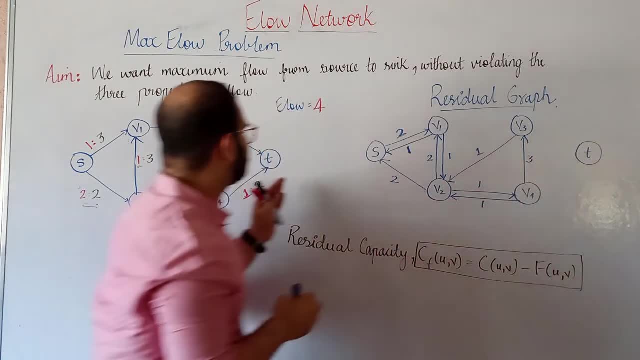 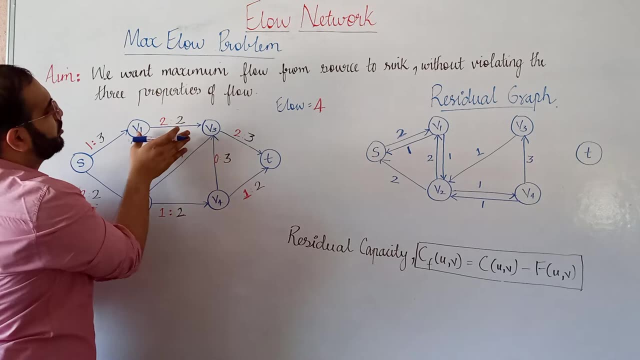 is 1, so the residual flow will be actually equal to capacity. in this case, where nothing is flowing right Now from V1 to V3, basically it is flowing at its capacity, so no residual flow is possible in this direction from V1 to V3. 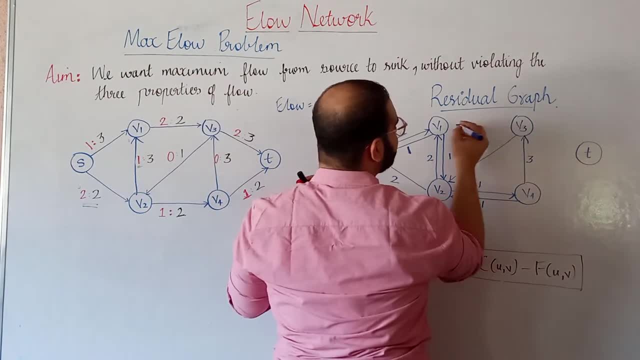 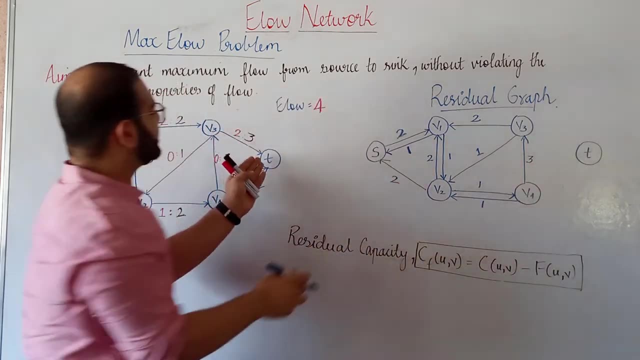 but we will draw flow in the opposite direction using the skew symmetry property. so we will draw from V3 to V1, V3 to V1 and the value is 2. from V3 to T. the residual flow that is possible is 3-2. 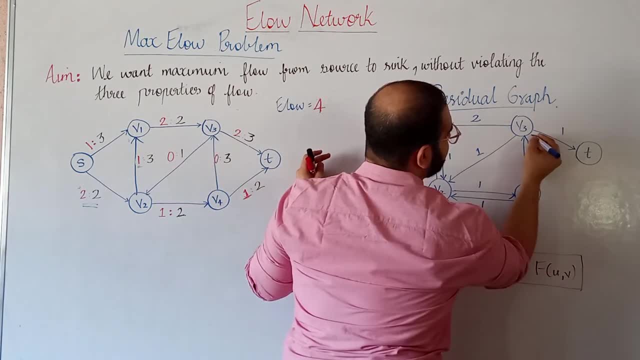 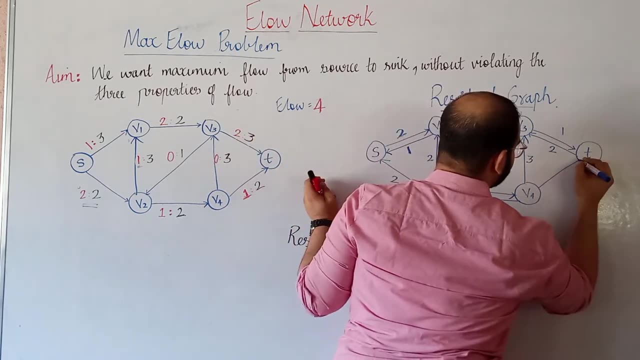 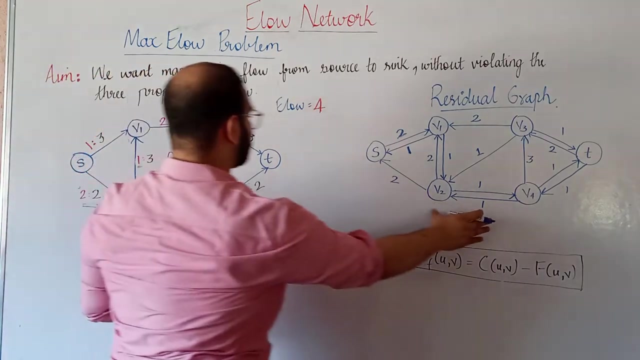 that is 1, okay. and in the opposite direction. we will denote this flow that is already flowing with 2 from V4 to T. residual flow that is possible is 1. in the opposite direction: 1 right. So this is our residual graph. I hope I have. 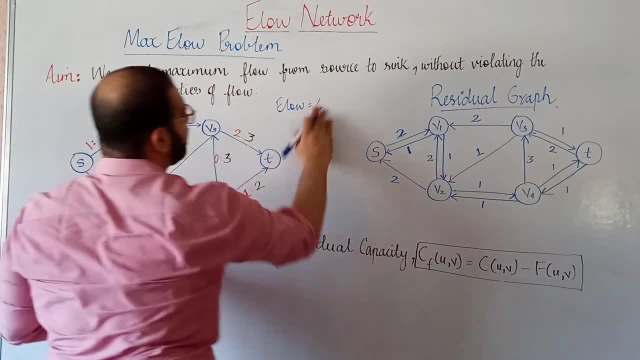 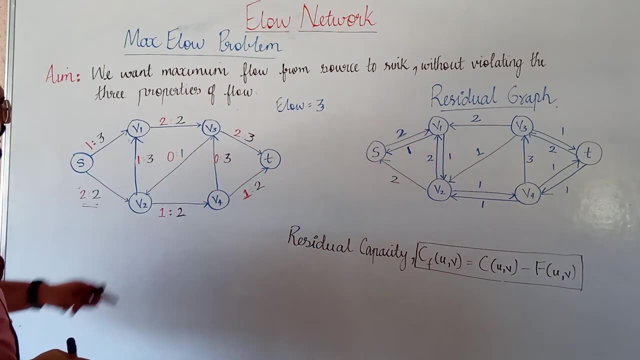 covered each and every edge over here. so in this case I have taken my initial graphs. so this graph, as you can see, is 2 plus 1, 3 itself right. So earlier, what I did was I decreased the value of flow at this edge from 1 to 0. 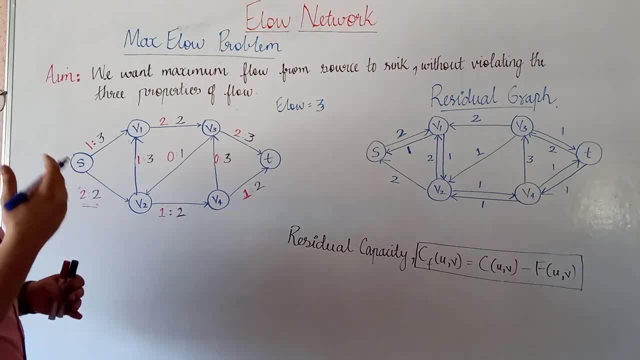 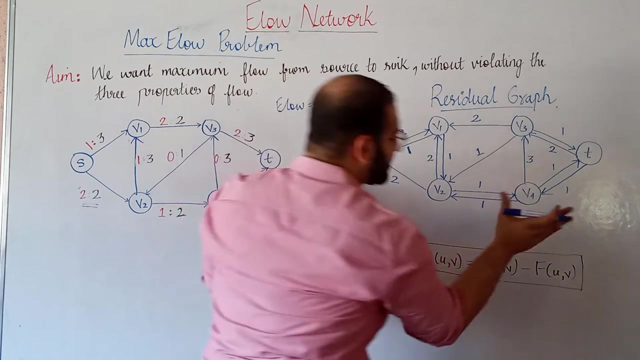 and then I made all the different changes so that each and every vertices follows the flow conservation property and finally I made the flow to 4 right. But then we saw that it is very difficult to determine such kind of edge flow in a residual graph. so if 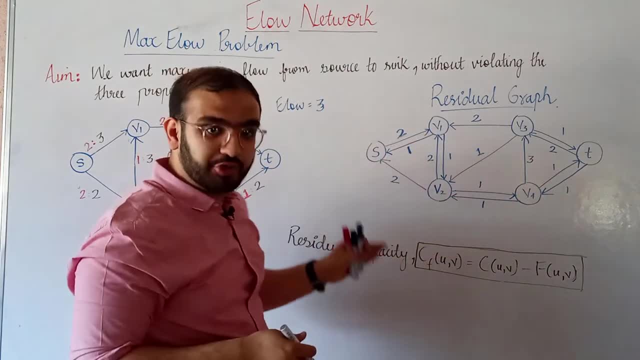 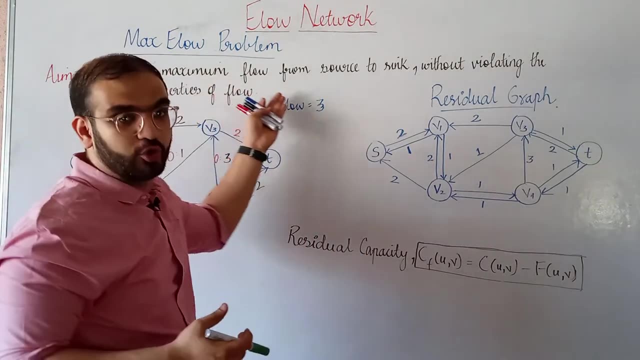 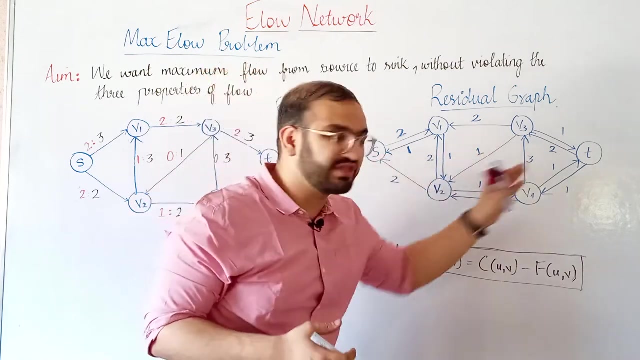 there is a path possible from the source to the sink. in the residual graph that means there is a scope of increase in the flow or the overall flow of our flow network. and if such kind of path is not possible from the source to the sink, any path is not. 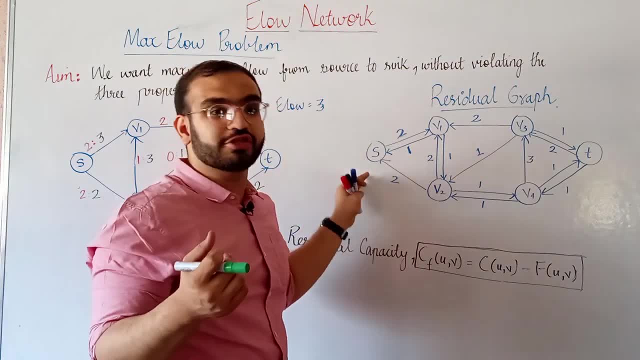 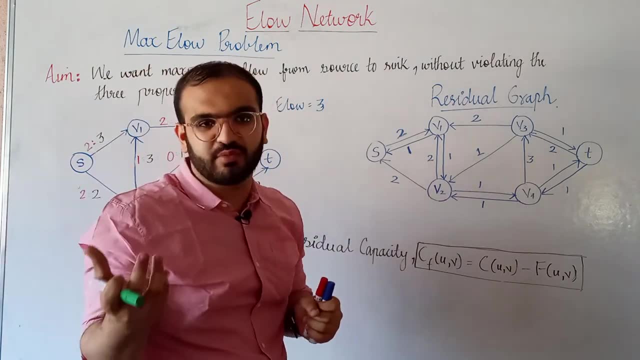 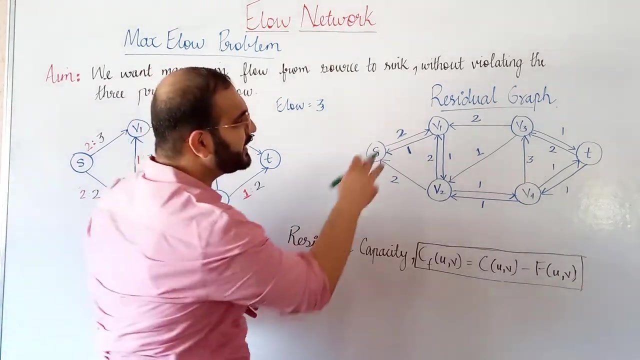 possible from source to sink in a residual graph and that flow that we already have will be called as our maximum flow, right? So here I cannot call flow of 3 as maximum flow. why? Because if I look at my residual graph I can see that if I go. 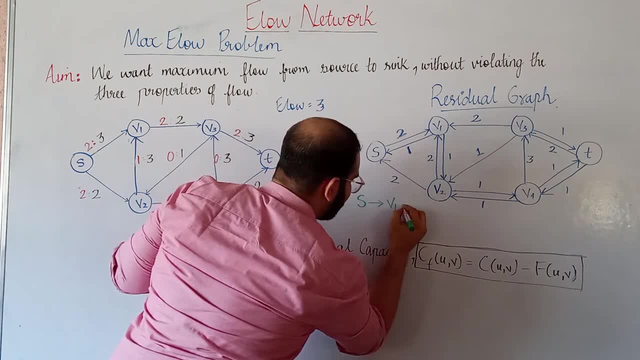 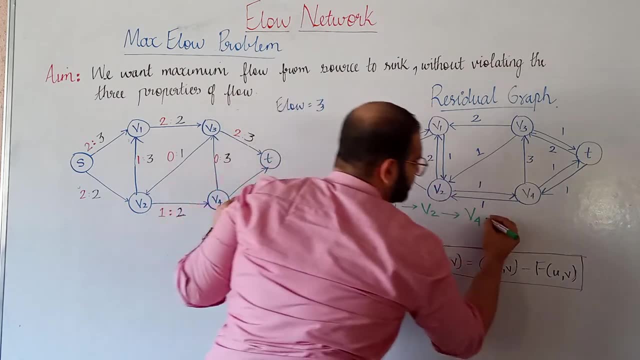 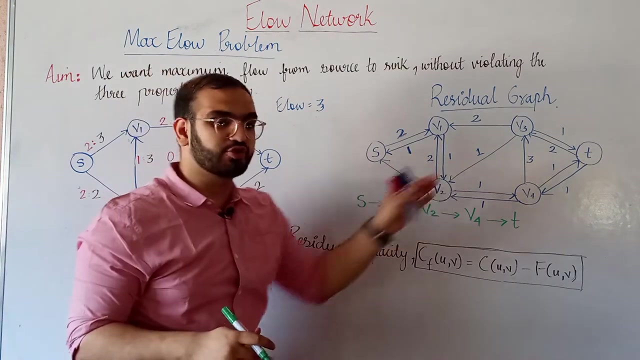 from S to V1, from S to V1, and then if I go to V2, and then if I go to V4, from V2 to V4 to V5. there is such kind of path possible, right, And such kind of path from source. 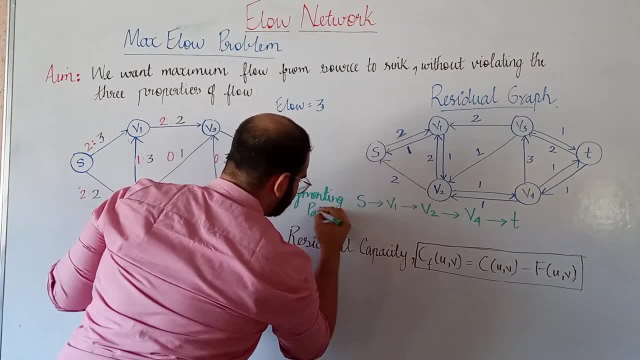 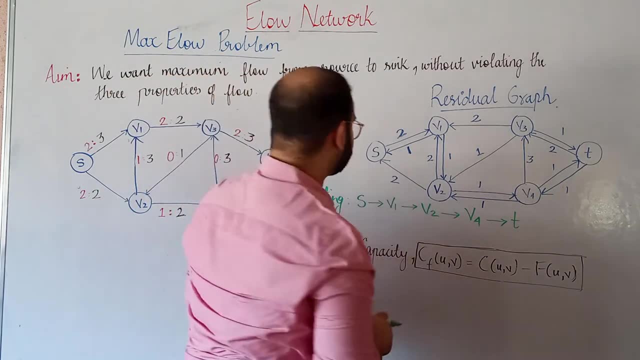 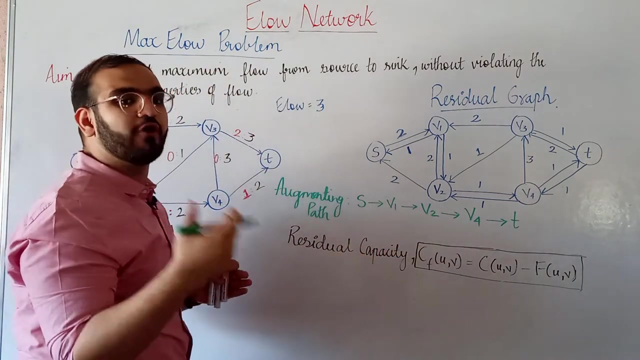 to sink in a residual graph is actually known as an augmenting path. so this path that I have written over here is an augmenting path which we derived out of our residual graph. okay, So if any augmenting path exists in our residual graph, okay. 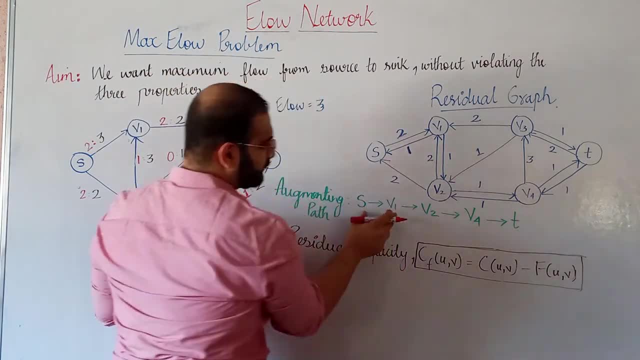 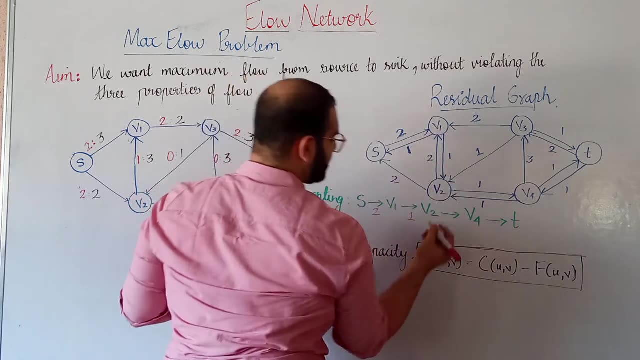 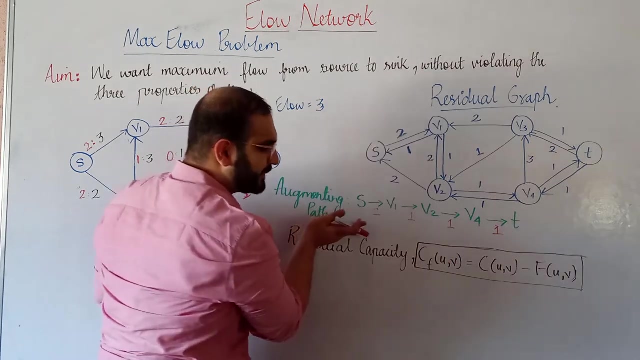 So now if I also write down the flows on these edges, so from S to V1, the flow is 2. from V1 to V2, the flow is 1. from V2 to V4, it is 1. from V4 to T, it is 1. 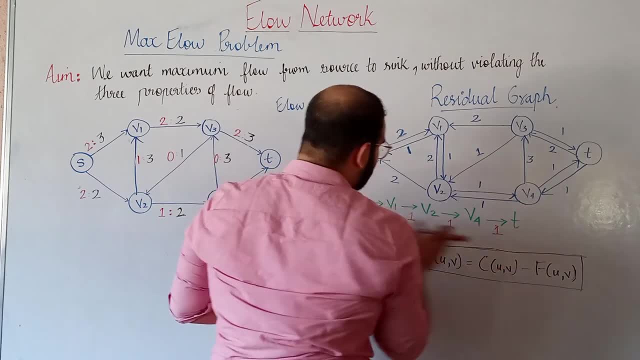 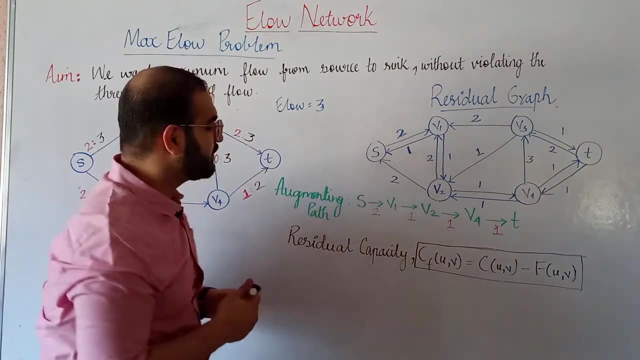 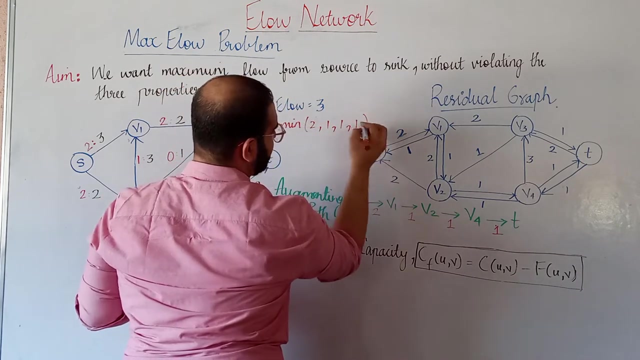 so the flow of the material that is possible, or the maximum flow that is possible from across this entire surface, is the minimum of all these flows. right, And the minimum of all these flows, the minimum of 2,1,1,1 is actually 1. 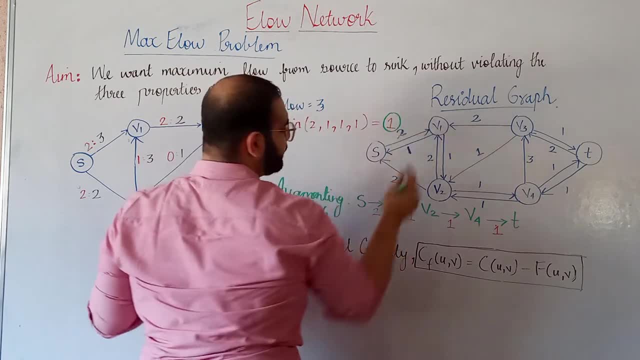 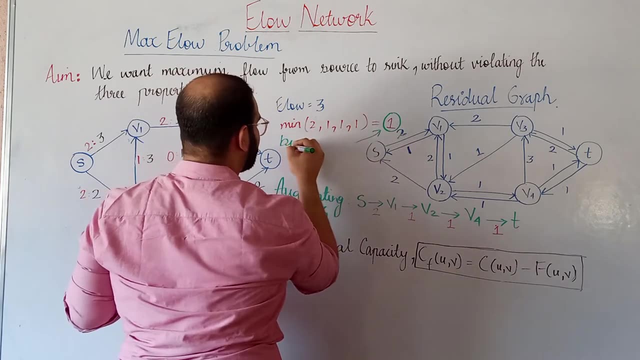 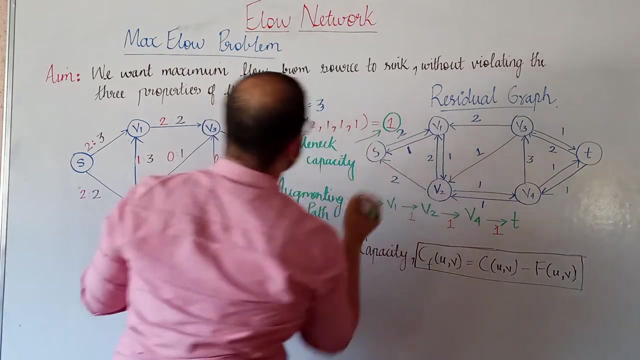 and this 1 that I got over here will actually determine the extra flow that is possible in the flow that we already have, and this 1 is also known as the bottleneck capacity right, So we learnt that an augmenting path is a path in our 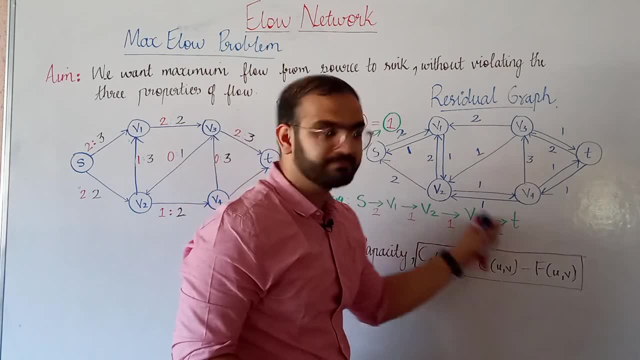 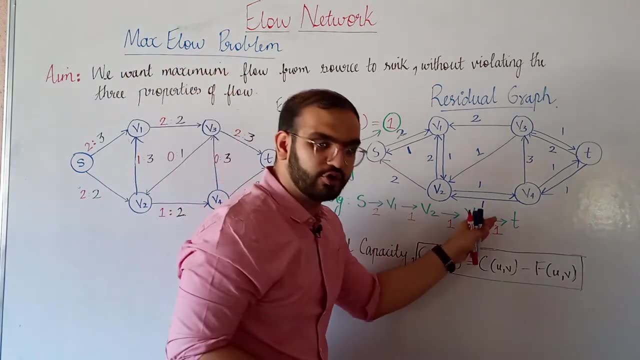 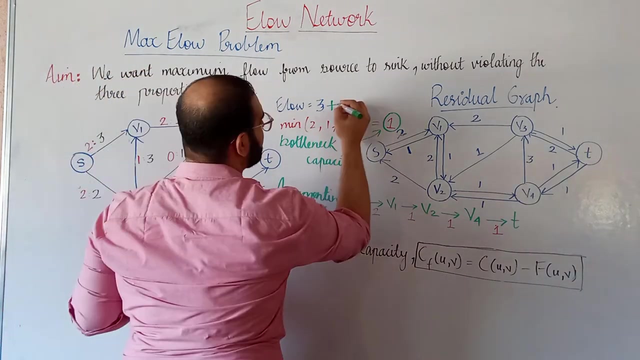 residual graph from source to the sink. and bottleneck capacity is the minimum out of all the flows in the augmenting path. so because I have got an augmenting path with a bottleneck capacity of 1, so that means there is a scope of increase of 1. 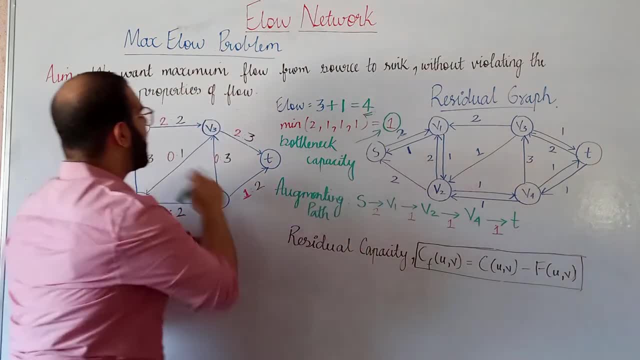 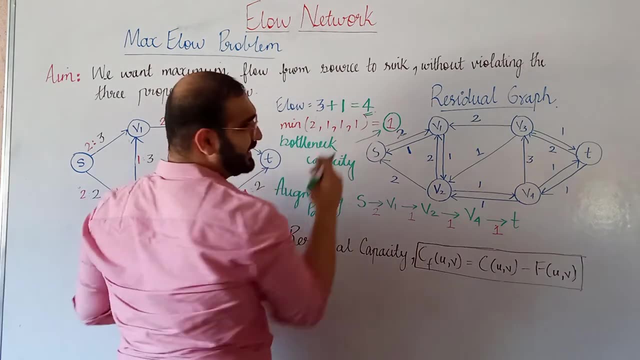 in my flow can be 4, right. So how I will make it 4 in the flow network, We will talk about it later when we discuss the 4 Ferguson algorithm. but right now I can say that this flow of 3 that I had earlier 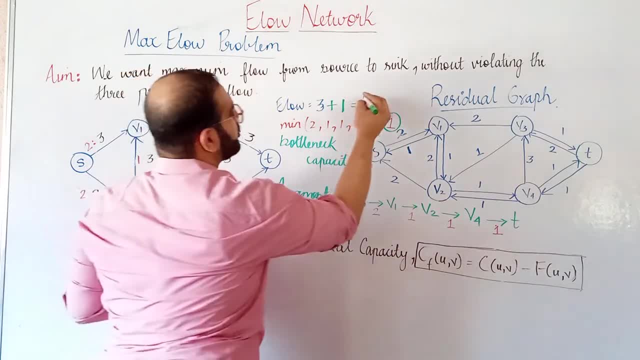 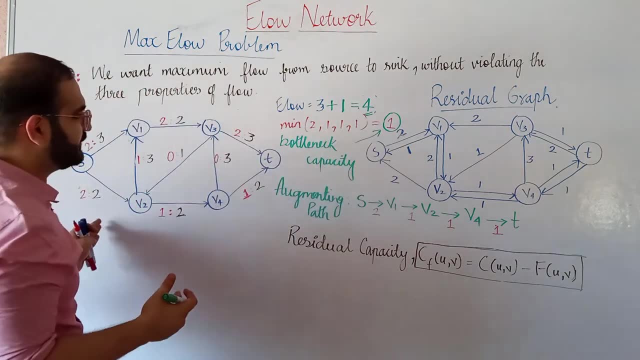 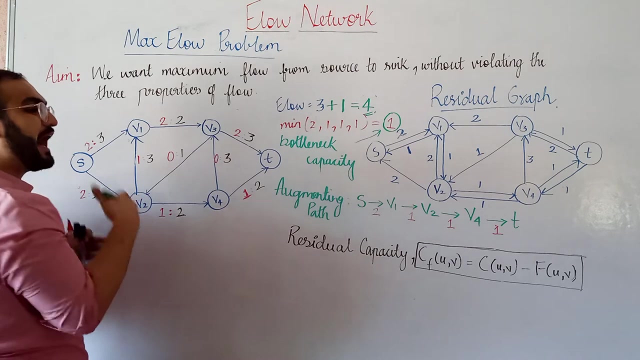 was not the maximum flow and here we are doing the maximum flow problem. so again is 4 the maximum flow. So for that we actually need to modify our flow network by including this additional flow into our flow network and out of that we need to derive. 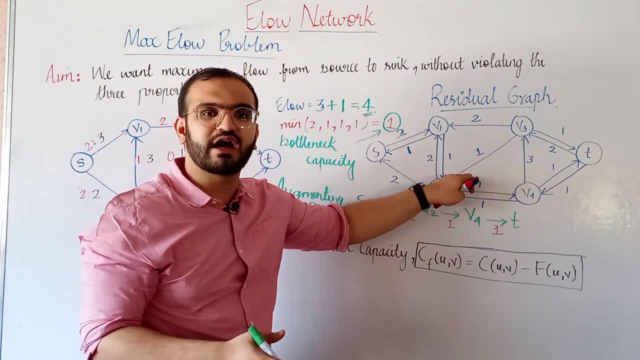 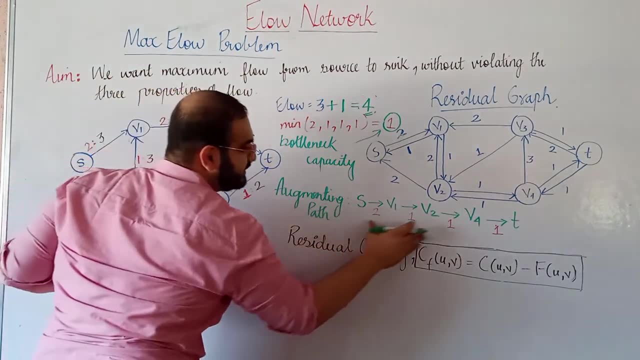 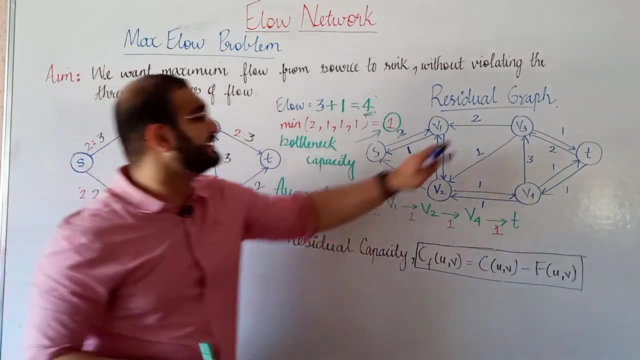 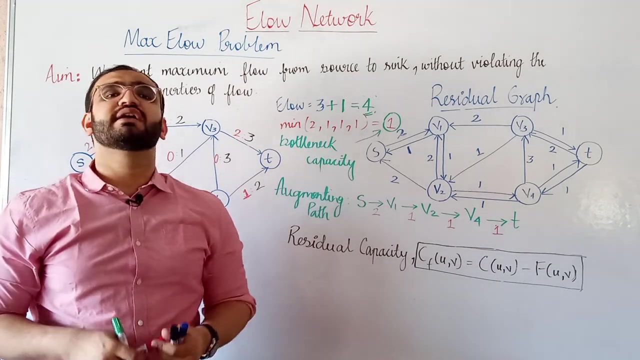 another residual graph that will be different from this residual graph, because that residual graph will actually be derived after we include this flow into our already existing flow right? So now we have already learnt residual graph, residual capacity, bottleneck and the flow of the flow network. so now we 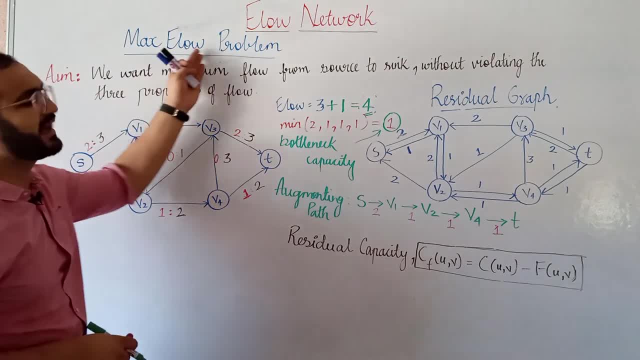 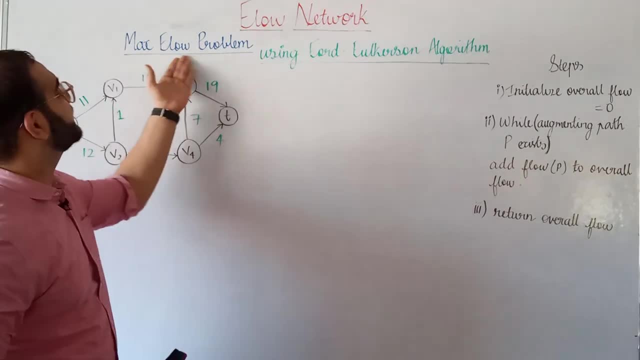 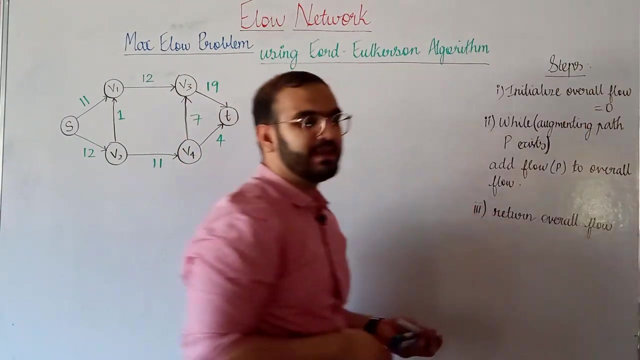 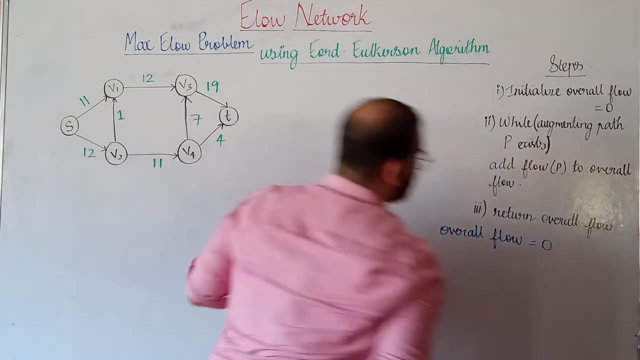 have to start the 4 Ferguson algorithm in order to solve the maximum flow problem. so now let us look at the 4 Ferguson algorithm in order to solve the maximum flow problem. so what are the steps of this algorithm? So the first step is that we need to 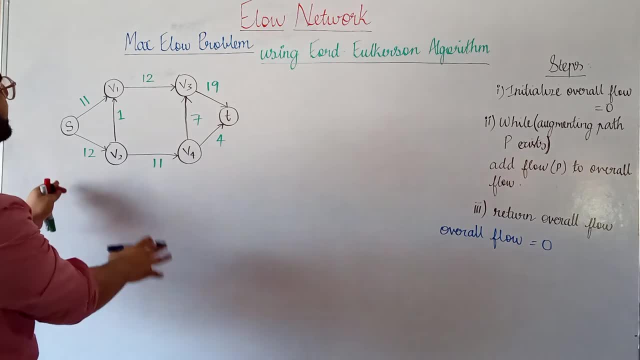 initially. so we are looking at this flow network. so initially the flow in this flow network or the overall flow in this flow network is 0. so I have written down the capacities for each and every edge over here. you should not confuse them with the flows. so all these 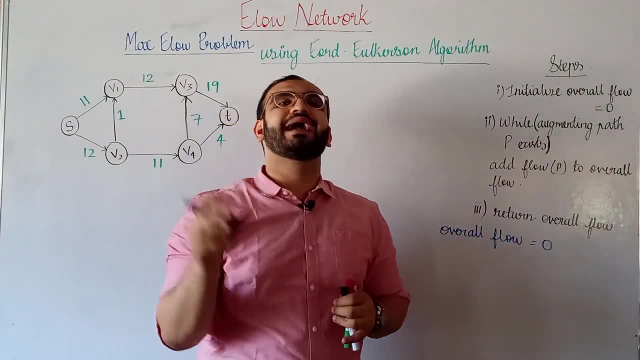 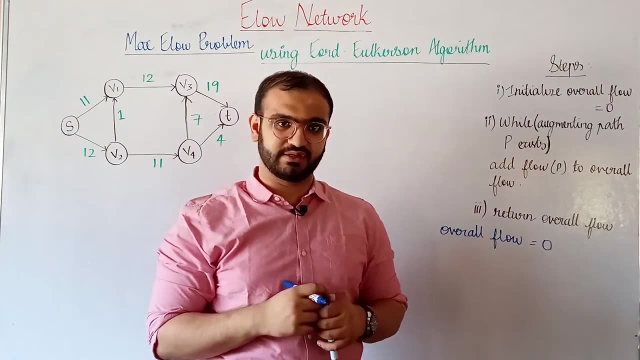 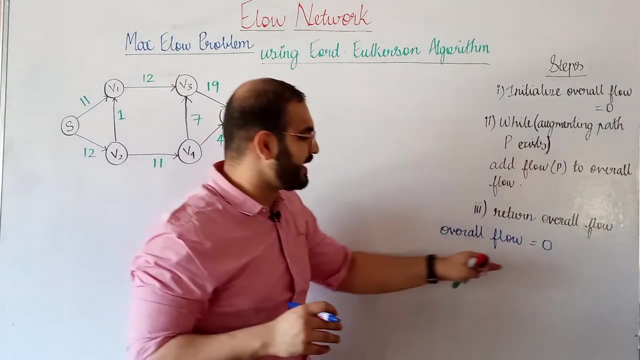 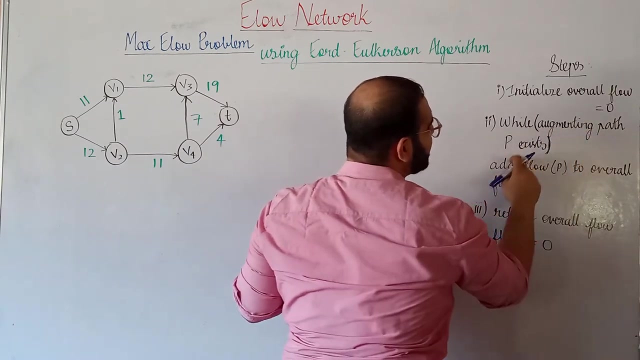 green ones are actually the capacity of each and every edge and in the residual graph, if we find an augmenting path- so the bottleneck capacity across this augmenting path, we will add that bottleneck capacity to our overall flow. or basically, as you can see in this step. 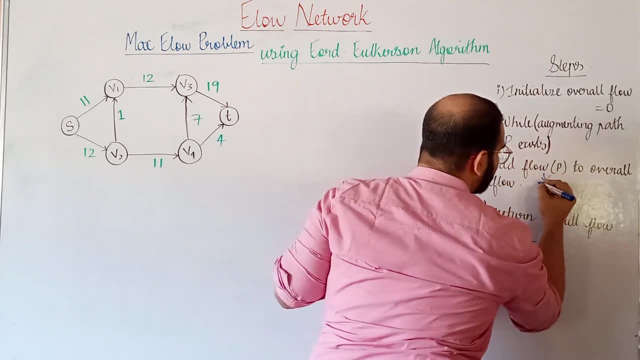 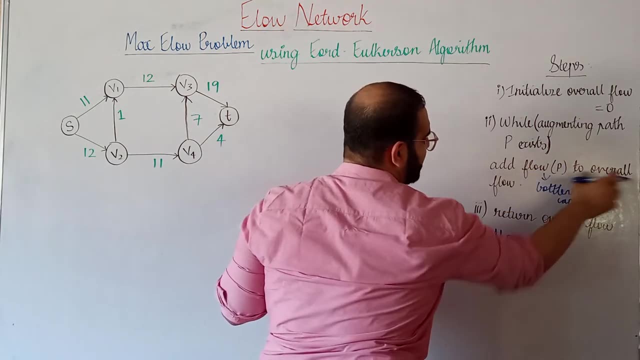 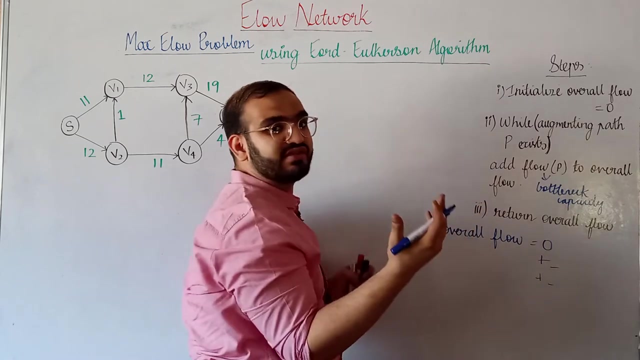 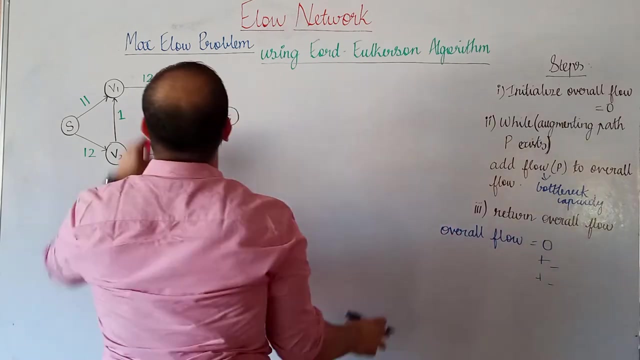 while augmenting path P exists in our residual graph, we will add the flow of P or we will add bottleneck capacity to our overall flow. so we will keep on adding it right until an augmenting path exists in our residual graph and, finally, we will return this. 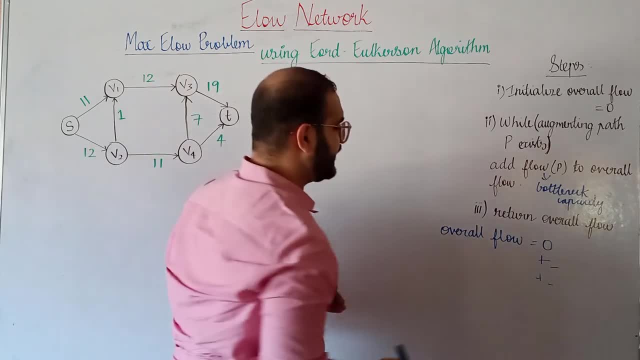 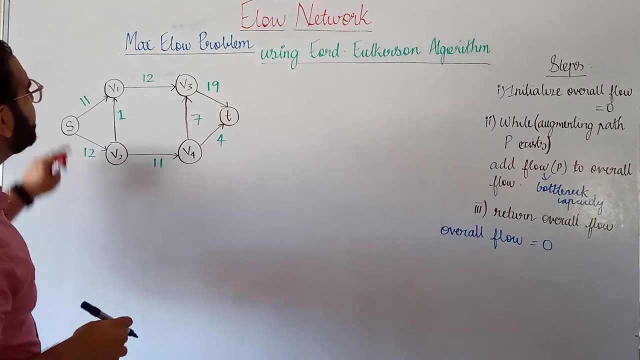 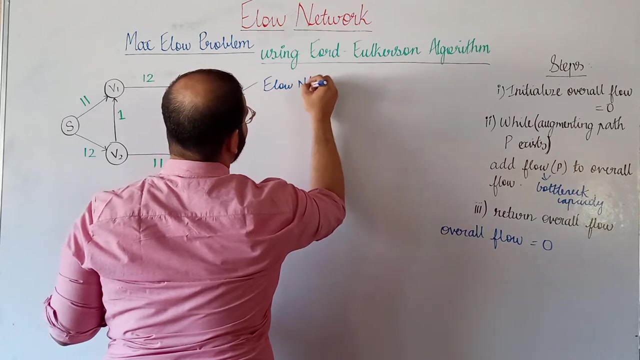 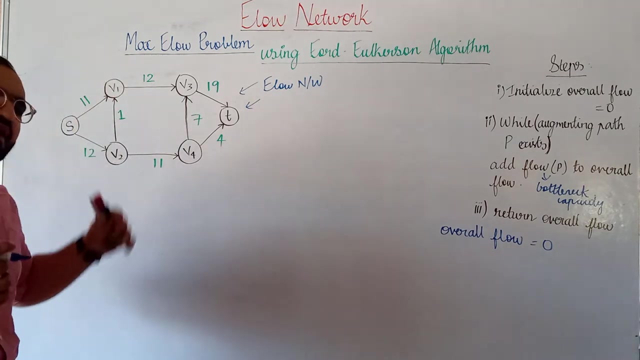 overall flow and this will actually be the maximum flow that is possible over here. now, if you look at this graph, this is basically our flow networks graph, right? at the same time, this is also our residual graph. why am I calling the same thing as my residual graph? 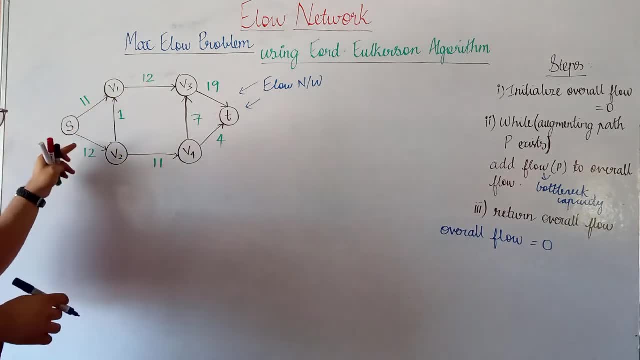 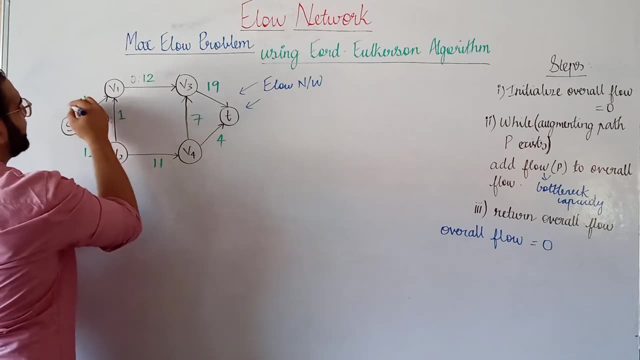 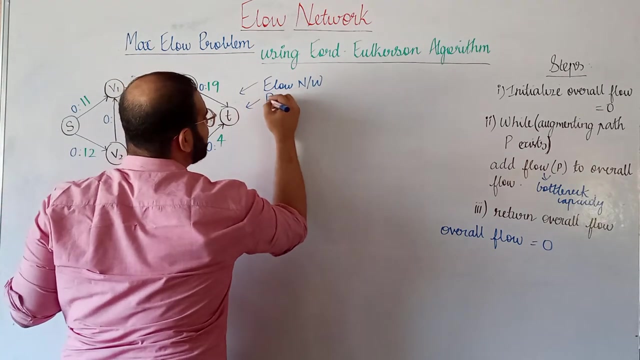 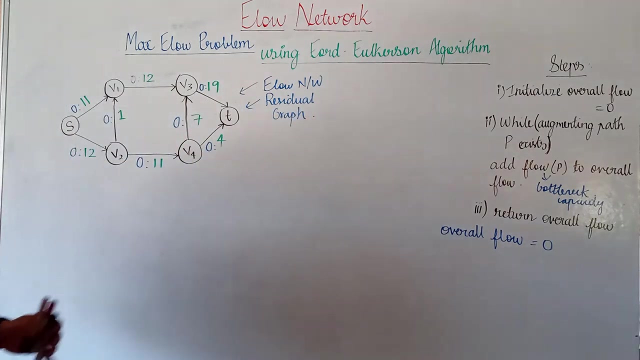 because initially, the flow at each and every edge is actually zero, right? so basically, it is not zero, zero. so basically, this is also my residual graph in the initial case. right, this is also my residual graph, right? so now, as we say, in the second step, we need to. 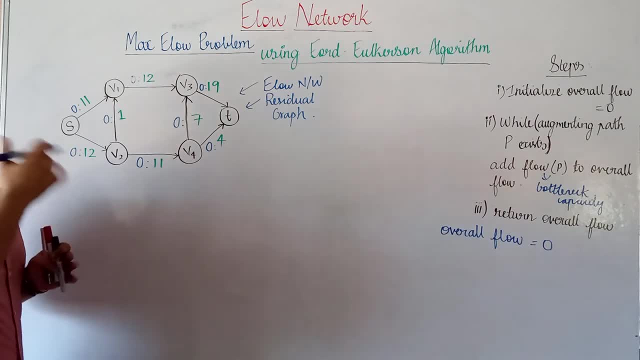 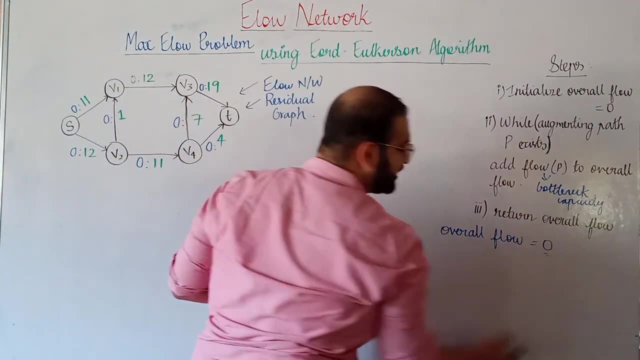 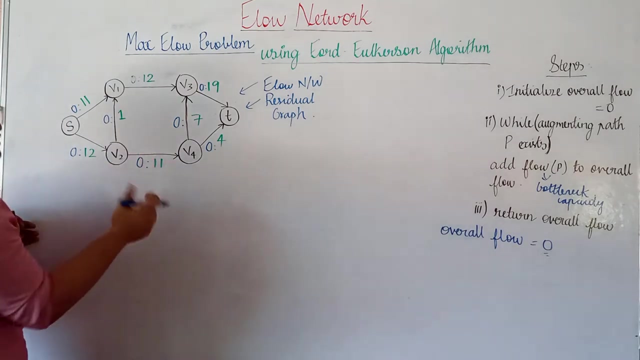 find an augmenting path. if an augmenting path exists in this residual graph, that means there is a. so let us see if an augmenting path is possible in this case or not. so let me just remove the zeros so I can see that many paths are possible. 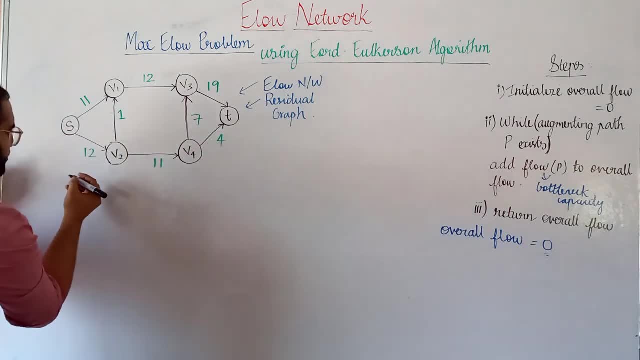 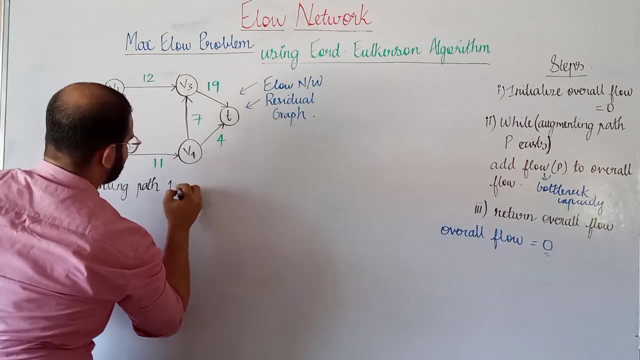 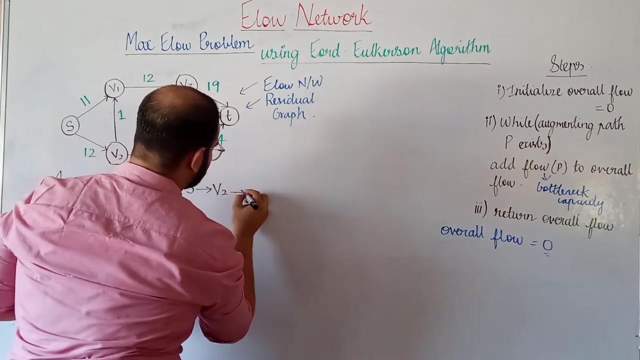 but let me take the first augmenting path from source to sink so I can see what: from s to v2, v2 to v4 and v4 to t. so the augmenting path one is actually equal to s, to v2, to v4 and v4 to 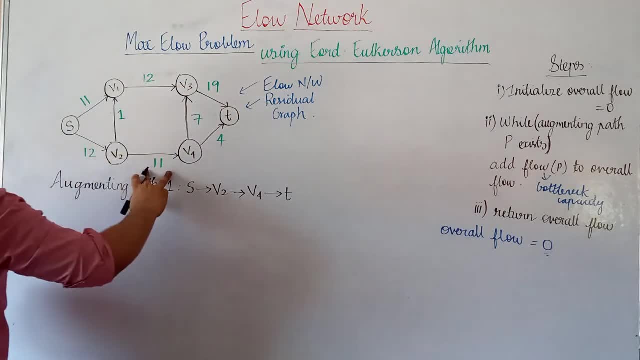 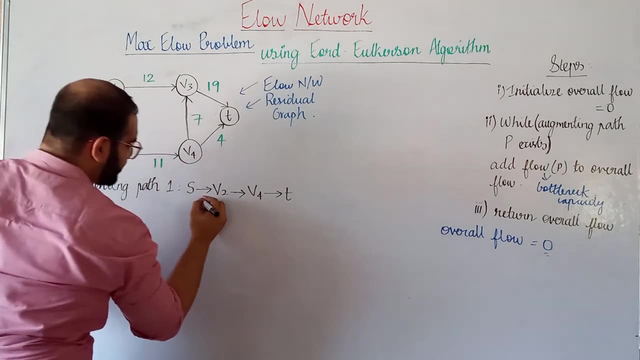 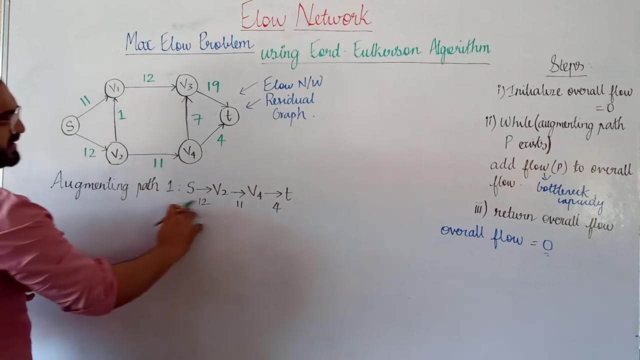 c. okay, and if I write down the residual flows, as this is also a residual graph in the initial case, so the flows, so the flows are twelve, eleven and four, so in this case our bottleneck capacity is, or the minimum out of all these is four, right? so basically, 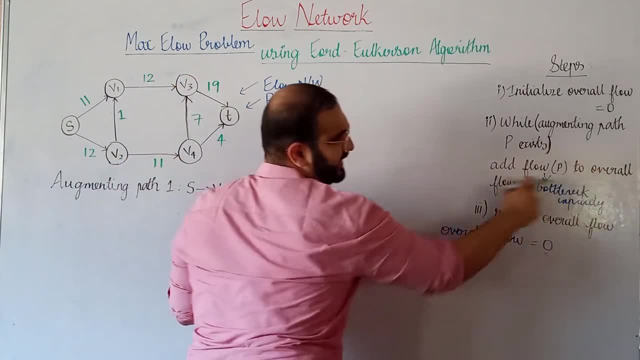 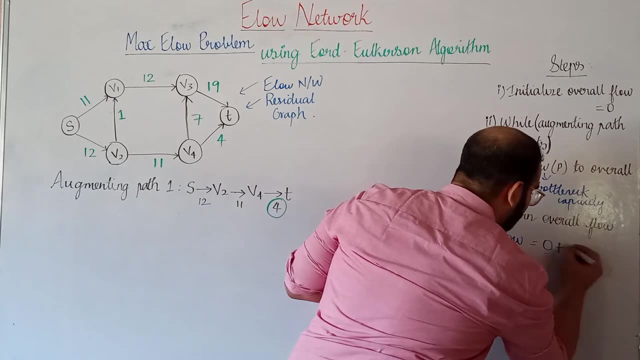 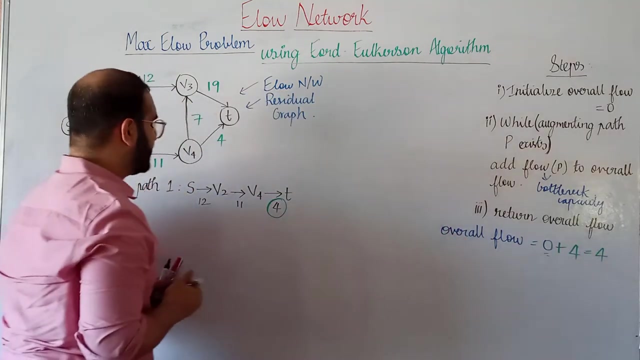 this is what we are going to add in our overall flow. so we found an augmenting path and the bottleneck capacity is something we are going to add in our overall flow. so the bottleneck capacity is four. right, so our overall flow is four. okay, so now, when we add, 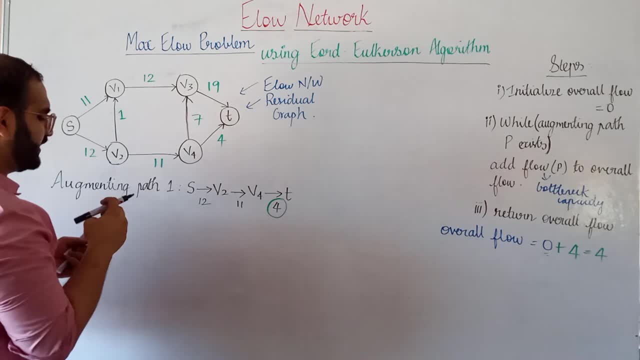 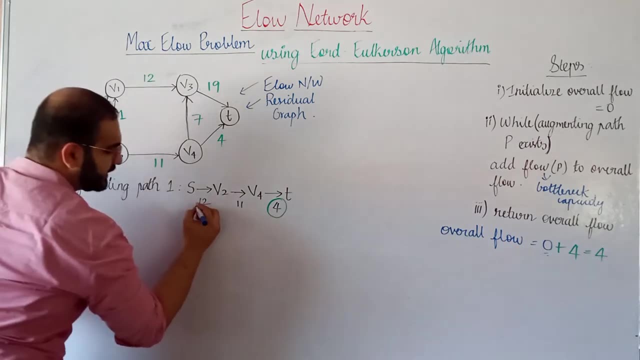 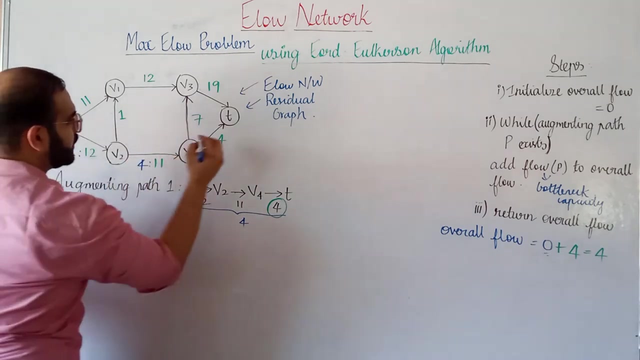 this flow into our flow network. so our flow network is going to change, right, so how our flow network will change. so we also have to denote basically four, right, so I can draw from s to b to four, four and again four. okay, but after drawing this flow, 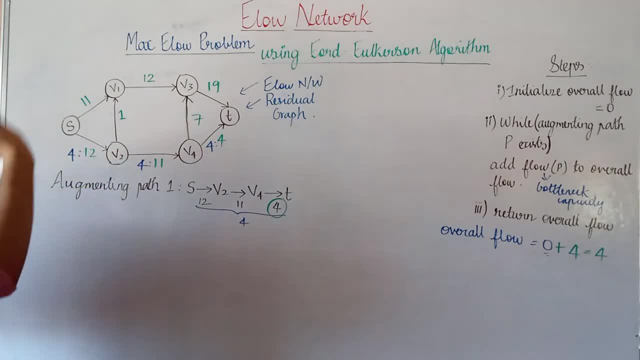 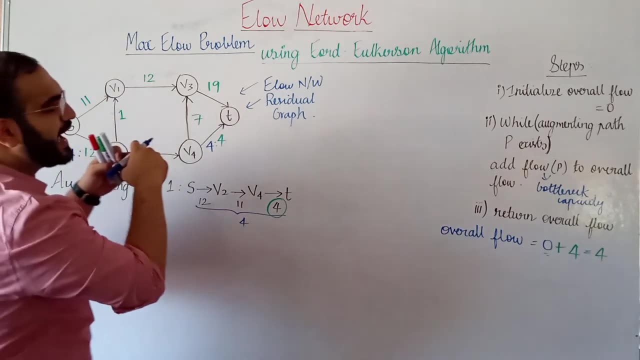 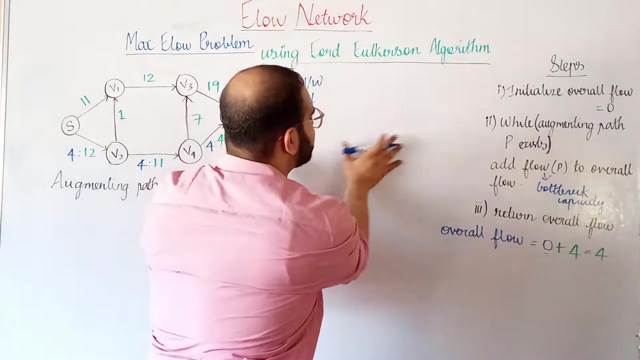 over here in this augmenting path, my I have a different residual graph right because, as you can see, this path has changed or the flow across this path has changed, so I get a different residual graph out of this flow network over here, so this will not remain. 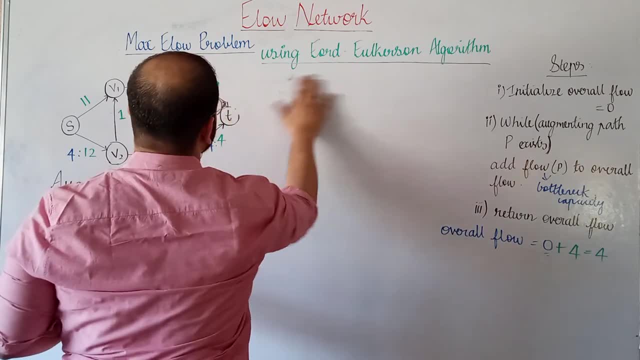 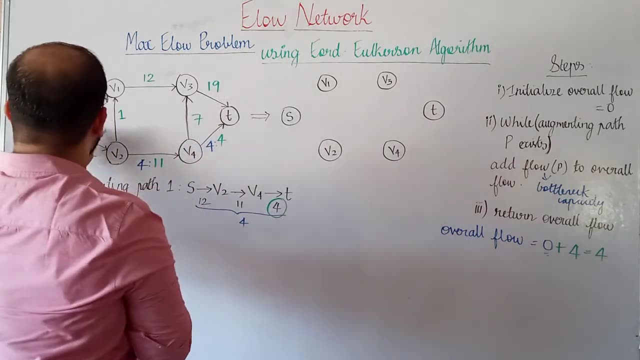 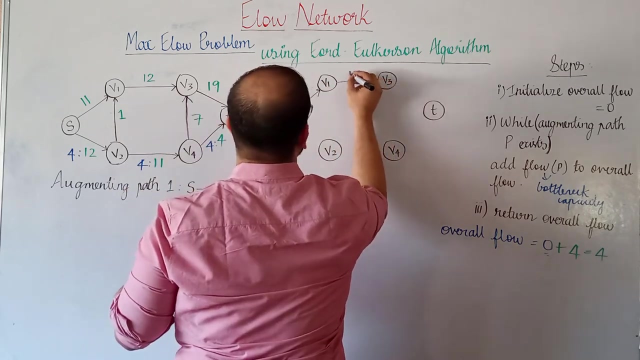 a residual graph. we will get a new residual graph for this flow network, so I have already shown you how to draw a residual graph out of a flow network. let us do it once again. so, from s to b1, there is no change. it will remain 11. 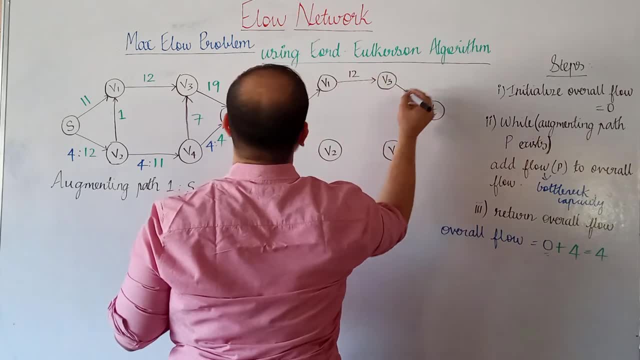 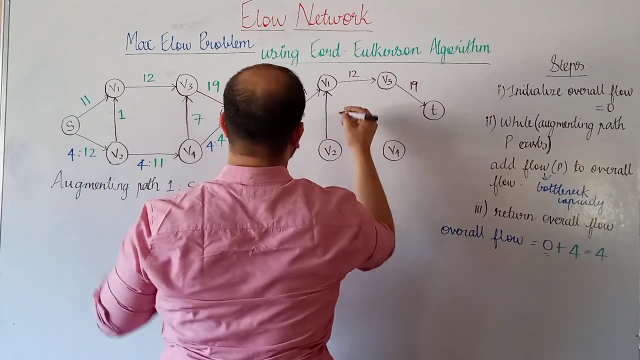 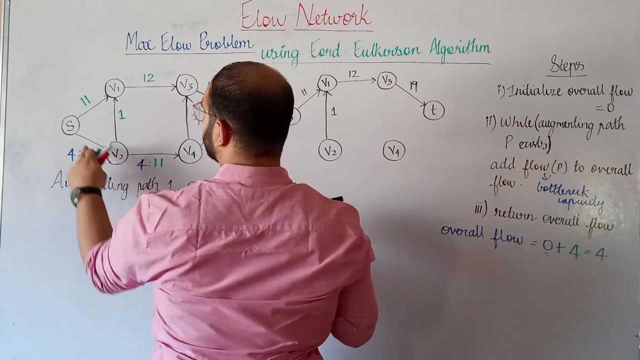 even from b1 to b3, no change. so the residual capacity is 12 from b3 to bt. so again, this was not. this edge was not included in our augmenting path. so it will remain at 1 from s to b2. so basically, the residual 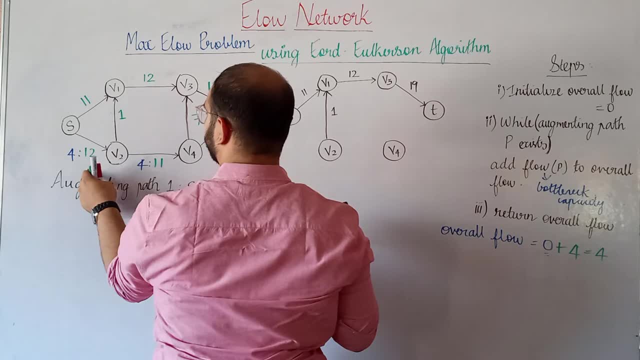 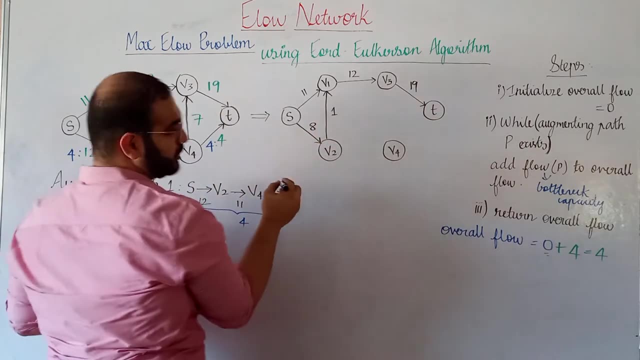 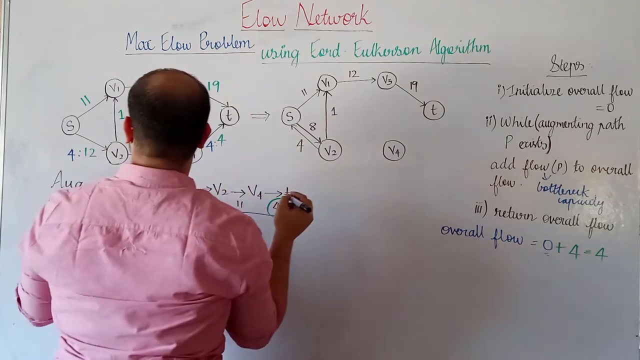 capacity from s to b2 is 12 minus 4 because initially 4 is already flowing. so 12 minus 4 is the residual capacity, that is h. ok, and again we will draw an opposite edge to denote this initial edge from b2 to b4. 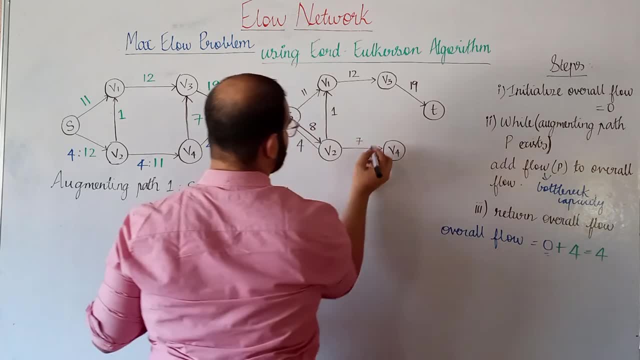 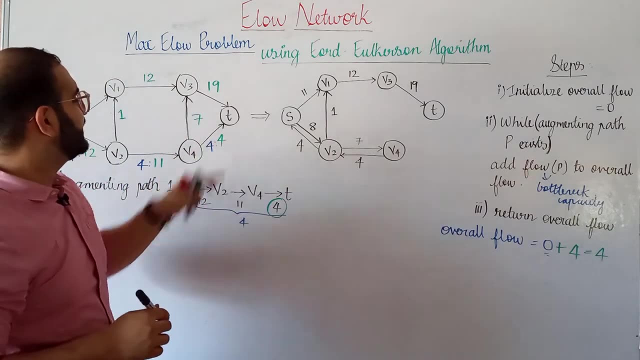 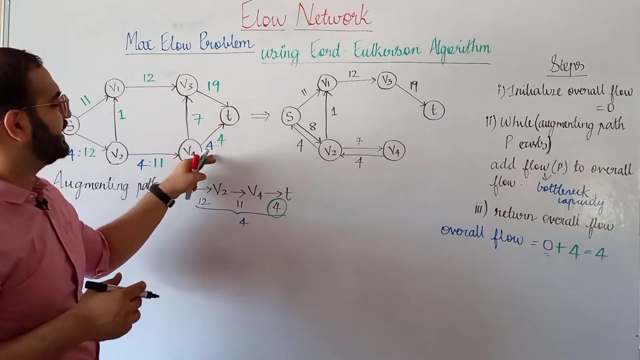 the residual capacity is capacity minus flow, that is 11 minus 4, 7, and in opposite direction we will draw 4, and from b4 to t the residual capacity is 0. right, because now no more extra flow is possible in this direction, because it is flowing. 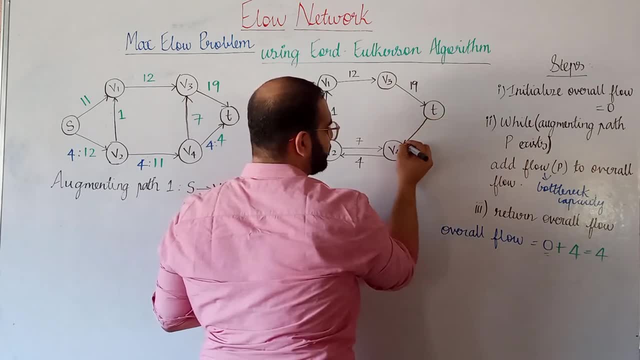 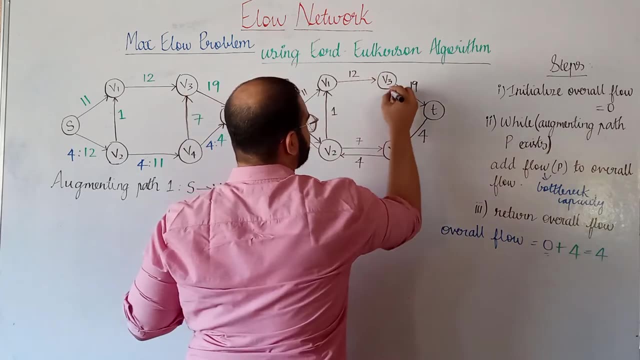 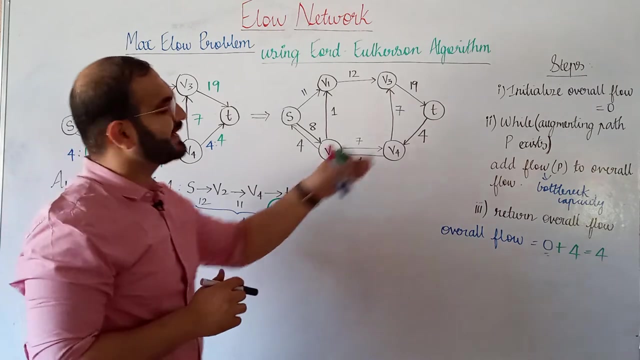 at its capacity of 4 right. so in this very interesting flow, we will draw an edge in the opposite direction with the value of 4, and again in this direction. it will remain same. from b4 to 3, it will be 7. ok, so this is. 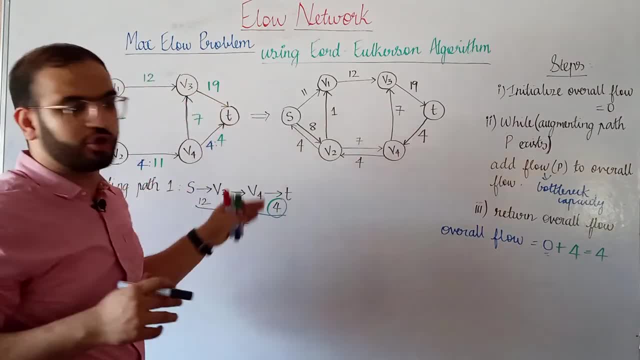 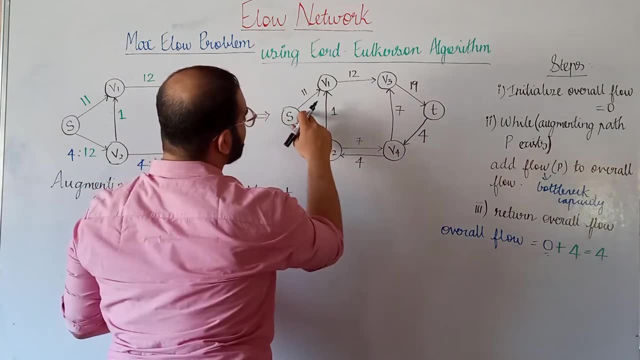 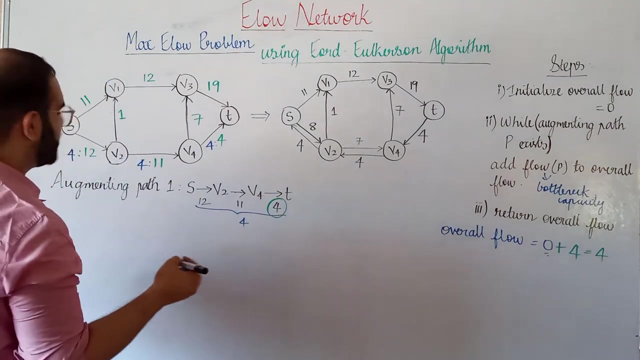 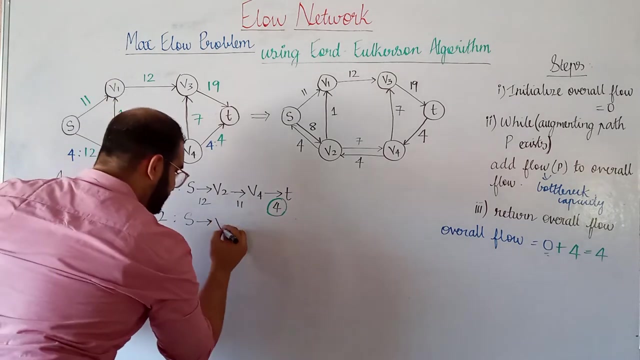 my residual graph. now again, i will check in this new residual graph that if an, i can see a path from s to b1 to b3 to t. yes, so this is another augmenting path that i found out, so let me draw that augmenting path. 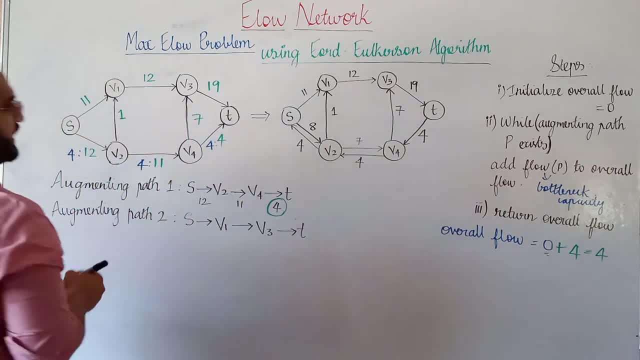 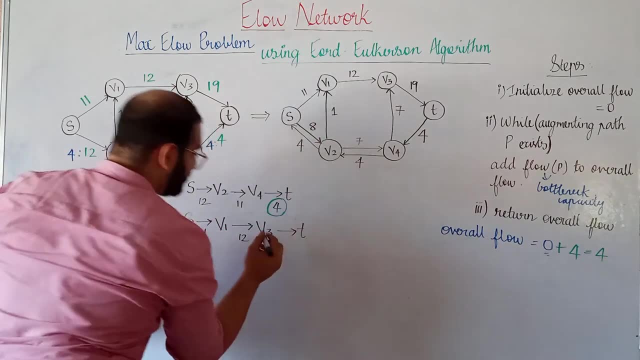 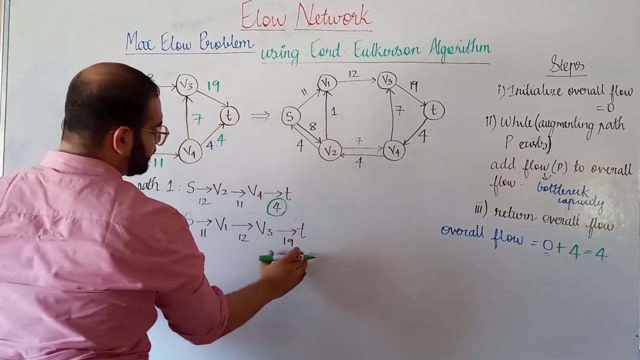 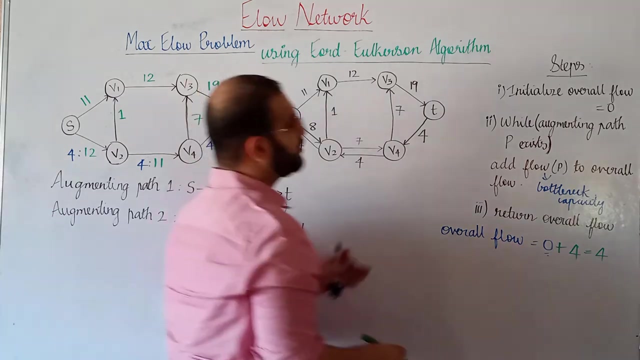 we will call it as augmenting path 2, so it is from s to b1 to b3 to t. ok, and if i write down the residual capacities, so if i talk about the bottleneck capacity or the minimum capacity out of all these residual capacities, it is: 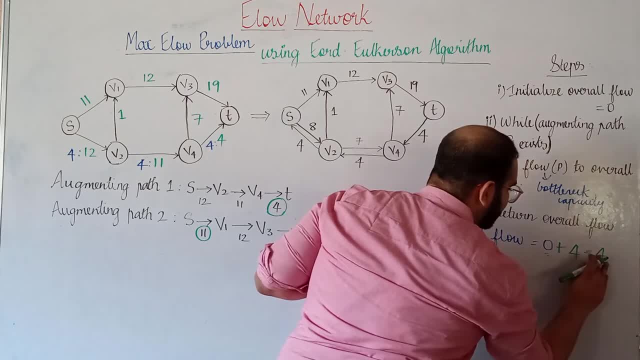 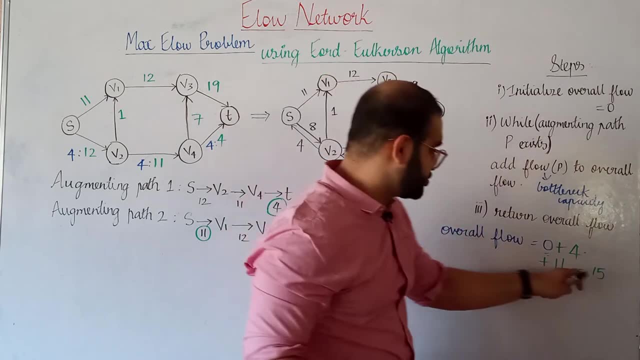 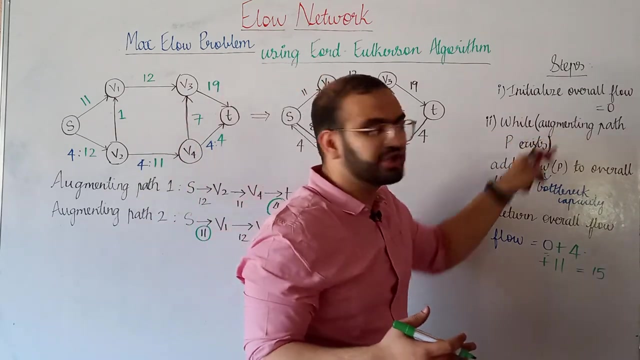 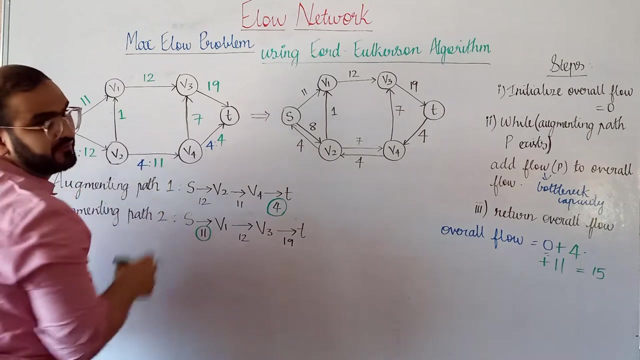 basically 11, right, the minimum is 11. so i will add this bottleneck capacity to my overall flow. so, again, i will add this to my flow. ok, so this particular flow, we need to denote it in our flow network. ok, so let me denote it in my 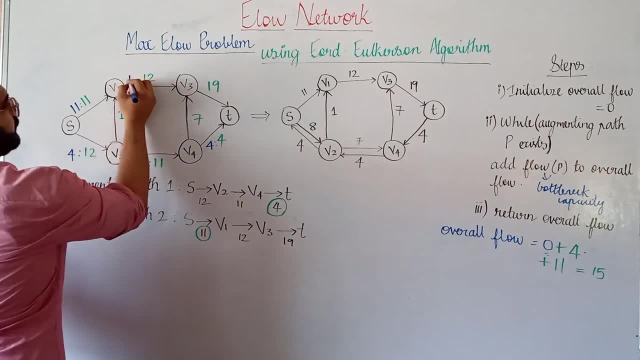 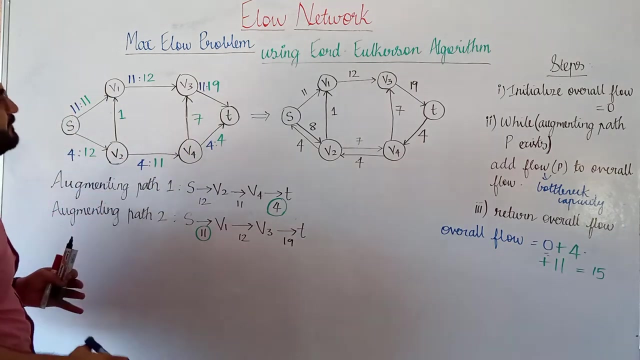 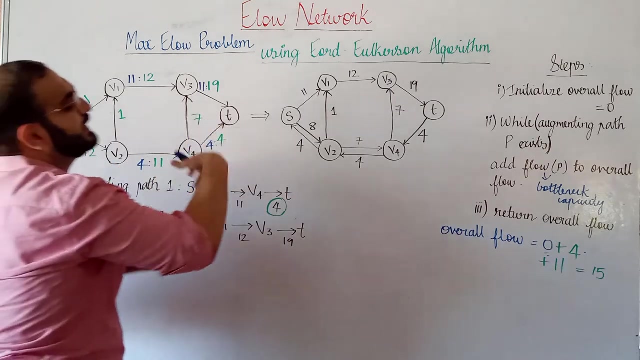 flow network. so initially in this path there was no flow, but now there is a flow of 11 from s to b1 and because of this flow, or because of this new augmenting path, we will have a new residual graph. this is not the residual graph. 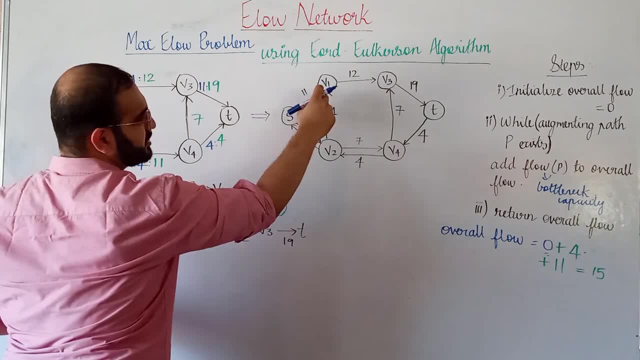 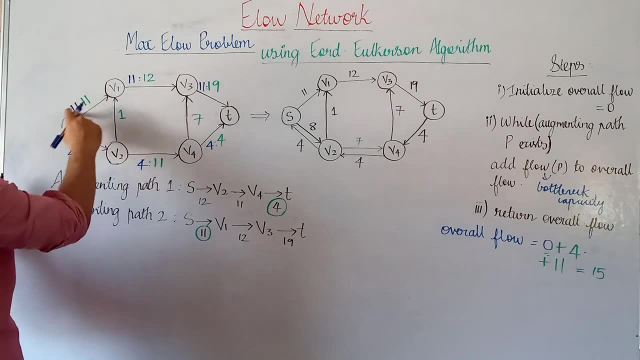 corresponding to this flow network. we will get a new one. right, because even if you see over here from s to b1, the residual capacity will be zero. right, because already a value of level is flowing through this edge and its capacity is also level. so this is not. 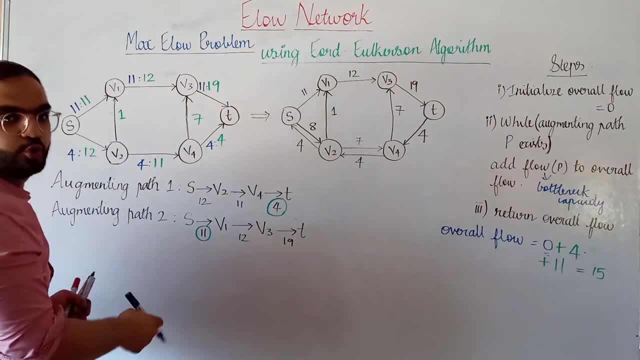 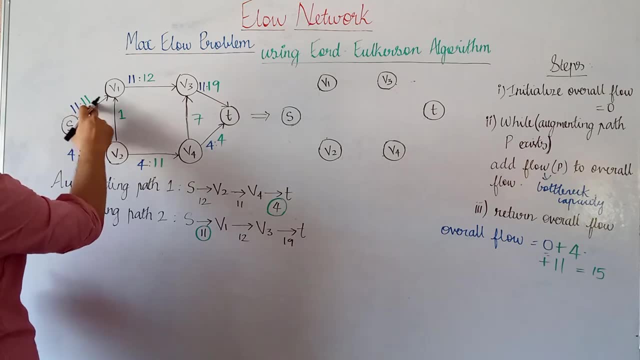 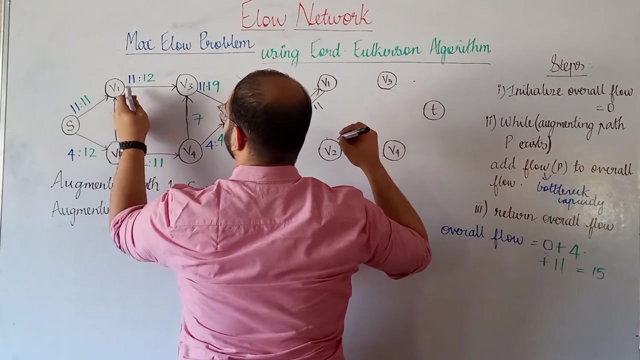 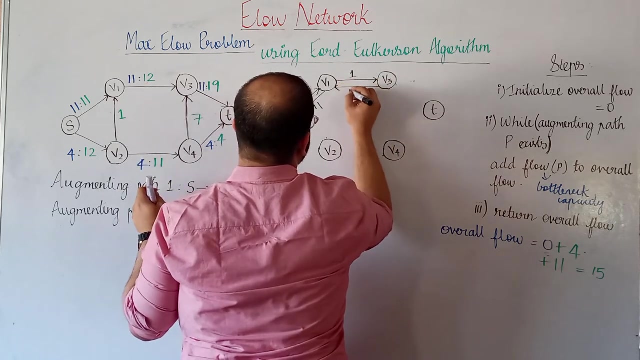 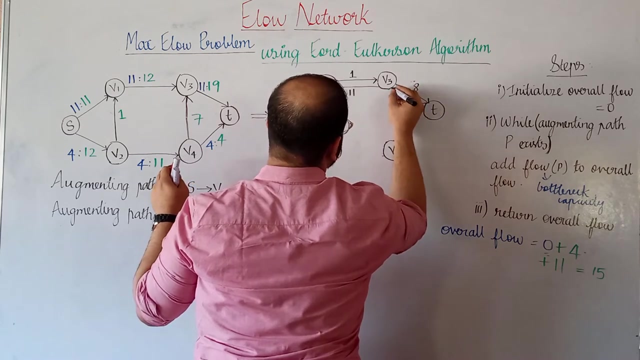 the residual graph corresponding to this flow network. let me draw another residual graph that will correspond to this flow. we will draw an s in the opposite direction. okay, and from b1 to b3, the residual capacity is one that is twelve minus eleven, in the opposite direction. 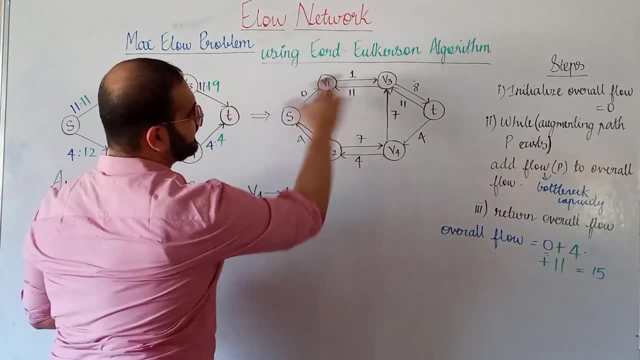 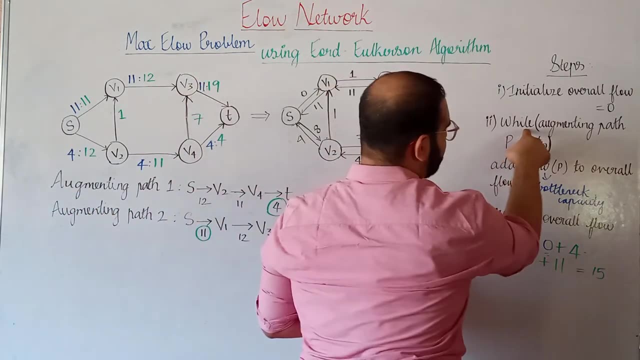 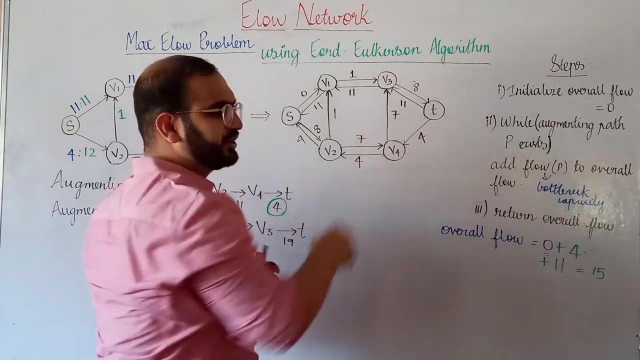 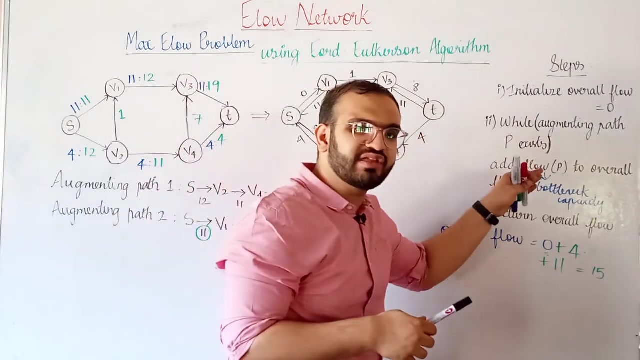 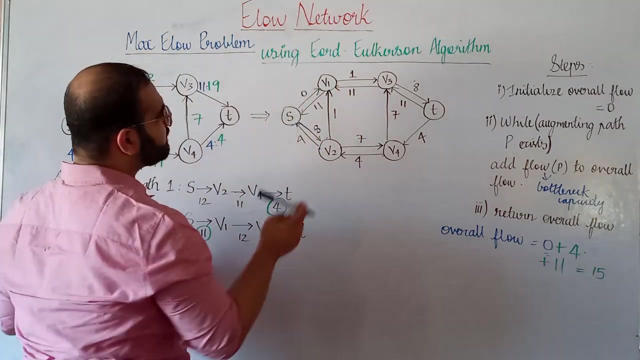 eleven, and the residual capacity from b3 to t is nineteen minus two. so again we are at this step. two, and again we are checking the value condition. if the augmenting path p exists in this new residual graph, then we will add the flow of that augmenting. 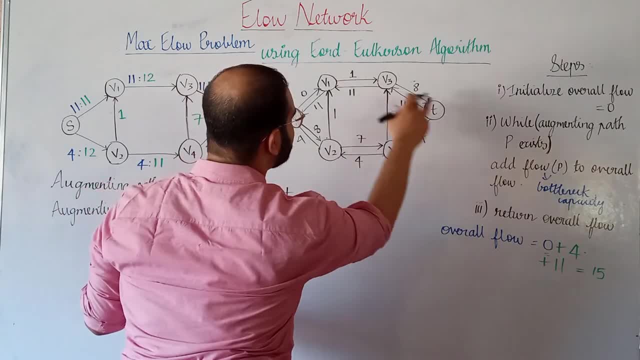 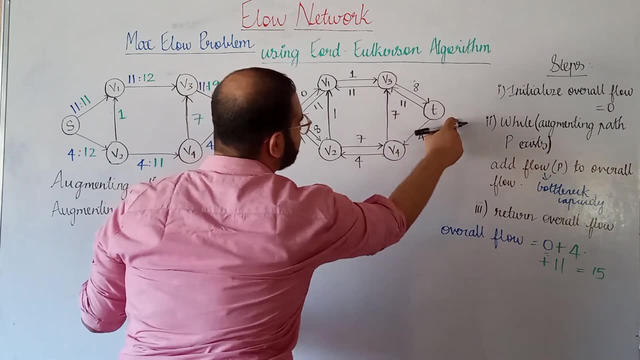 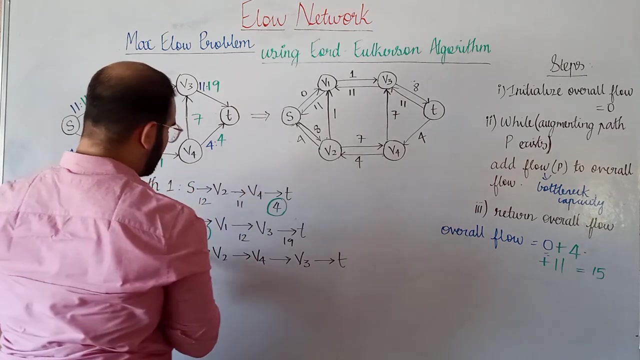 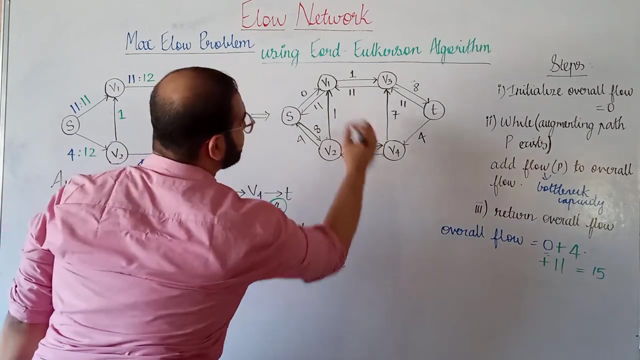 path to our overall path. so yes, there is another augmenting path, from s to b2, b2 to b4, b4 to b3 and b3 to t. so let us write it down as our augmenting path. three and the residual capacities across on all. 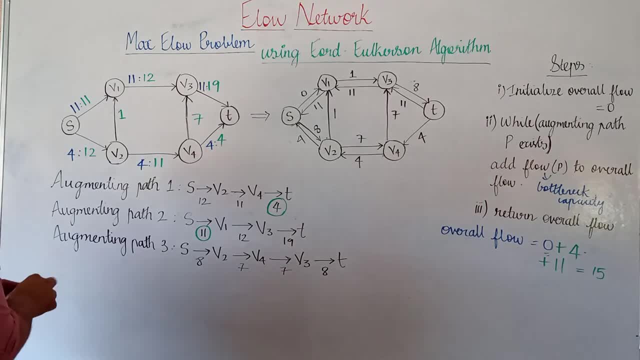 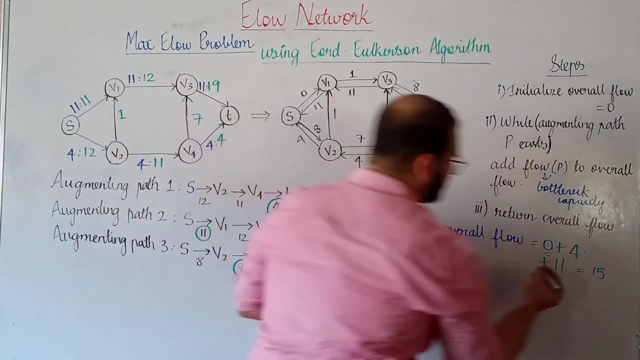 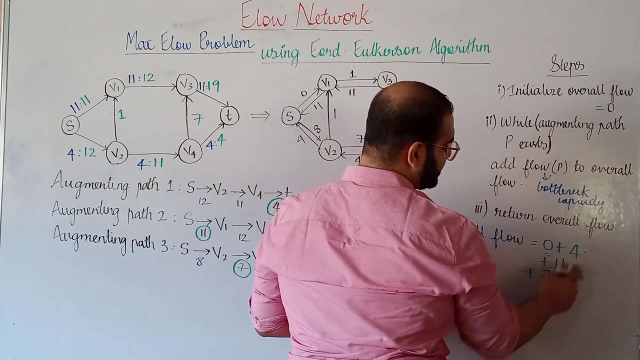 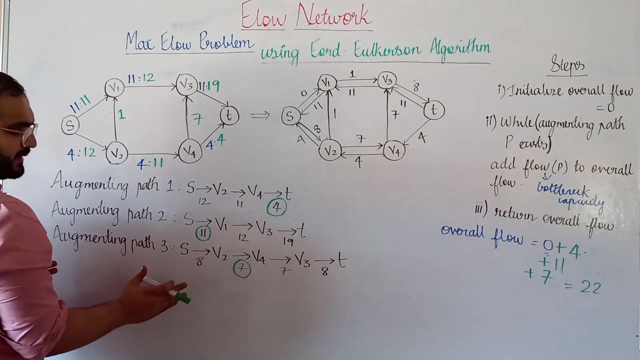 the edges across these paths are: you can call it this seven or this seven, but the value of that is seven, right? so again, there will be an addition in our overall flow and this value will change from fifteen to twenty two. okay, so now we are adding an. 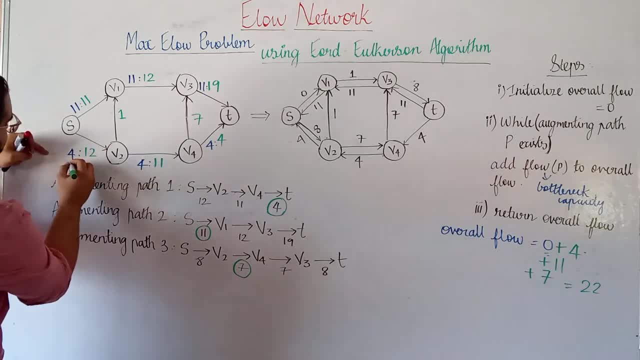 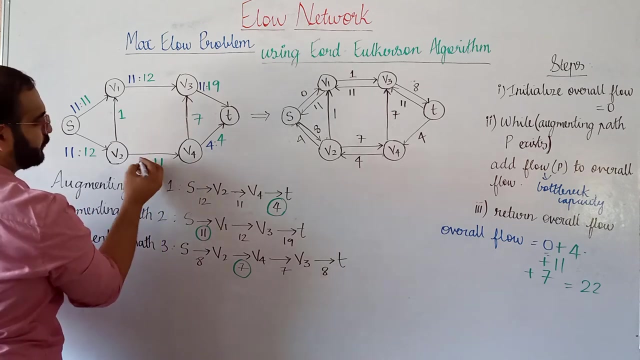 additional flow. so there was already an existing flow from s to b2 of the value four, but we are adding an additional flow of seven. okay, so four plus seven, eleven. okay, even in this case we are adding an additional flow of seven. and from b3 to 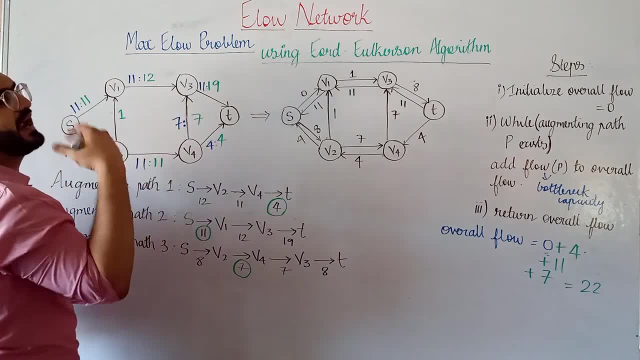 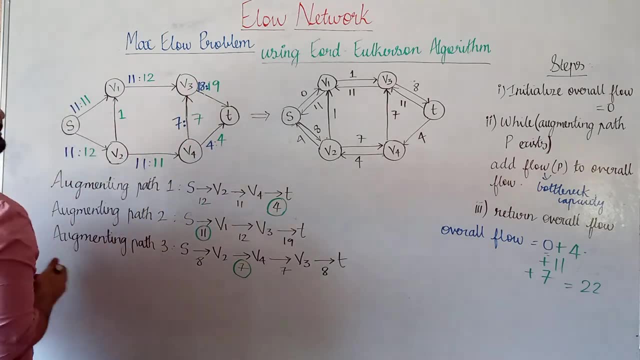 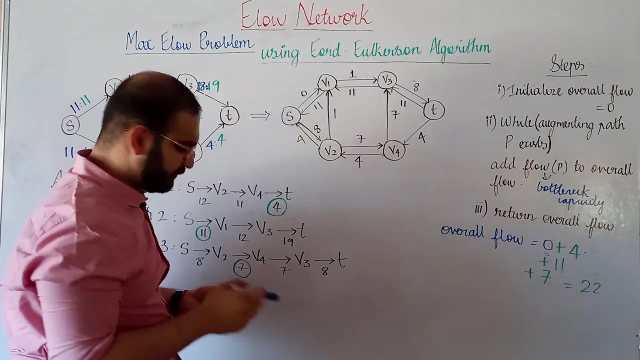 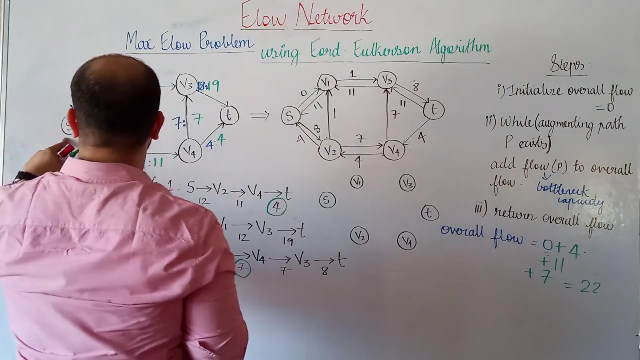 t. initially it was eleven, so again we are adding an additional flow of seven. so eleven plus seven is equal to eighteen. so now we have got this flow network and this residual graph does not have a residual graph over here, over here itself, so we went across this path. 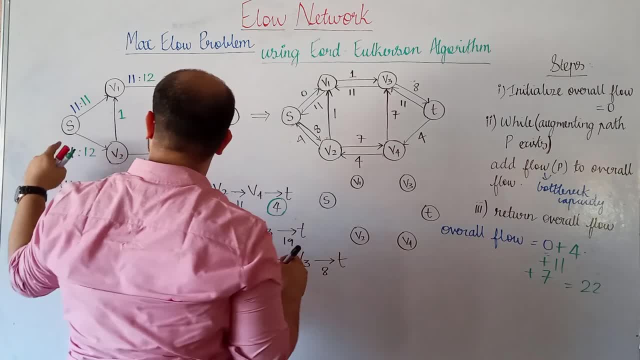 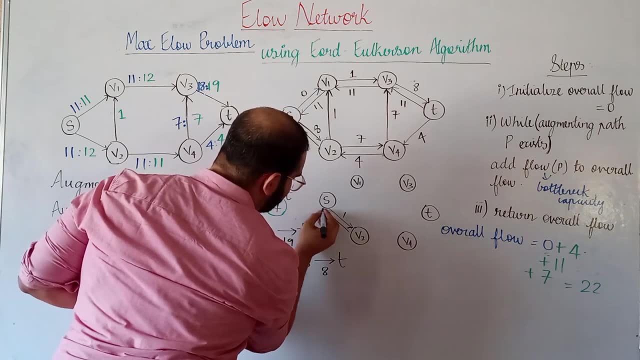 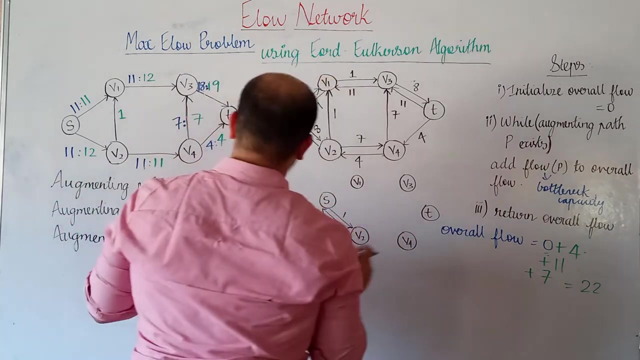 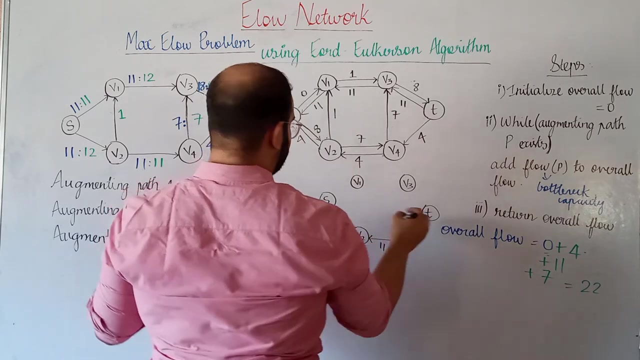 from s to b2. okay, so from s to b2 now we can have. now the residual capacity from s to b2 is twelve minus eleven, that is one, and we will draw an edge. so we will just draw an opposite edge of eleven. then from b4 to 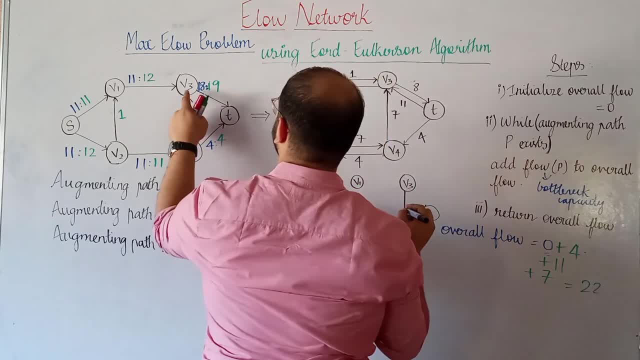 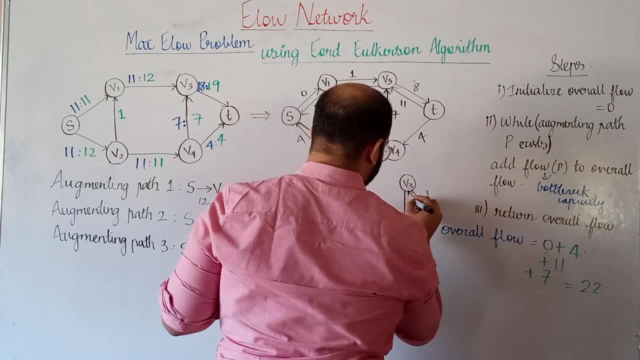 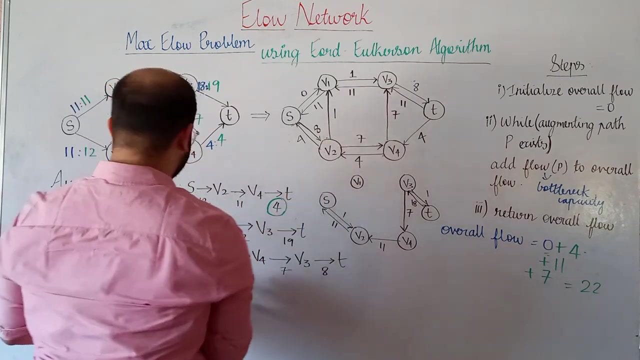 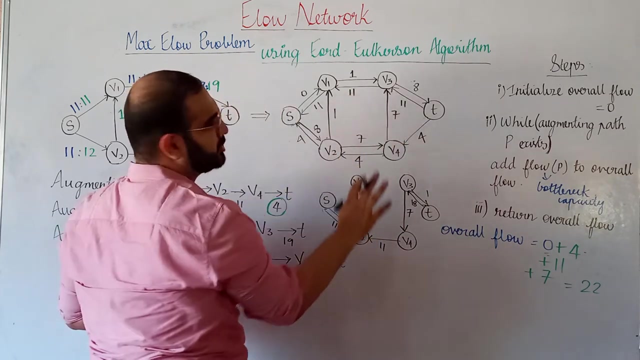 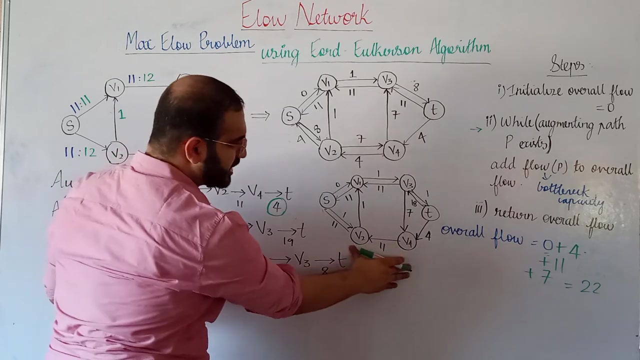 b3, again, the residual capacity is seven minus seven zero. so we draw an opposite edge of seven from b3 to t, the residual path. okay, so the rest of the things will remain same as they were in the earlier residual graph, so I copy that as it. 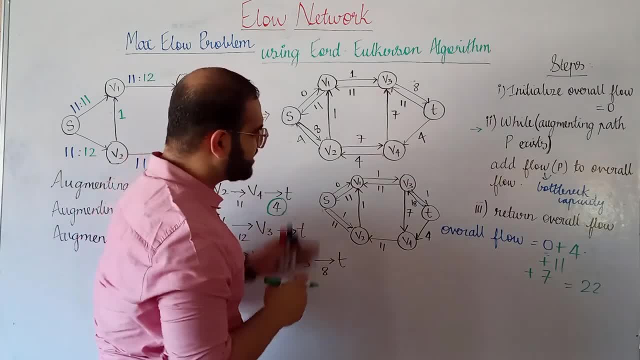 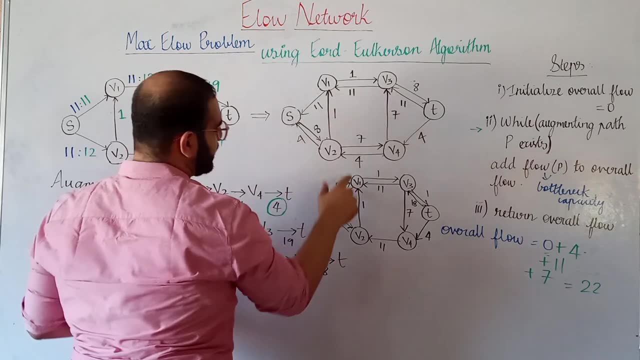 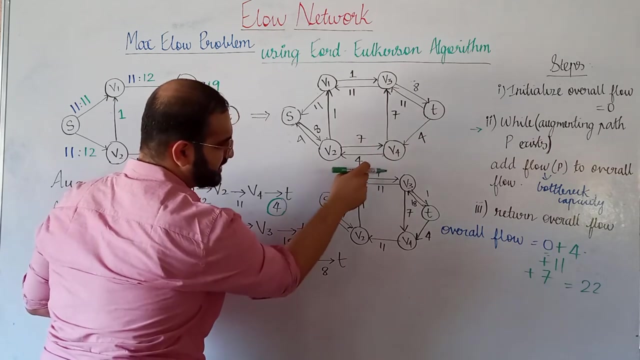 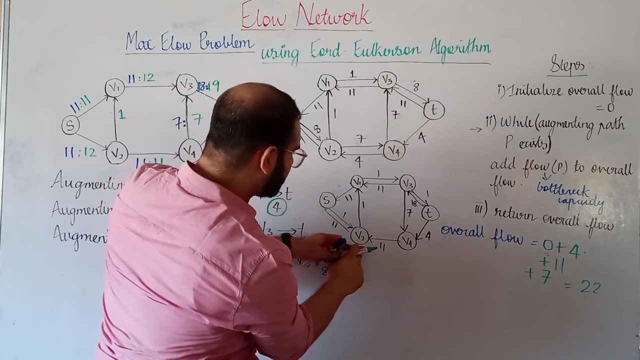 is so now again, I am at my step two and I look at this new residual graph and I check if an augmenting path exists in this residual graph or not. so I will just look at this direction because there is just an incoming edge from v1. 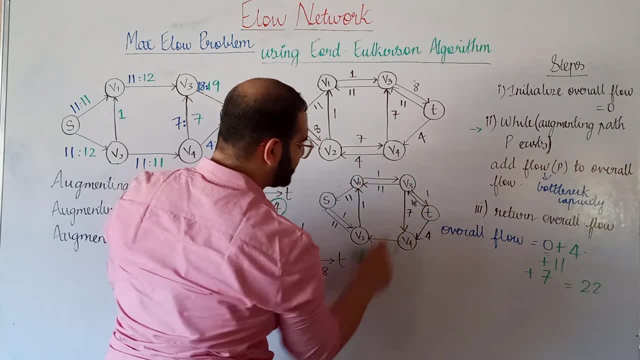 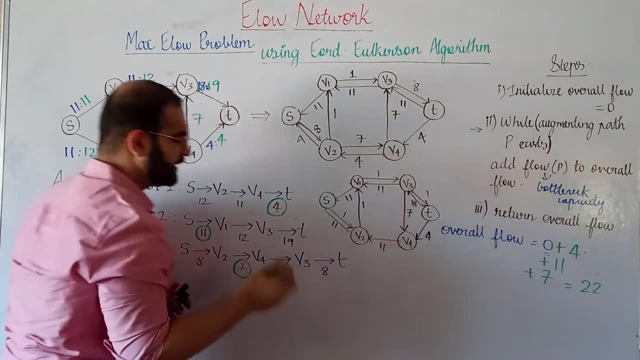 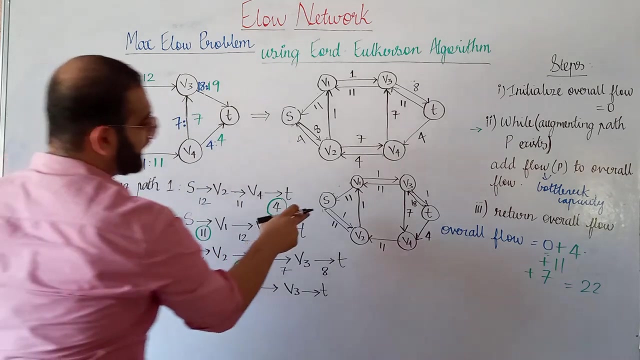 but if you look at this direction, from s to b2, so from v2 we can only go to v1, from v1 to v3, then from v3 to t. yes, we have got an augmenting path from s to v2, v2 to 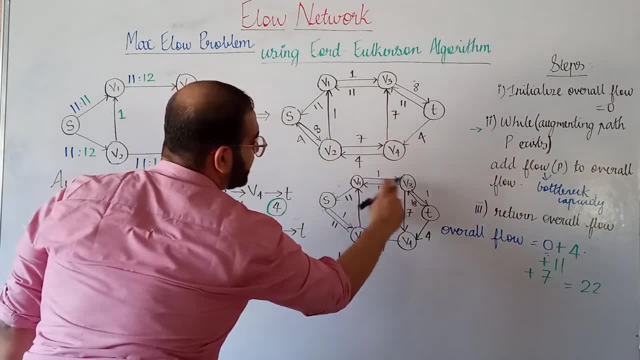 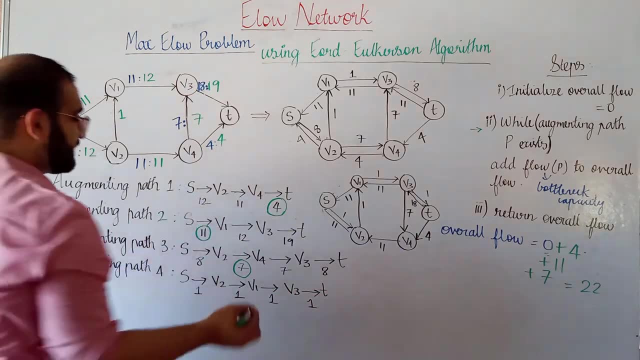 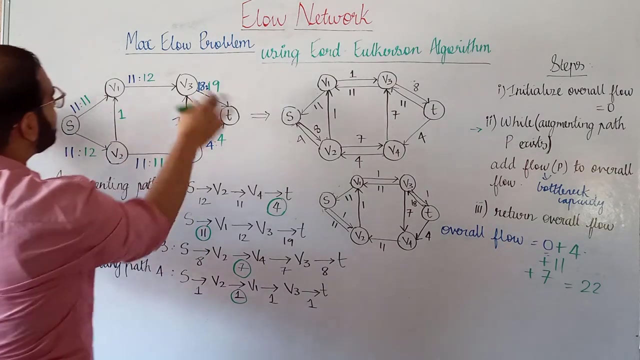 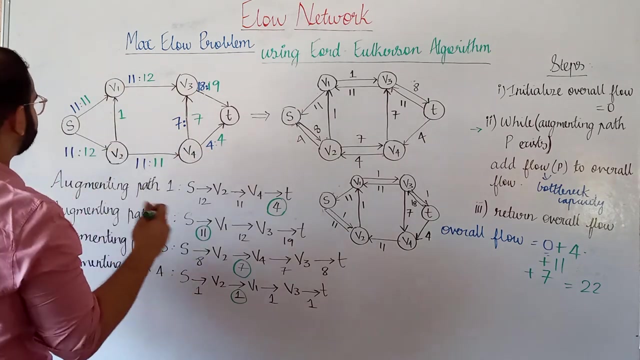 v1. also it is one. v1 to v3, it is one. from v3 to t it is one. so no doubt about it. the bottleneck capacity in this case is one, because the minimum of all of these, of all ones, is one right. so to include. 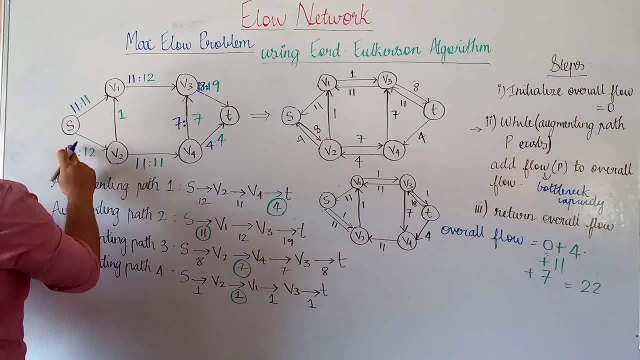 this from 11. there will be an additional one value of bottleneck capacity, so it will change from 11 to 12, from v2 to v1. initially the flow was zero, as you can see over here, so it changes to one. so again from v1. 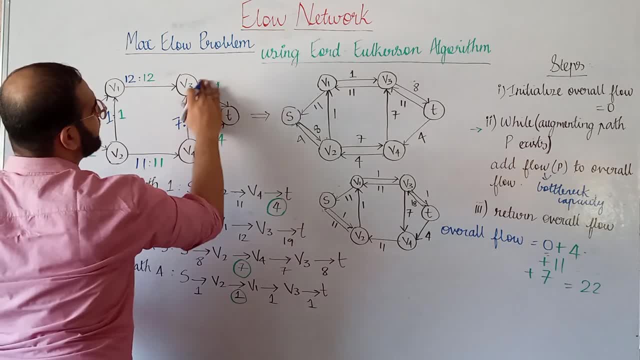 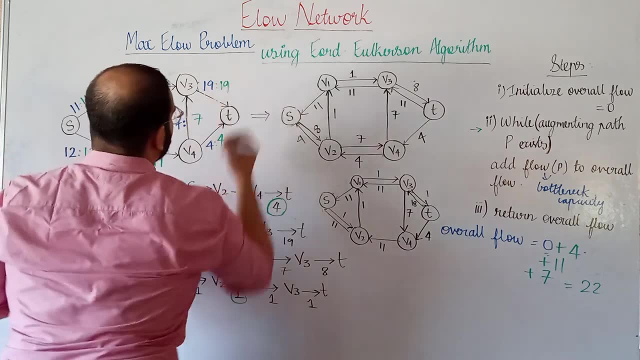 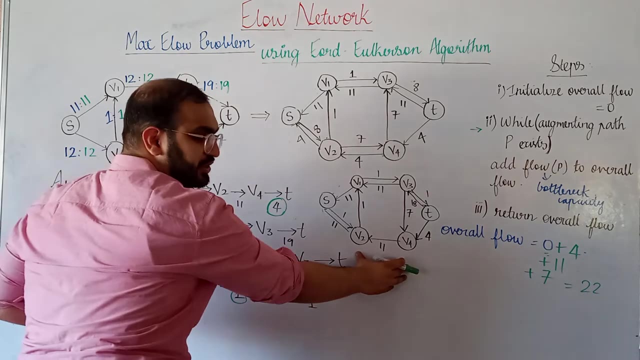 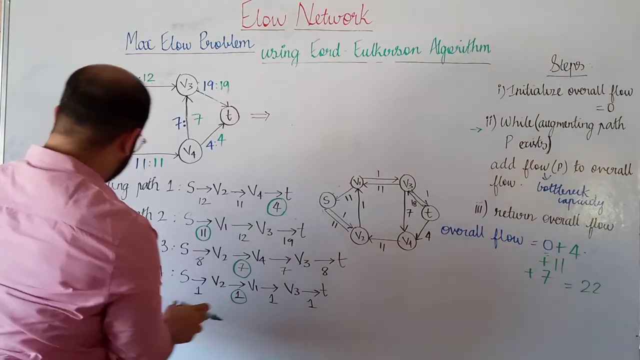 to v3. it was initially 11, so we add the bottleneck capacity to 19 and the capacity was also 19. okay, fine, so this is the new flow network, now corresponding to this flow network. this is not the residual graph, but we need to draw another. 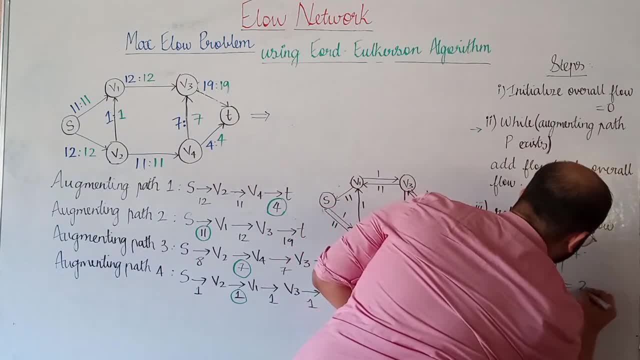 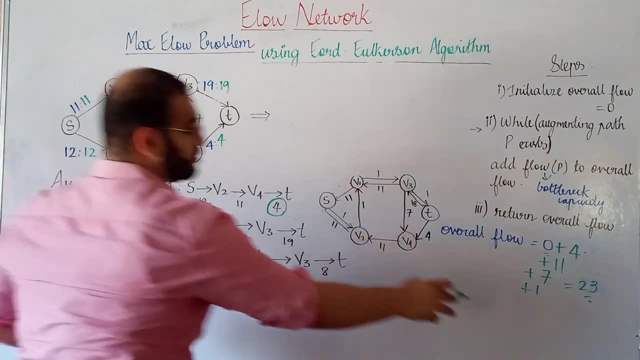 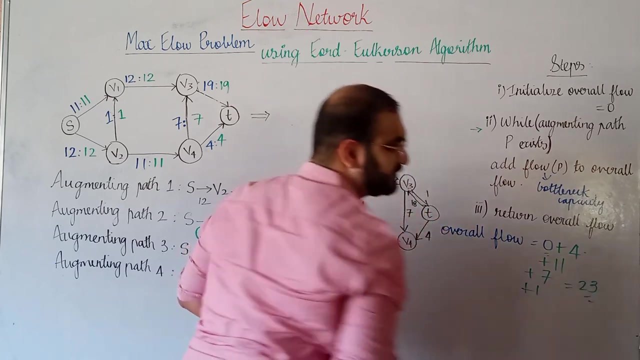 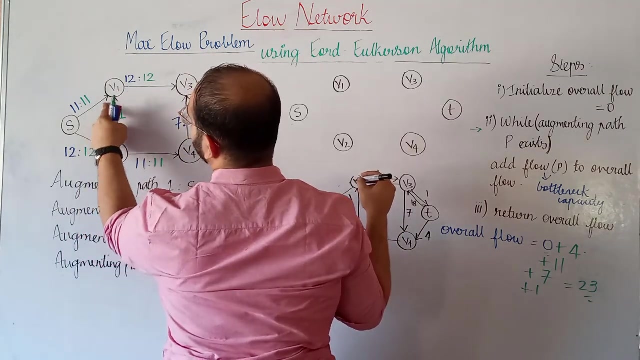 residual graph. so i will remove this old residual graph at the end of this video. so let me draw the residual graph corresponding to this flow network. so for s to v1 there is no residual capacity. so there will be no edge from s to v1, just an. 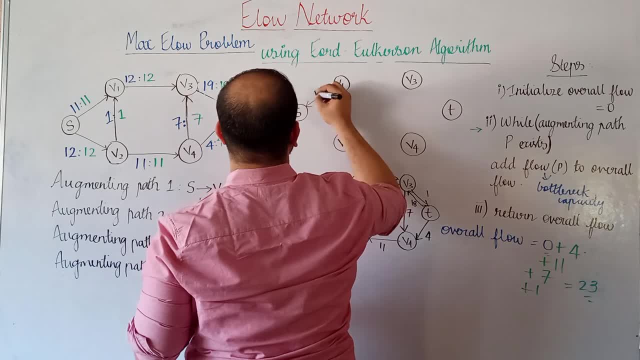 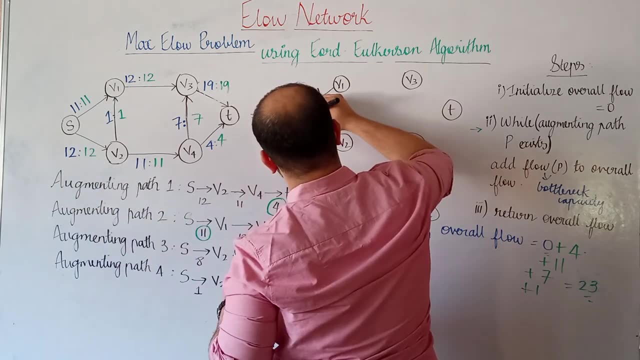 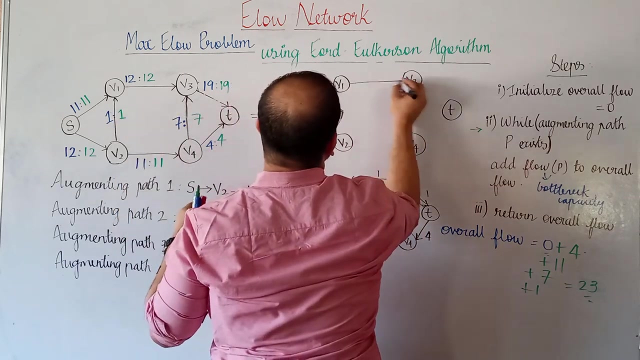 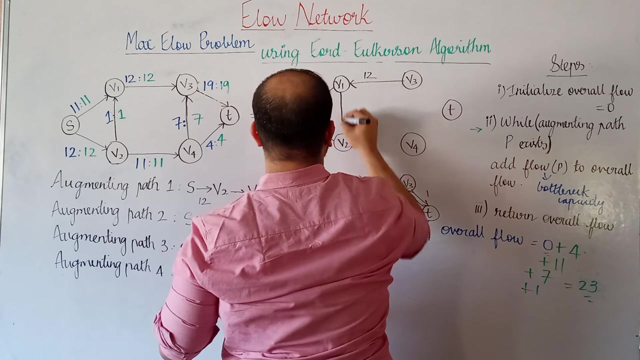 opposite edge of 11 and from s to v2. again, the residual capacity is 0 because 12 minus 12. so there will just be an opposite edge, that is, from v2 to s, and its value will be 12, same in the case of. 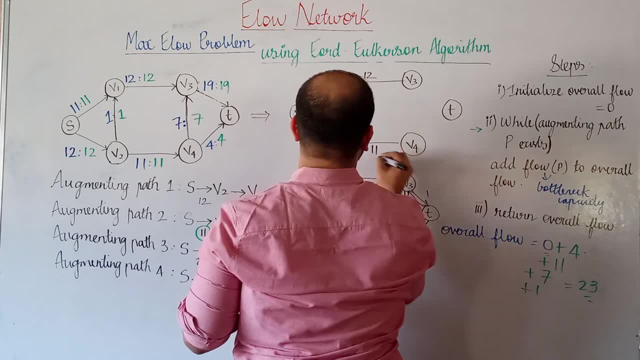 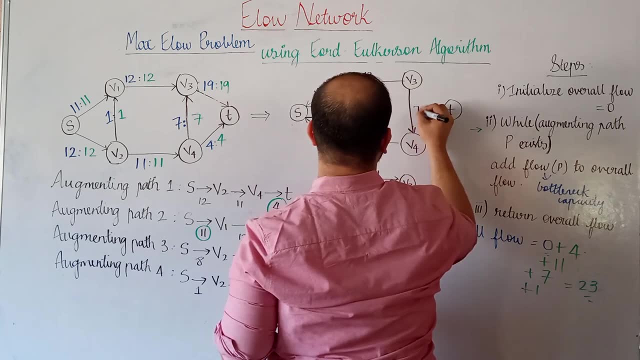 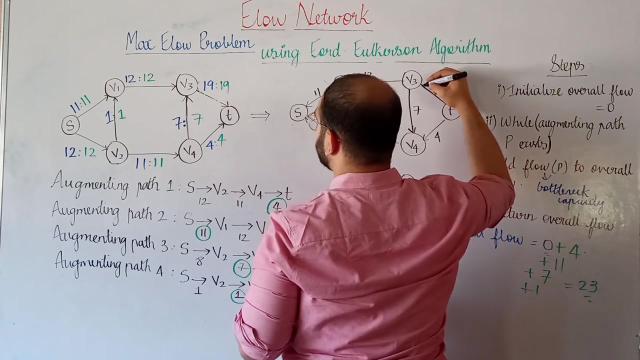 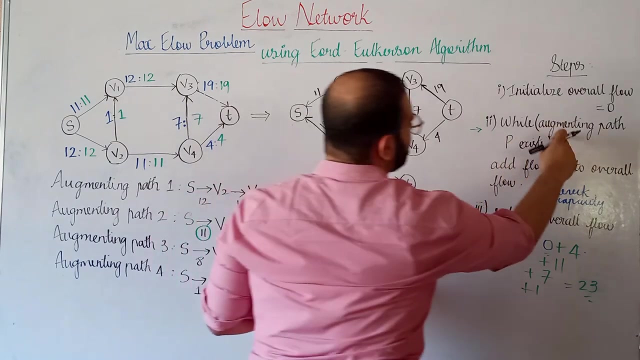 v1 to v3. for v2 to v1, the residual capacity is 1 minus 1: 0, so we will draw it as 7 over here 4. so, as we can see, the residual capacity at each and every edge seems to be 0. 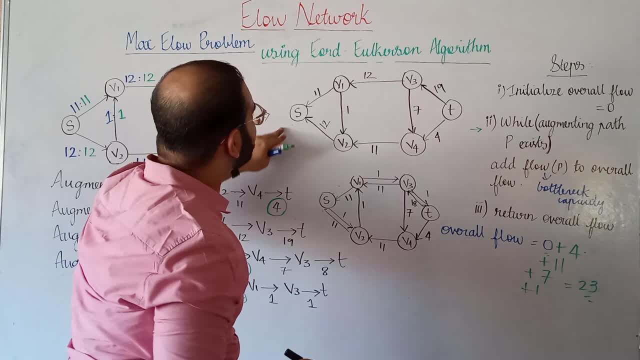 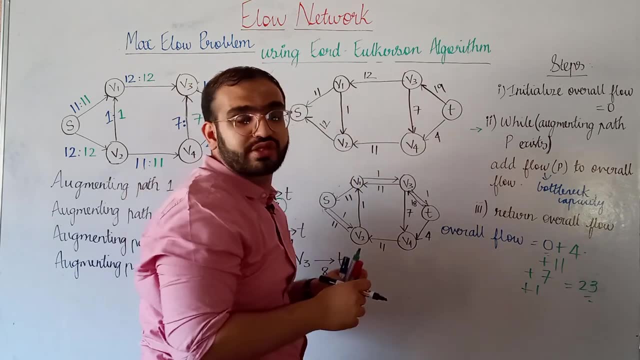 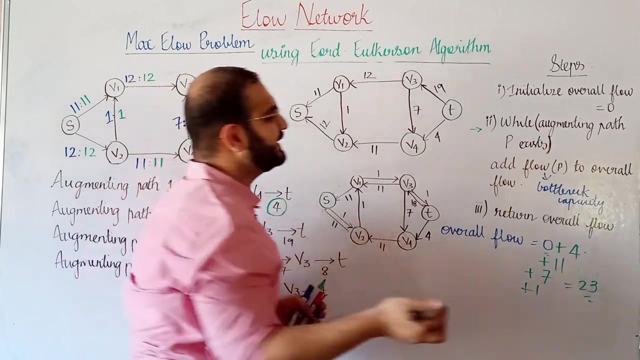 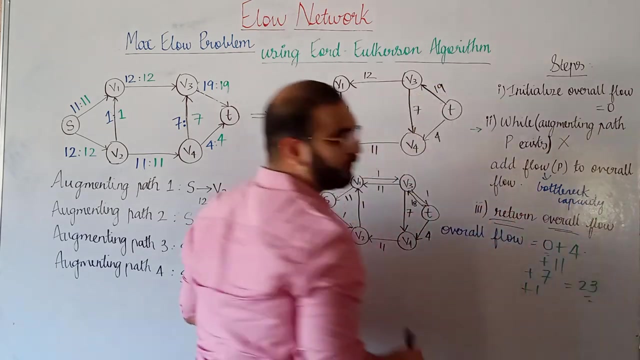 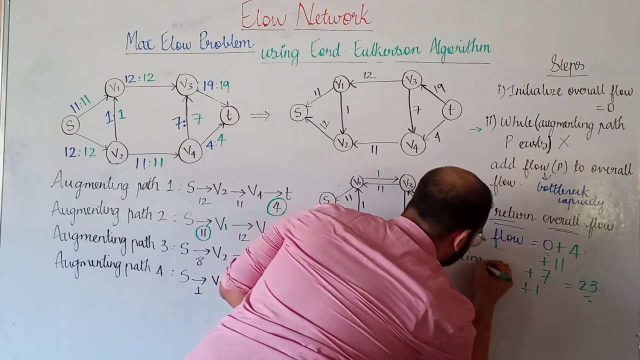 it is 0. so again, let us try to find if an augmenting path p exists in this new residual graph. so if we have a path in this residual graph, so in this case the y condition fails and we go to the third step where we return. 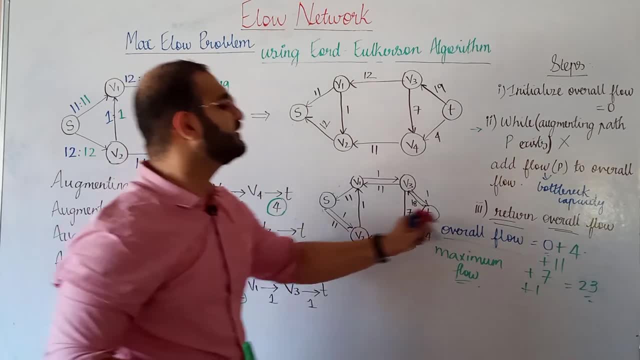 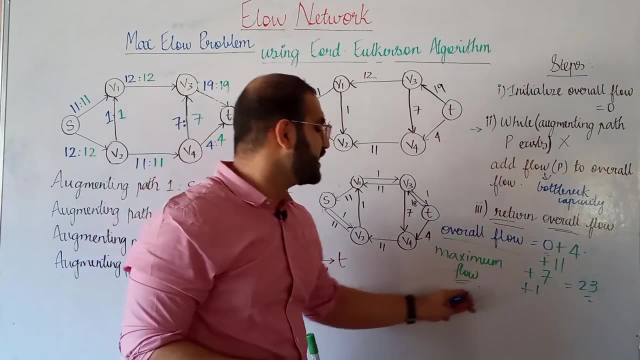 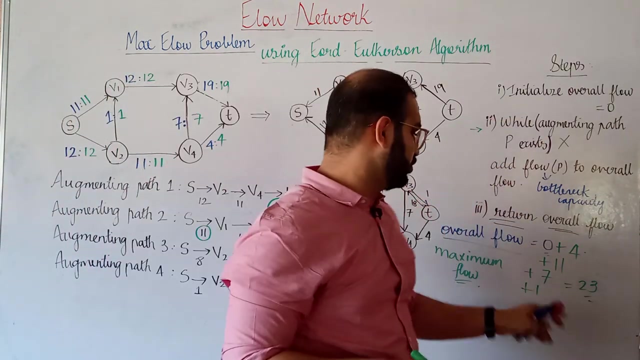 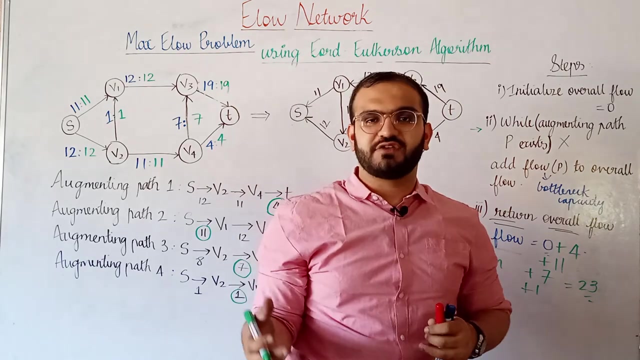 the overall flow, and this overall flow is actually also our maximum flow. ok, so this was our Schwarz-Pulkerson algorithm, in which we initialized our overall flow in the initial step with 0, and then we check for each and every new residual graph that we got. that. 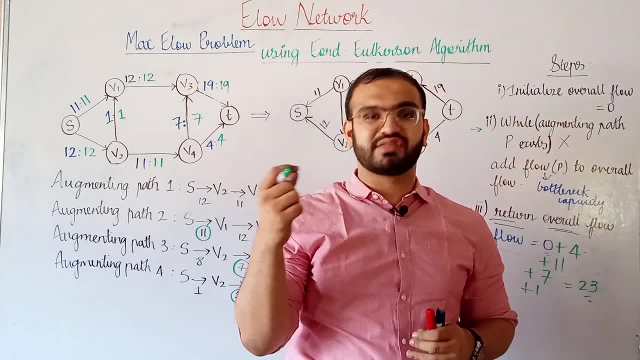 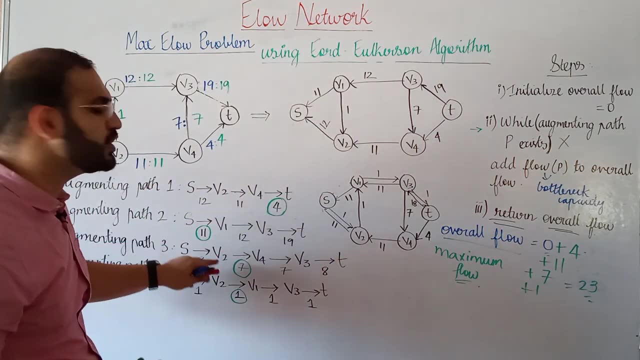 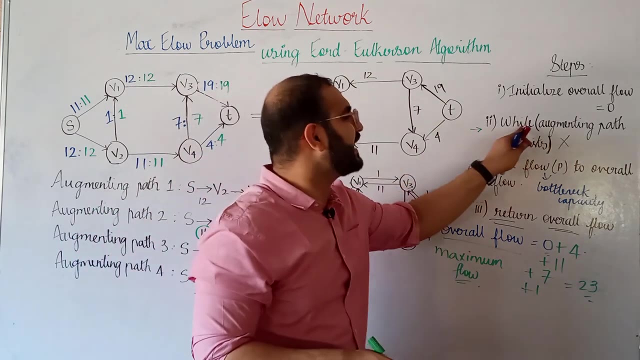 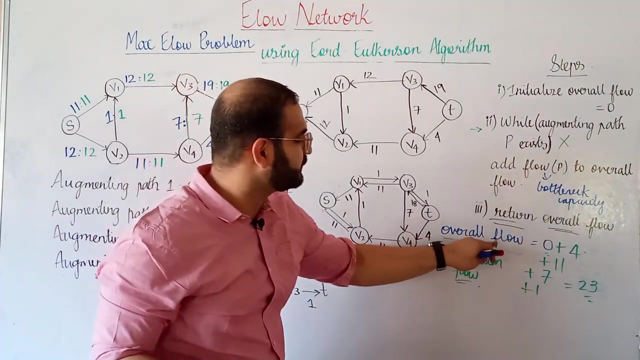 is there an augmenting path existing in that residual graph? if an augmenting path is existing in the residual graph, then we changed each and every of those augmenting paths and we added them to the overall flow, right and when this y condition failed at that time. 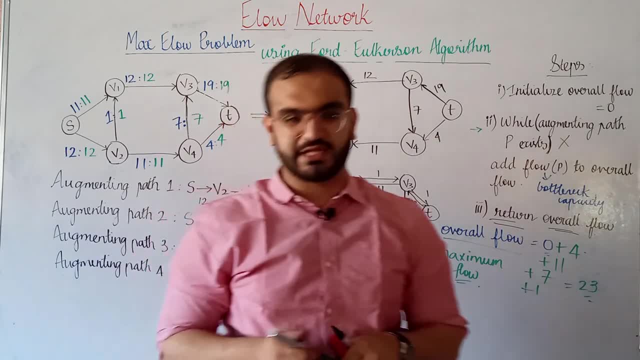 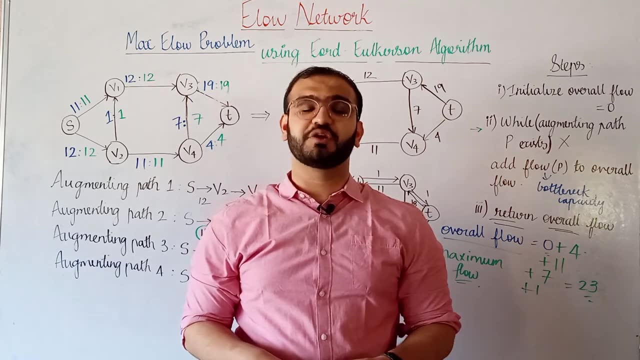 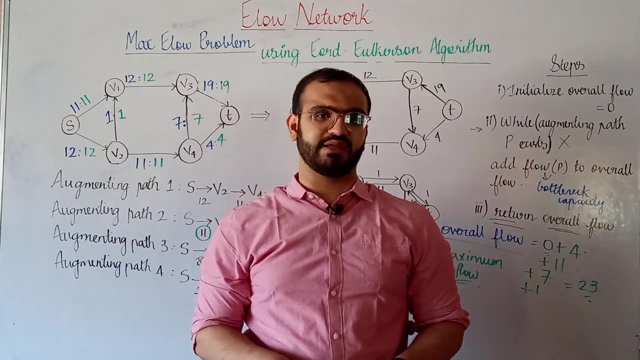 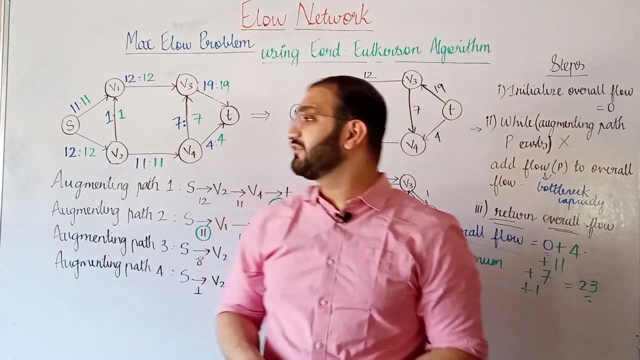 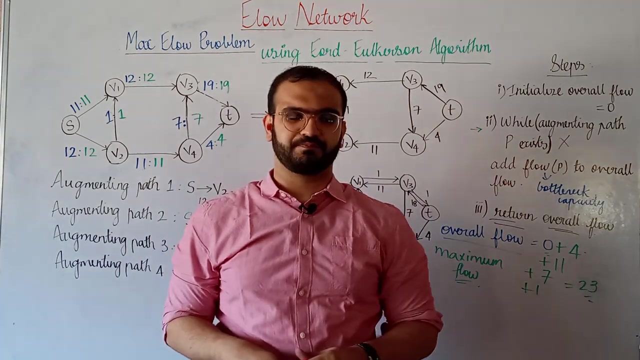 we returned this overall flow. and guess what this overall flow is? we found the different properties of flow, and then we saw what is the residual graph, what are augmenting paths and what is the bottleneck capacity. and then we saw the aim of our maximum flow problem, and then 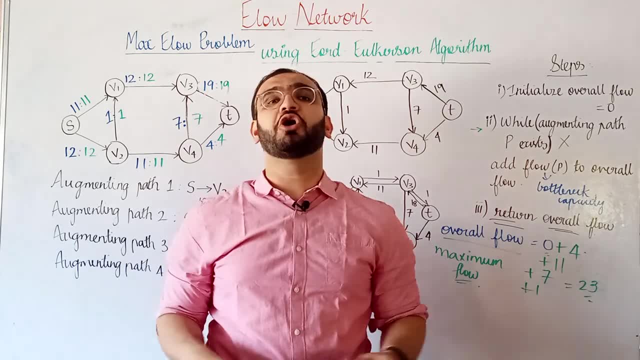 we looked at the Ford-Pulkerson algorithm and finally we came to the conclusion that this is the original flow that we had in the original flow and this is the original flow, and this is the original flow and this.